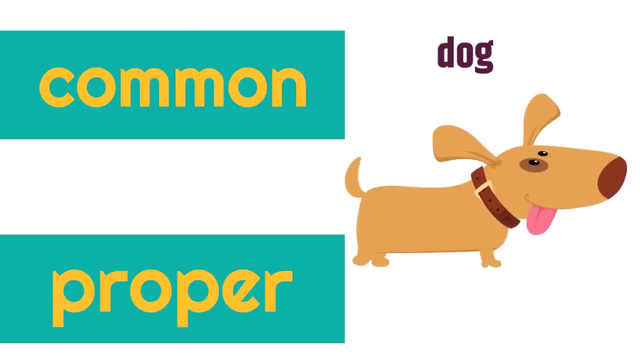 Now, let's say this dog's name is Fido. Fido is the proper noun for this dog, Because that's the specific name of this dog is Fido. Dog is the type of thing that this is, So it's the common noun. The common noun is dog. 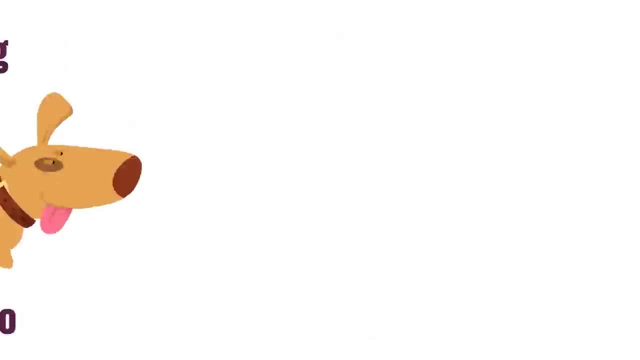 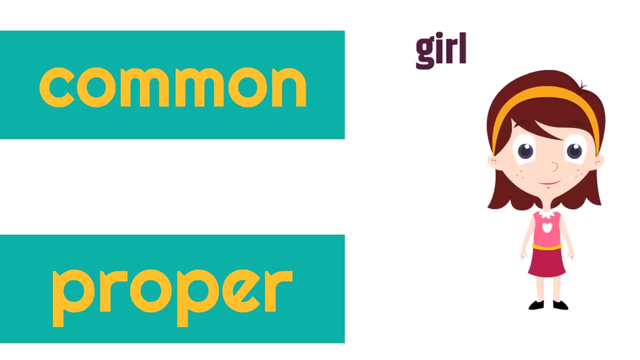 The proper noun for this is Fido. Here's another example. Here is a girl, A girl, And girl would be the common noun, because a common noun is a type of person, place or thing, And girl would be the common noun, because a common noun is a type of person, place or thing. 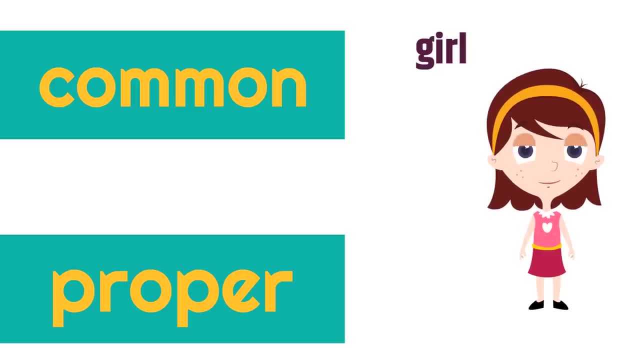 And girl would be the common noun, because a common noun is a type of person, place or thing. But this girl's name is Rachel. Rachel would be the proper noun because it's a specific person, place or thing. So the common noun is girl. 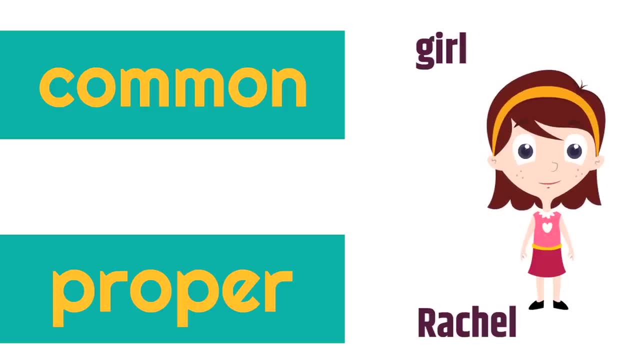 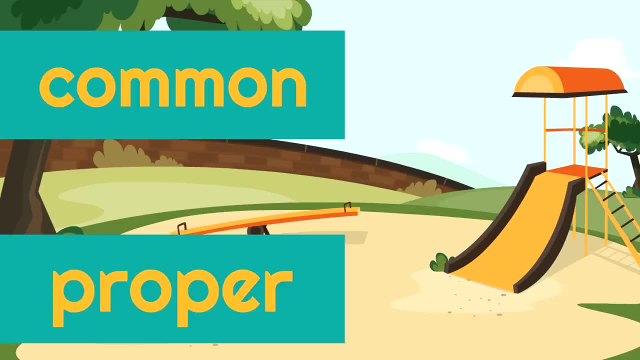 The proper noun is Rachel. Here is another one. Here we have a picture of a park. Park would be the common noun. It's the type of person, place or thing. Now let's say this park is called Smithfield Park. 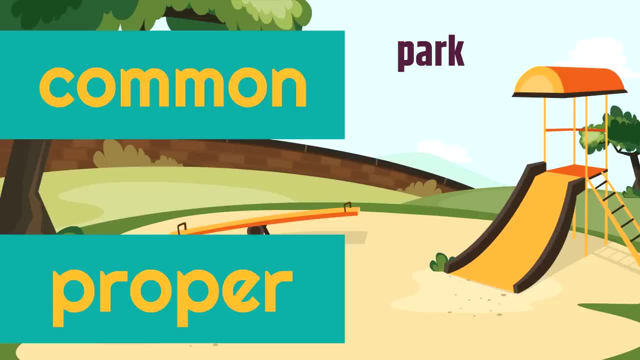 Smithfield Park would be the proper noun. It is the specific person, place or thing that this is. It is a park. that's the common noun and the proper noun is Smithfield Park. Remember common nouns. name a type of person, place or thing. 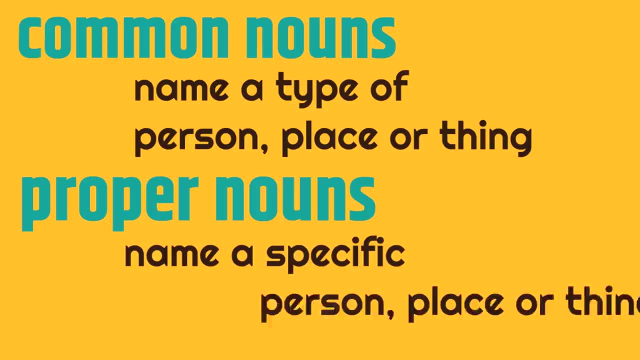 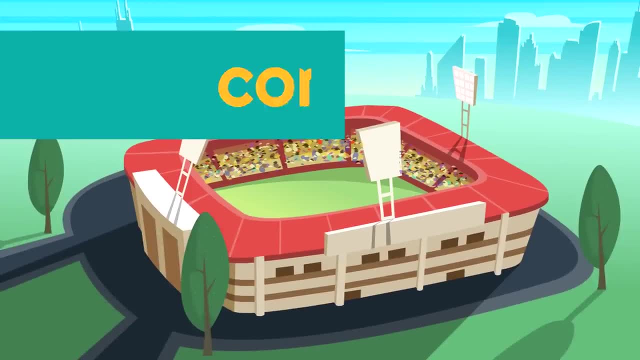 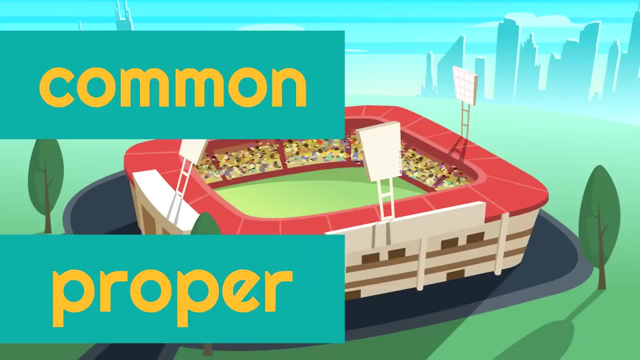 Proper nouns name a specific person, place or thing. Let's look at this example. This is called a stadium. The common noun for this is stadium. But let's say the specific name of this stadium is York Stadium. York Stadium would be the proper noun, It's the specific. 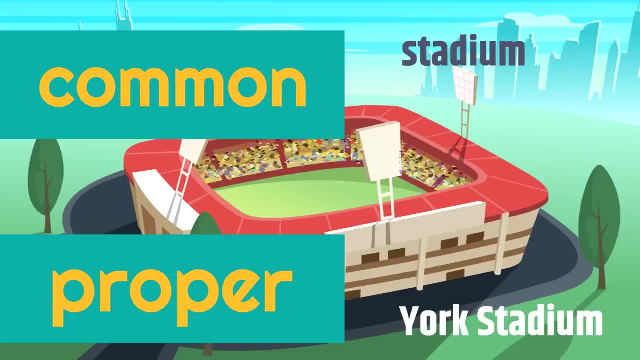 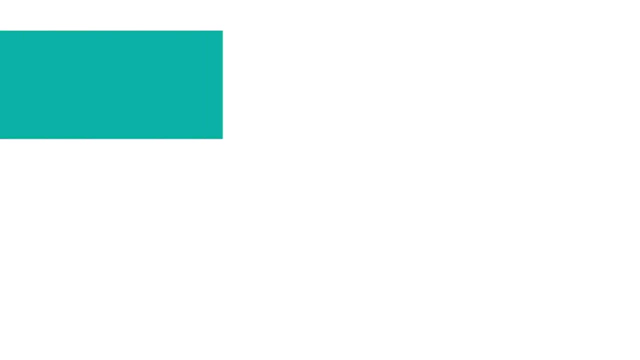 person, place or thing. The common noun is stadium. It's the type of thing that this is. York stadium is the proper noun because it's the specific thing that this is. Let's try this one. What is this? What would be? 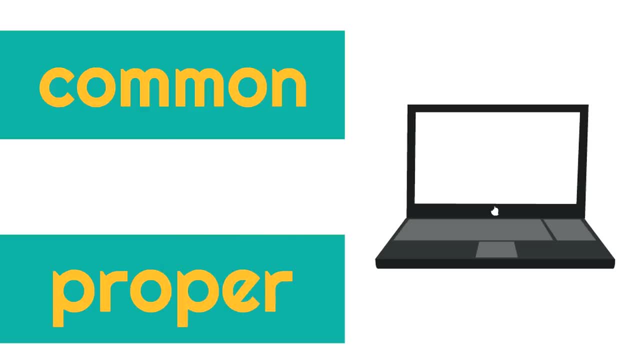 the common noun. Yeah, computer, Computer would be the common noun. computer is a platinum 10. that means that the proper noun for this would be platinum 10. the common noun is the type of person, place or thing which is a computer, and the proper noun is the specific one, which is the platinum 10. 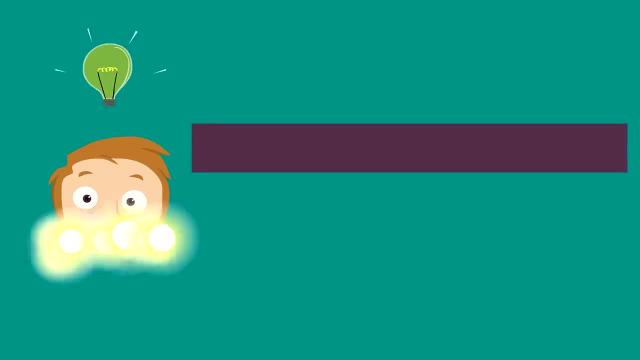 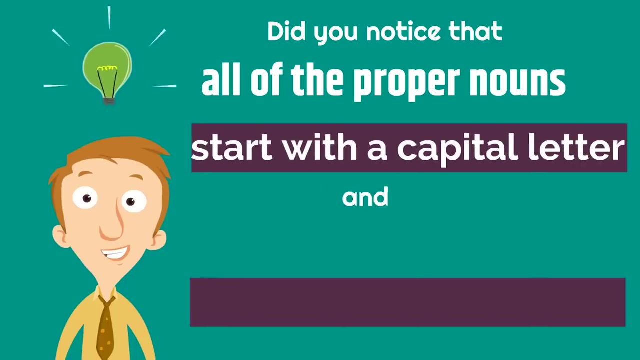 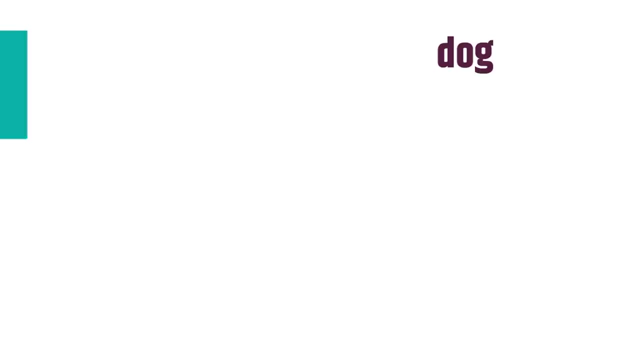 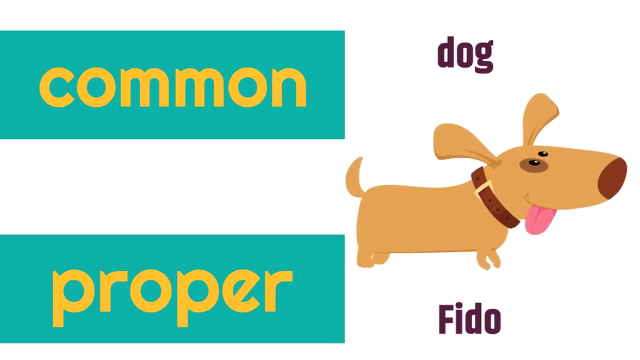 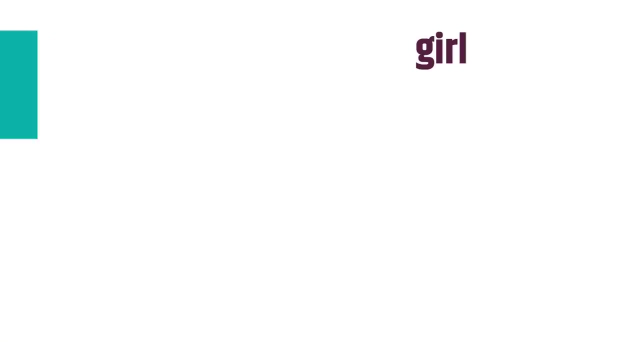 now did you notice that all of the proper nouns start with a capital letter and all of the common nouns start with a lowercase letter? isn't that interesting? let's look back. okay. so dog is common and it's lowercase, and Fido is the proper noun and it's uppercase- it's a capital letter, let's see. and girl is the. 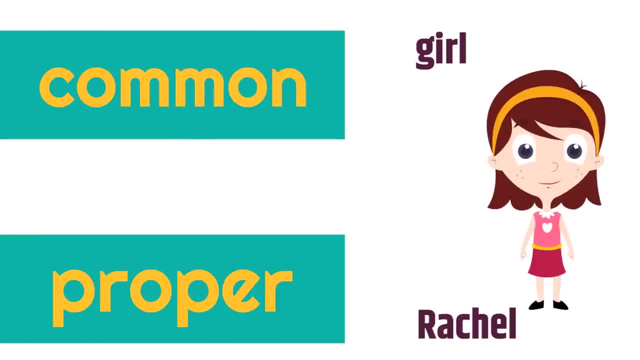 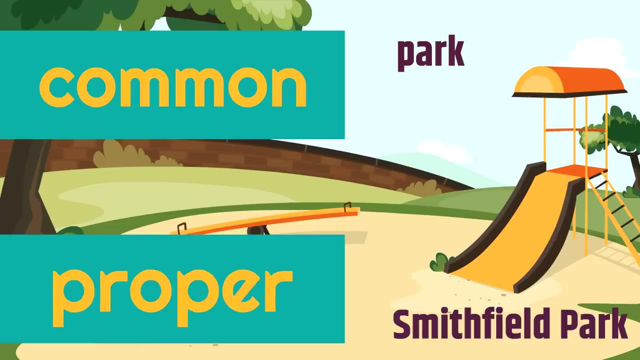 common noun here and Rachel's the proper noun, and Rachel starts with a capital letter. proper nouns always start with a capital letter. oh, wow, and. and. Park is the common today, and it starts with a lowercase letter. and Smithfield Park is the proper now, and so, because it's a proper now, it starts with: 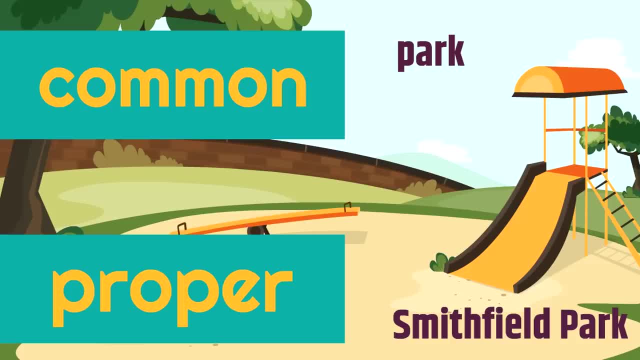 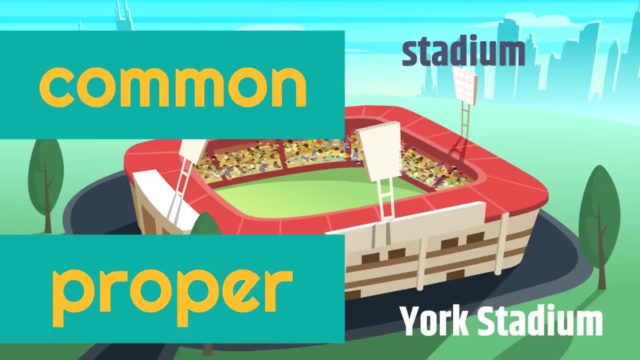 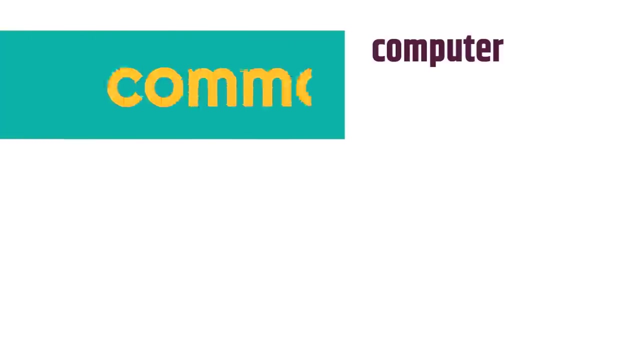 letters. and let's get this one to the common. now. here is to you been the proper now is York Stadium. in the proper noun it starts with capital letters: York Stadium. they are capitalized because it's a proper noun. and what about this one again, okay, the common noun is computer, so has a lowercase letter, but the proper. 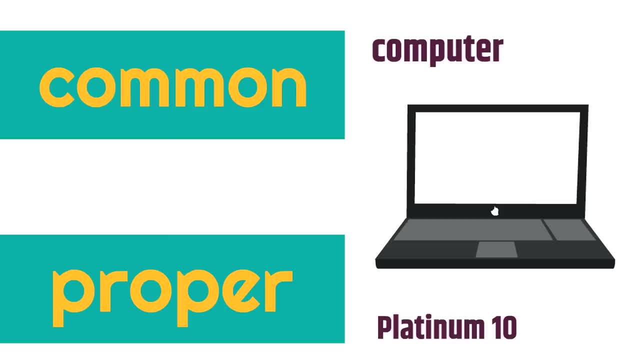 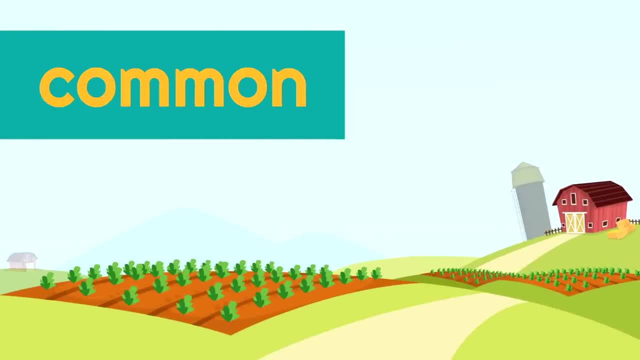 noun is platinum 10, which is capitalized because it's the proper noun. let's look at two more examples. okay, this is a picture of a what yeah, farm is the common noun and notice it's got a lowercase letter. it's the common noun, it's the type of thing that this is now. the name of the farm is Johnsonburg. 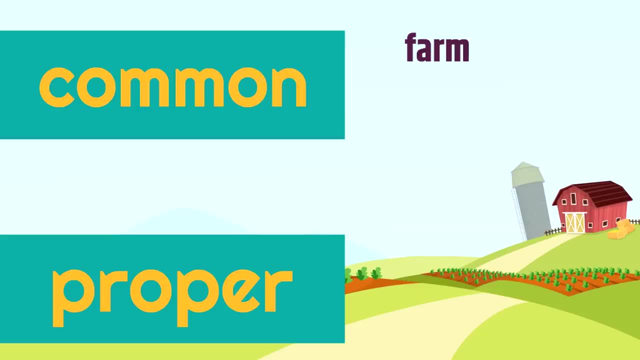 Ranch. so that's the proper noun, it's the specific farm, that it is Johnsonburg Ranch, and notice how it's capitalized, because it's a proper noun. Johnsonburg Ranch is the proper noun and it's capitalized. it's the specific thing, that it is okay. now this is our. 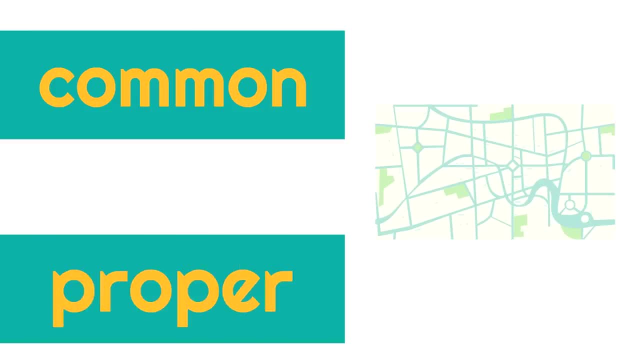 final one. the common noun of this is a map of a city. city would be the common noun. and notice the lowercase letter. it's the type of person, place or thing. it's got a little letter. it's the common noun. now let's say this city is Denver. Denver would be the 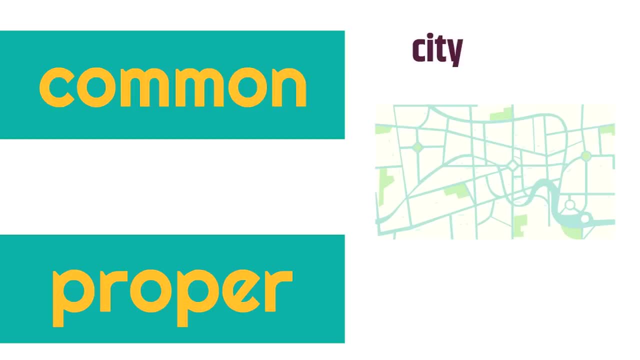 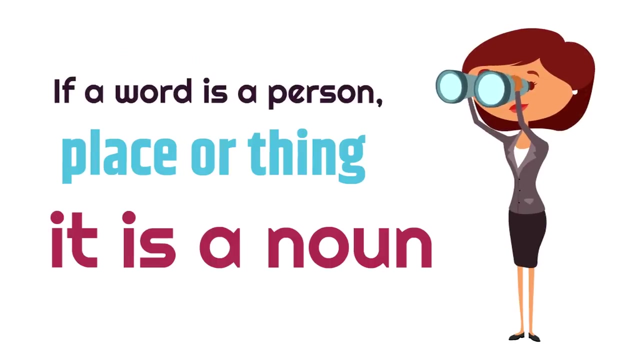 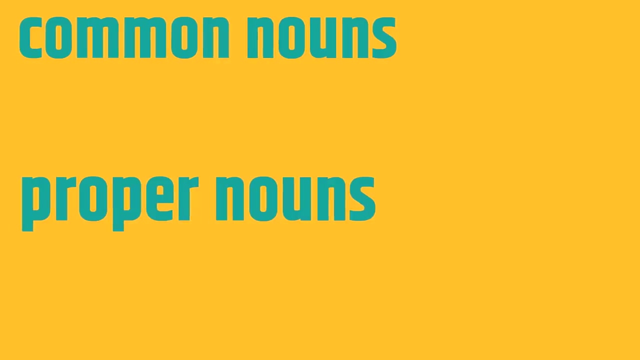 proper noun and notice it's an uppercase or capital letter, because it's the proper noun. it's the specific thing that it is. it's Denver to review if a word is a person, place or thing. it is a noun and there are two types of nouns: common nouns, which name a type of person, place. 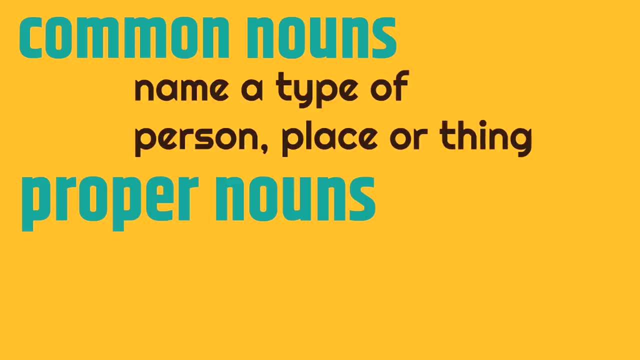 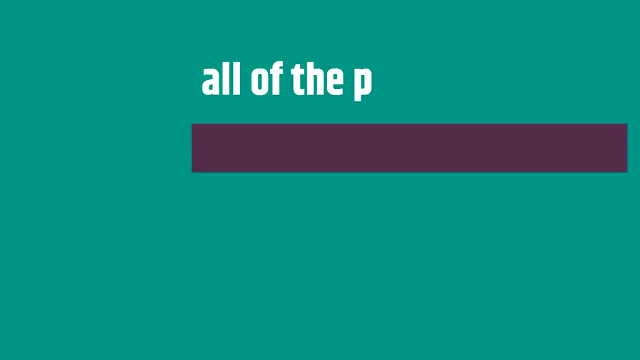 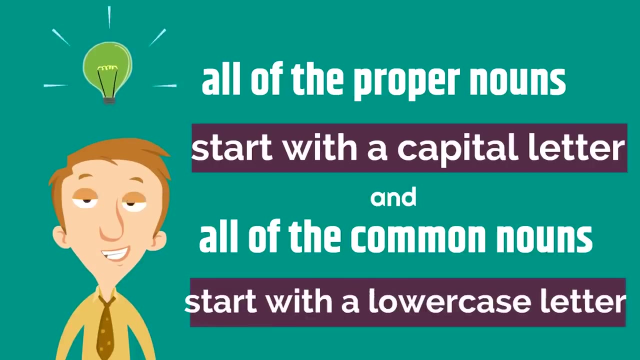 or thing, and proper nouns which name the specific person, place for thing. and, of course, all of the proper nouns start with a capital letter and all of the common nouns start with a lowercase letter. well, now we're going to play a quick game to see how much you've learned. 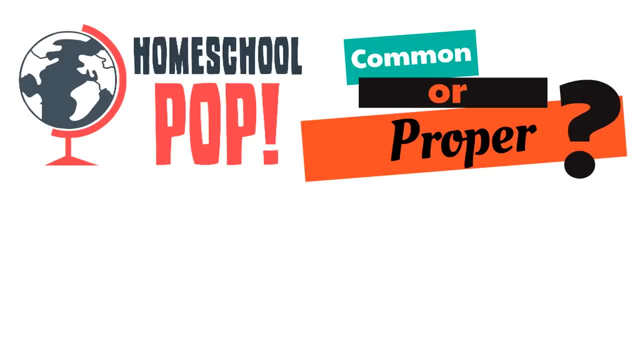 we're going to call this game common or proper. It's where we will share a noun with you and you tell us whether you think it's common or proper. Here's the first one. Sock, Is this a common or proper noun? 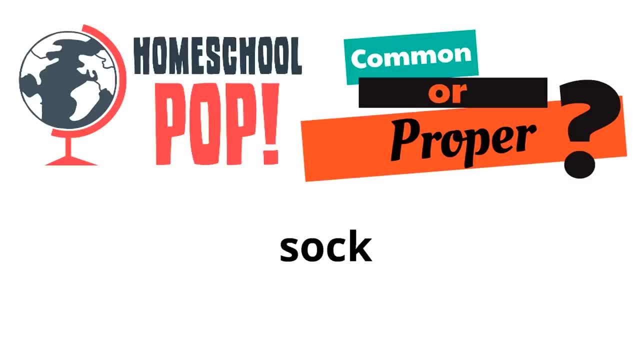 Is it a common or is it a proper? Yeah, it's a common noun. It's a type of thing. So we know it's a common noun, but also it starts with a lowercase letter. Sock is a common noun, Let's try this one, Mrs Barrow. Is this a common or a proper noun? 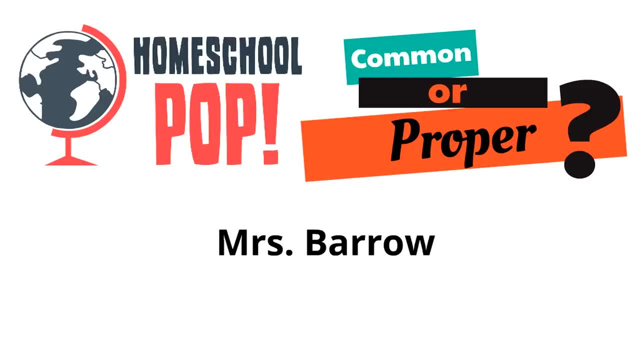 Yes, It's a proper noun, It's a specific person. We also have the clue that it has the capital letters. They start with capital letters. The capital M and the capital B tell us that this is a proper noun. Mrs Barrow is a specific person. This is a proper noun, Great job. 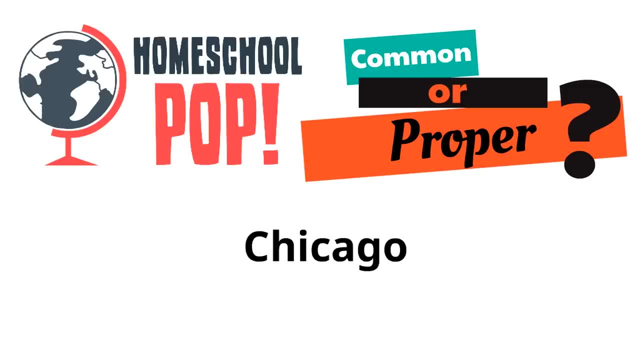 How about this one, Chicago? Is this a common or a proper noun? Yeah, it's proper, And we have two clues. The first one is that it's a specific place, Chicago. And also what's the other clue? Yeah, it starts with a capital letter. We know that Chicago is a proper noun. Great job. 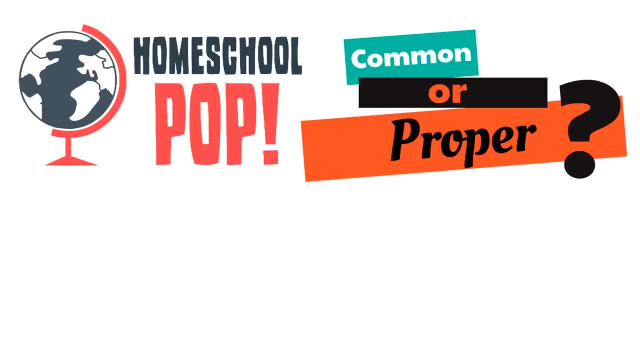 How about this noun Teacher? This might be a little tricky. Is this a common or a proper noun? Yeah, it's a common noun. It's a type of person. Also, what's the other clue that tells us that this is a common noun? 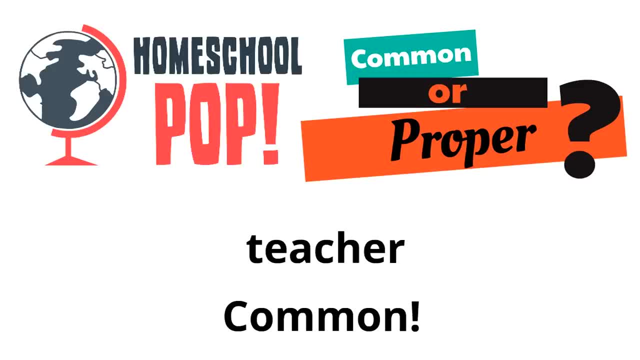 Uh-huh, The lowercase letter. The lowercase letter tells us this is a common noun. Let's try this one now. Box Is box common or proper? What type of noun is this? Yes, it's common, It's a type of thing. 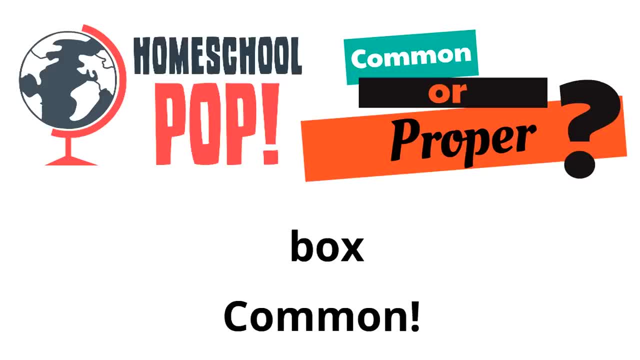 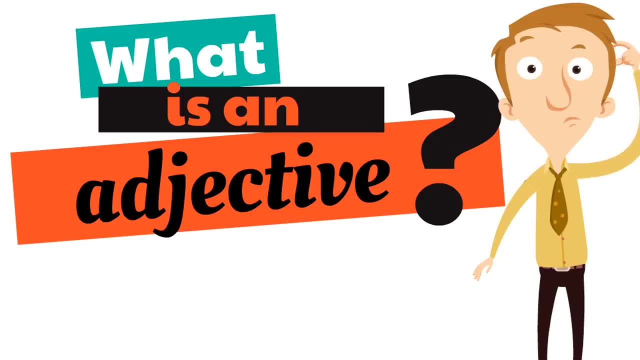 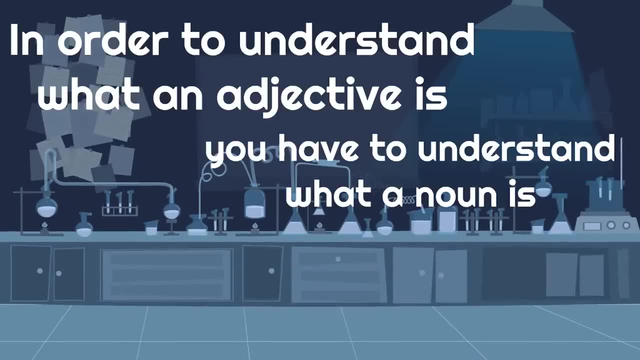 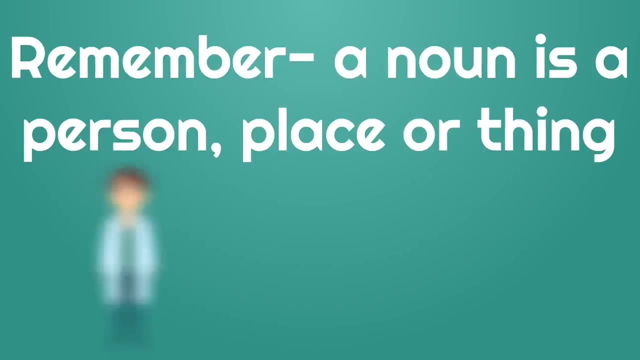 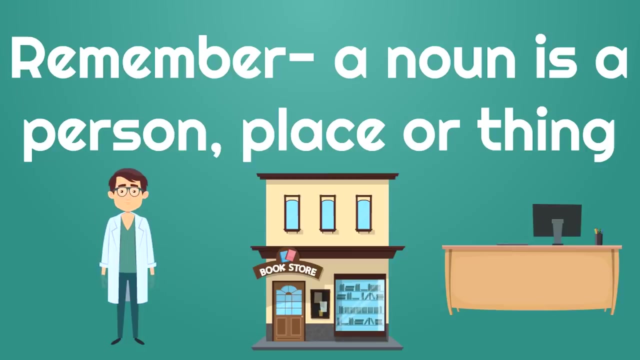 is an adjective. well, this might sound a little weird, but in order to know what an adjective is, you have to understand what a noun is. and remember: a noun is a person, place or thing: a person like a doctor, or place like a bookstore, or a thing like a desk. if it's a person, place or thing, it's a word, that's a noun. well, 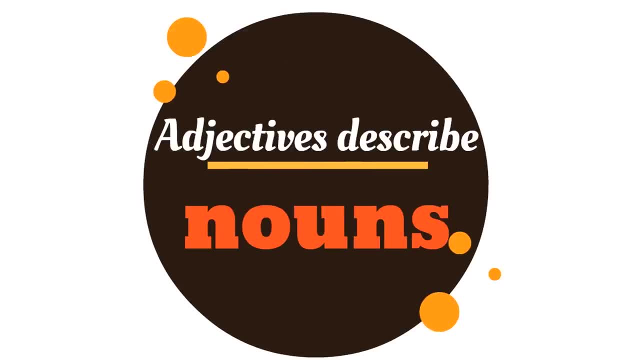 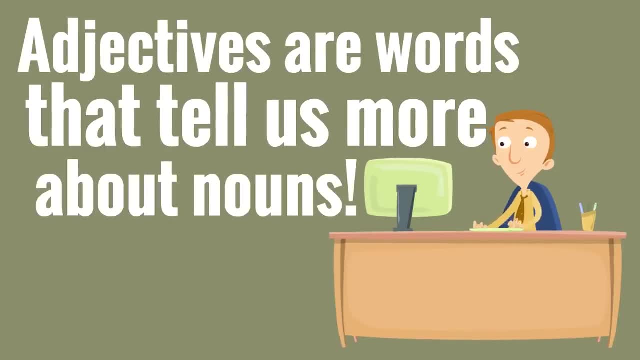 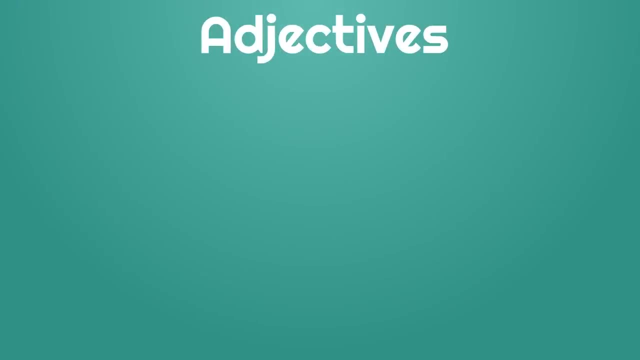 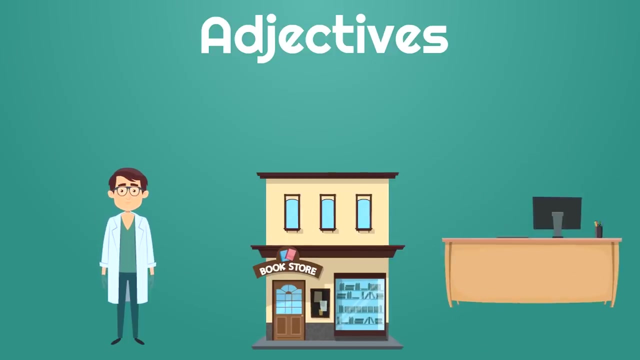 here's where adjectives come in. adjectives describe nouns. adjectives are words that tell us more about nouns. so let's look at some adjectives for these nouns that we shared: the doctor, the bookstore and the desk. the doctor- two adjectives we could use to describe this doctor- are tall and smart. 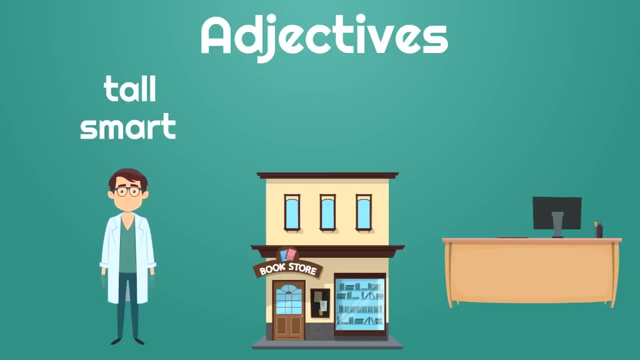 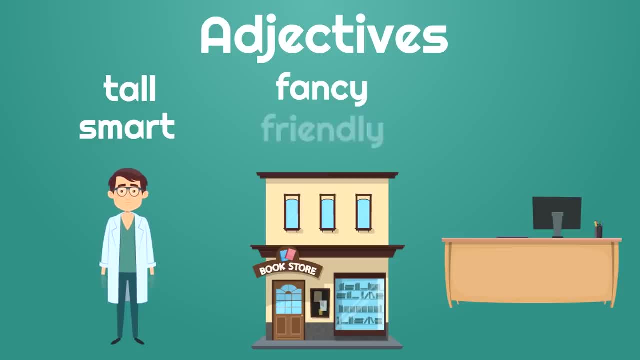 little bookstore and it also looks like it could be friendly. friendly is another adjective we could use to describe this bookstore. fancy and friendly are adjectives. they describe the noun well, what about this desk? well, two adjectives that could describe this desk are clean and tan. clean because you 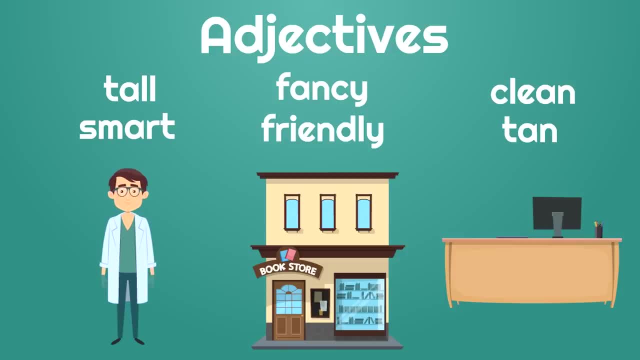 can see, it's not a dirty desk- and also tan, because that's the color of the desk. that describes the color of the desk. this is a tan desk. tan and clean are adjectives. they're describing the nouns. all of these words, you see, are adjectives: tall, smart, fancy, friendly, clean and tan. 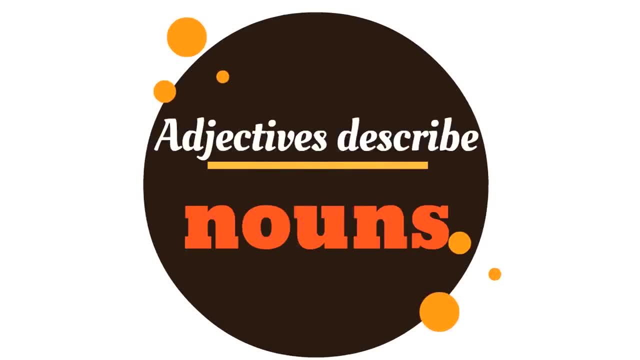 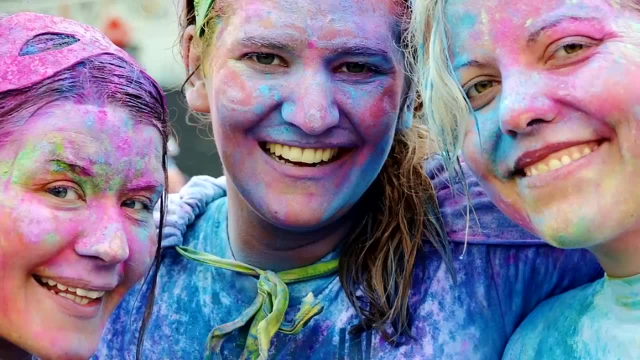 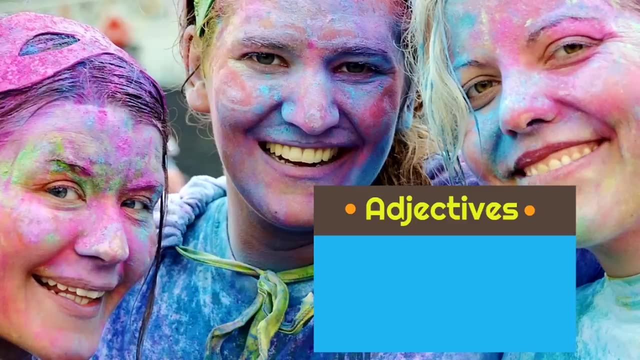 adjectives are pretty fun. all you have to remember is adjectives describe nouns. now let's practice using adjectives to describe nouns. look at this picture: these girls. how would we describe these girls? well, some adjectives we could use. we could use the adjective happy: they look. 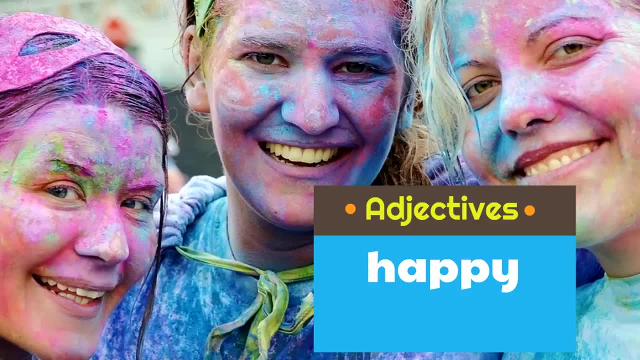 pretty happy. look at those big smiles. what else would describe them? do they look clean or do they look messy? yeah, they look pretty messy. messy is another adjective. happy and messy describe these girls. that's a pretty good job. now let's look at this picture. what are? 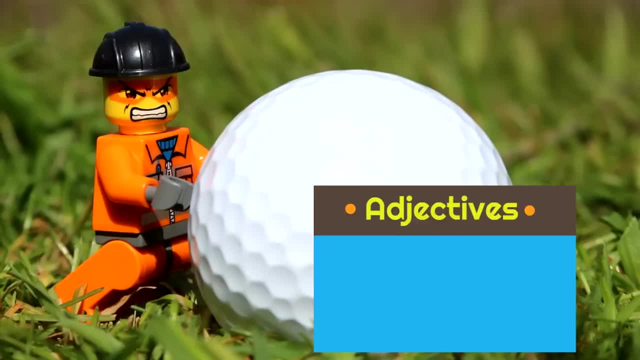 are two adjectives we could use to describe this Lego toy. Well, he looks a little angry, doesn't he? Angry describes him. That means angry could be a good adjective. What's another adjective? Is this toy very big? Look at this toy. compared to the grass, This toy is pretty. 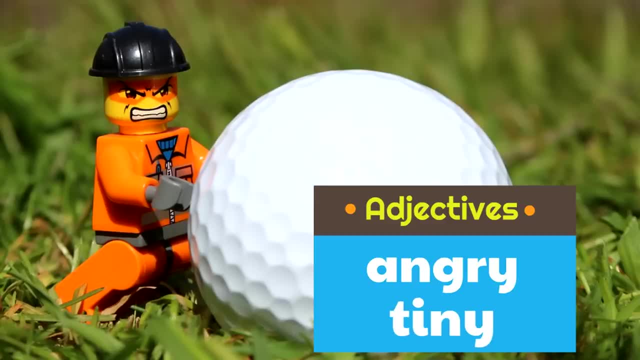 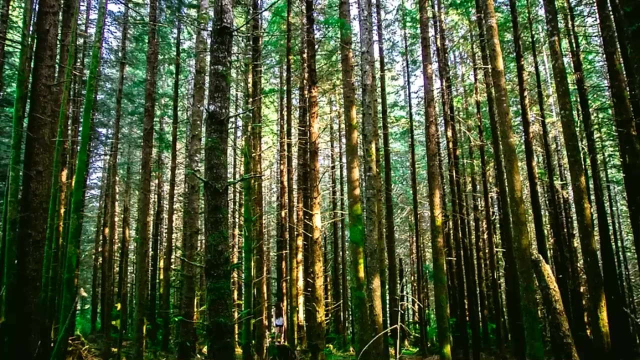 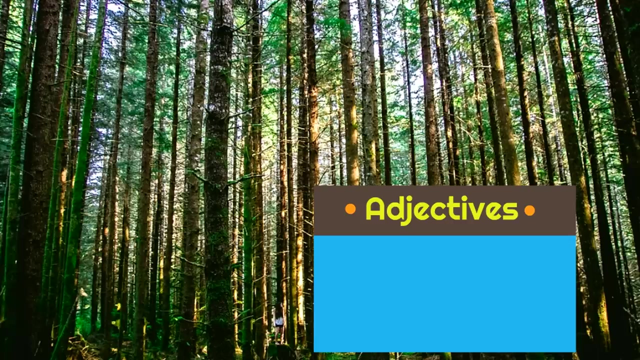 tiny. Tiny describes the toy in this picture, So the two adjectives we could use are angry and tiny. They describe the noun Wow. look at this picture. Look at all these trees. How would we describe these trees? What are some adjectives we could use to talk about? 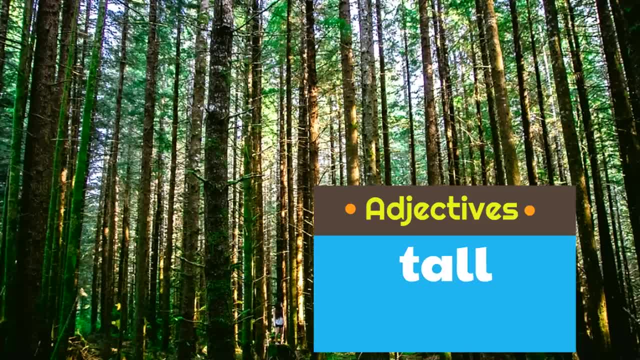 these trees? Well, these trees are tall, aren't they? They seem to reach all the way up to the sky. it looks like from this picture They are very tall. Something else about these trees- and we could tell this: because of just how tall they are, they must be very old as well. These are old trees. These aren't young. 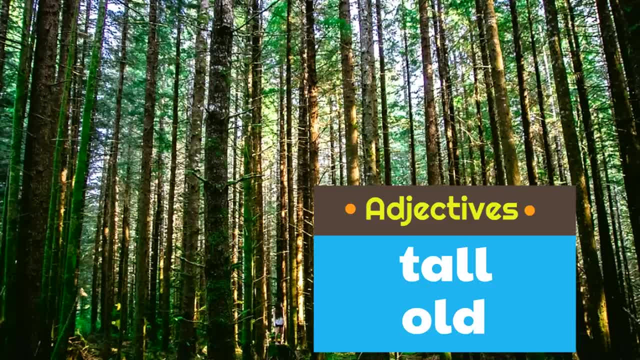 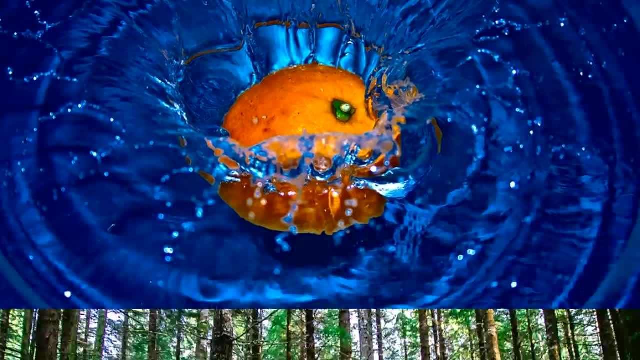 little saplings. These trees are tall and old. Tall and old are adjectives describing the trees. Oh, wow, look at this picture. How would he describe the trees? Well, these trees are tall and old. How would we describe, How would we describe, the water in this picture? 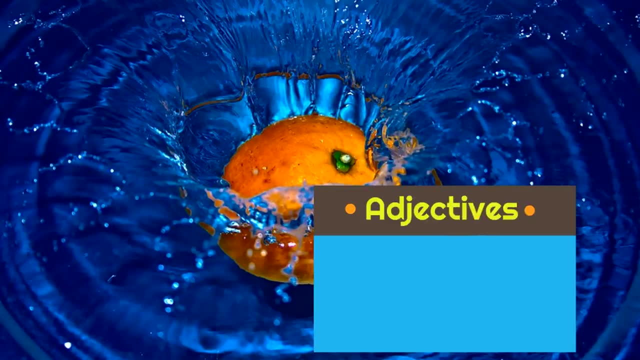 If the water is a noun, it's a thing. what are some adjectives we could use to describe it? Well, one of the first things we know about water is that it is wet. right, Whenever you get in water, you become wet because water is wet. 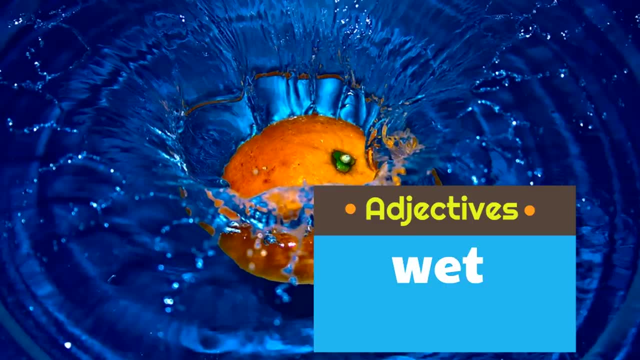 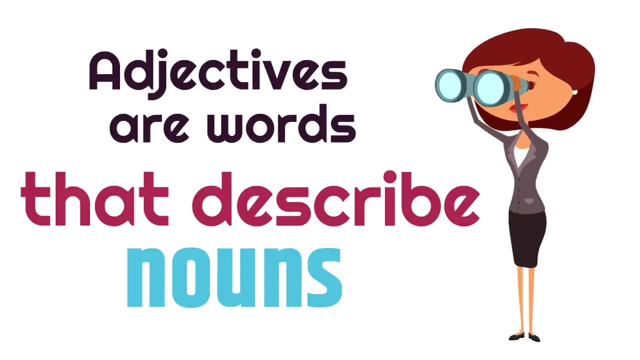 That's an adjective we could use. right, What's another adjective we could use? Look at the color. What is the color of the water? Yeah, blue, Wet and blue are adjectives describing the water. Adjectives are words that describe nouns. 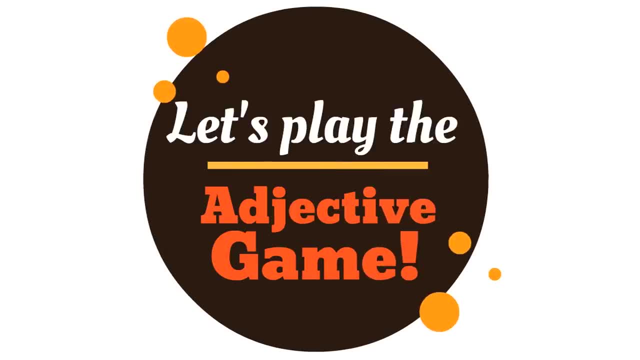 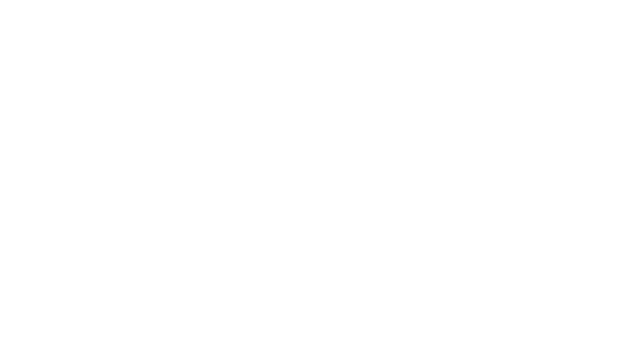 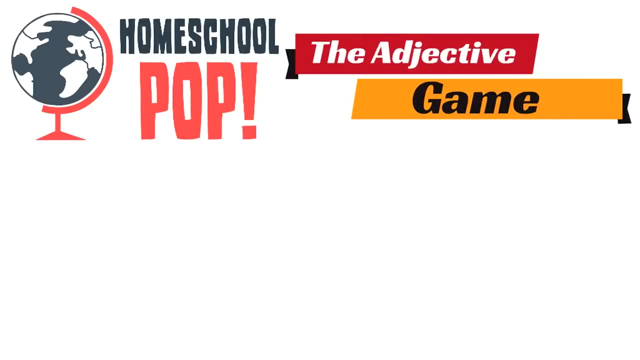 Alright, that was pretty cool. Now let's play the adjective game and find out how much you really learned. Okay, so here's how the game works. We're going to show you a sentence and you tell us which word is the adjective. It's kind of like a game where you hunt and find the adjective in the sentence. 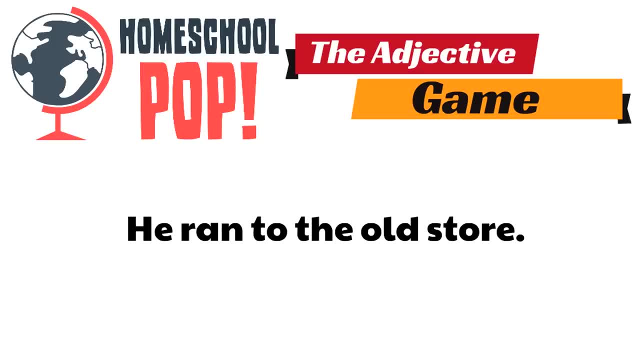 Let's get started. So here's the first one. The sentence says: he ran to the old store. Which word is the adjective Remember? adjectives describe nouns. Which word is the descriptive word? Adjectives describe nouns: Yeah, old. 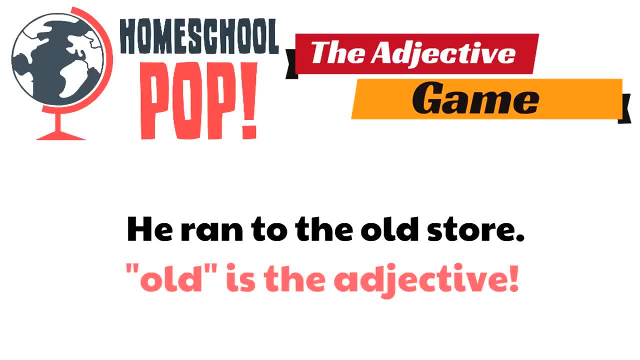 Old is the adjective. Awesome job, Here's the next one. The quick fox got away. Wonder which word is the adjective? Can you spot the adjective? Uh huh, The word quick. Quick is the adjective. Quick is describing the fox. 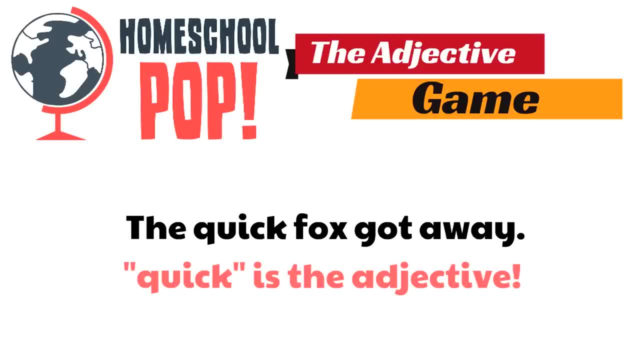 Quick is another word for fast. This is a quick fox that got away. Good job. Look at this one. It says he wanted to buy a new car. I think you might be getting the hang of it. Which word is the adjective? 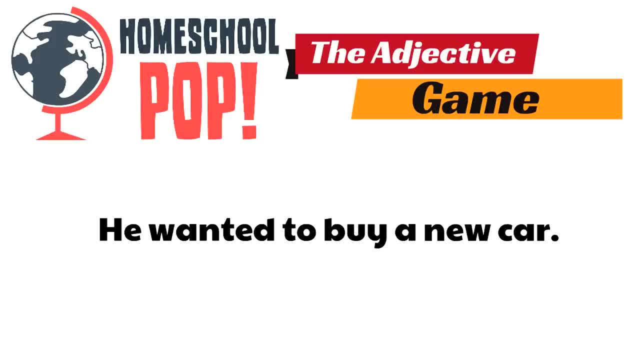 Yeah, The adjective is the word new, Because new is describing the noun car. Great job. New is the adjective. Okay, here's our last one. The birds flew past the big building. That's a long sentence. Can you pick out the adjective? 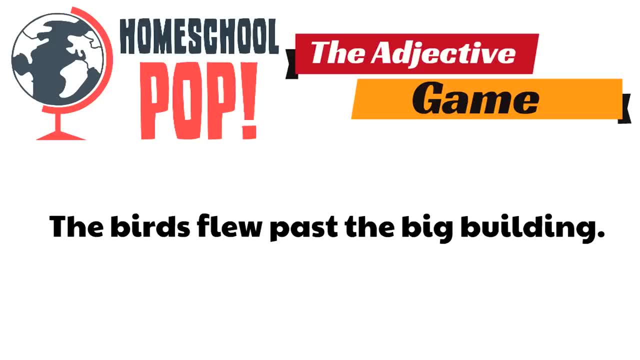 The birds flew past the big building. That's a long sentence. Can you pick out the adjective Big building? Which word is the adjective Big? Yes, And why is big the adjective? Uh huh, It describes the noun building. It's describing a noun. 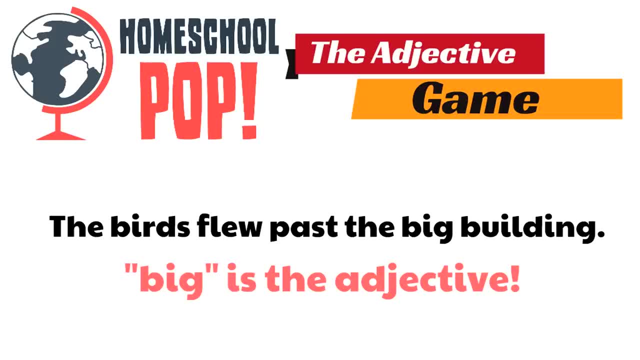 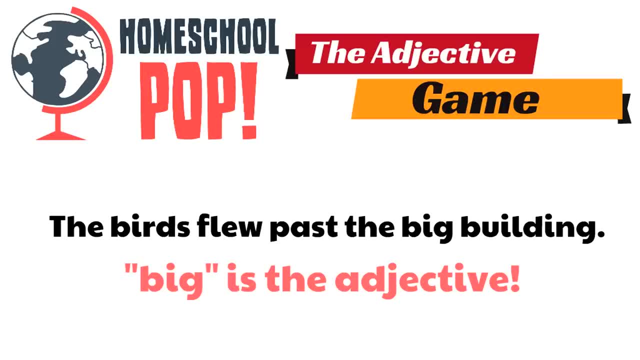 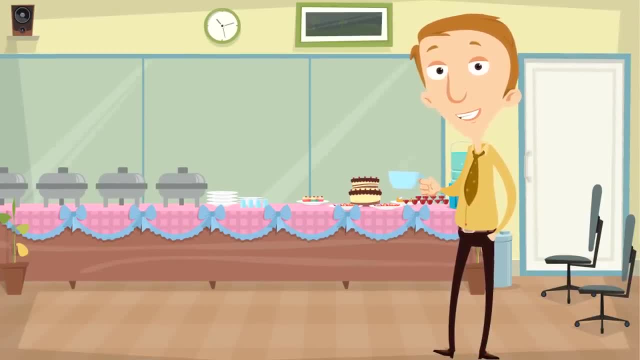 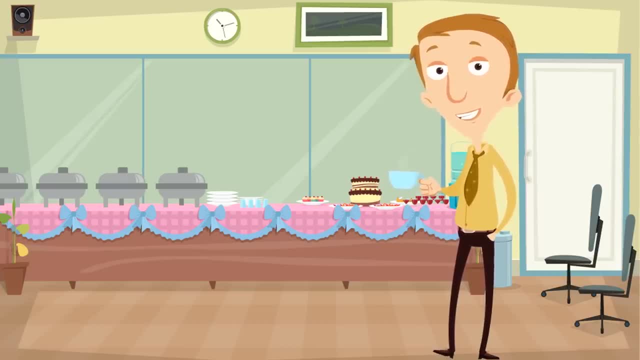 That's an adjective. I'm describing myself. Look at that cake on that table. Umm, I wonder what are in those silver bins. I bet there's some really yummy food in there. Better go. but remember you can use adjectives anytime. 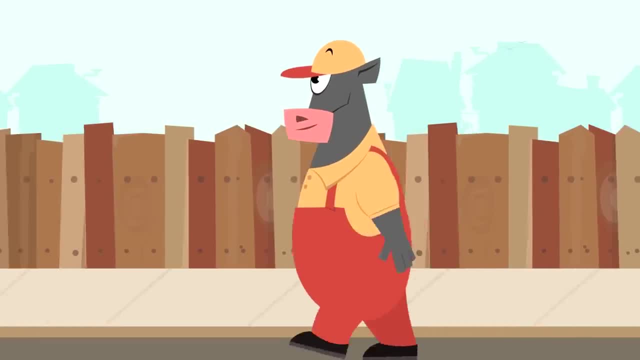 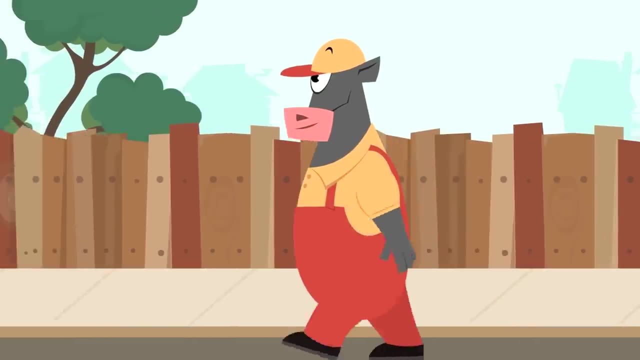 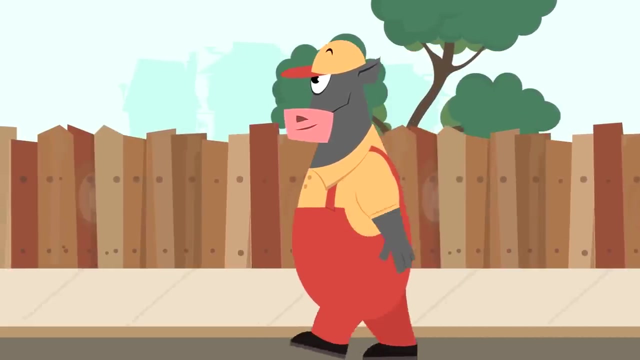 They're just words that describe nouns. Oh wow, Oh wow. look, it's the homophone cow. Homophone cow, Homophone cow. You're just walking, you're just going to ignore me. I see how it is Okay. so you're upset that we haven't included you in other videos. What do you call this? You know you're in a compilation video. That's cool too. 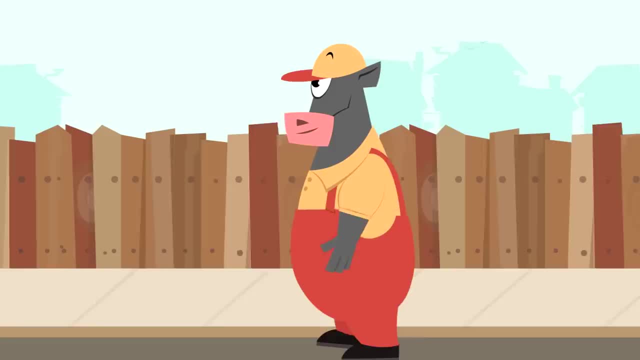 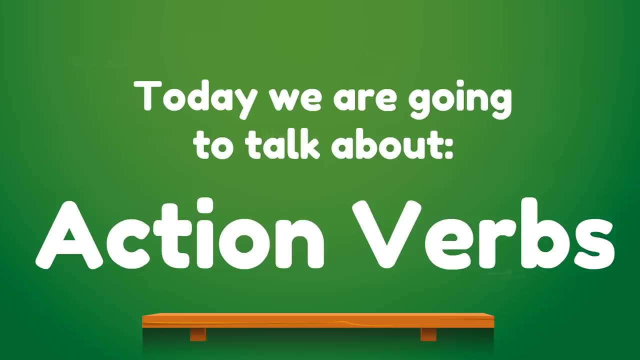 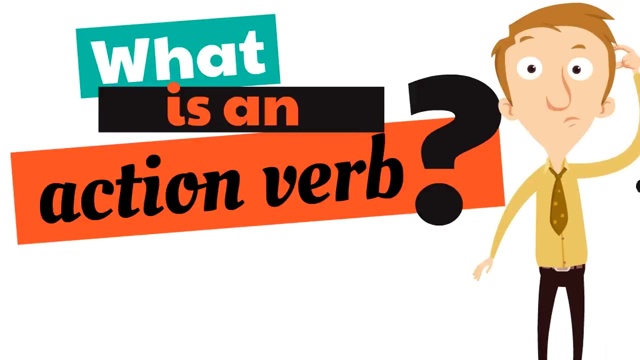 All right, I need to talk to the homophone cow, But in the meantime, let's learn about action verbs, which sounds exciting because it is exciting. Well, first things first, what is an action verb? Huh, What is an action verb? 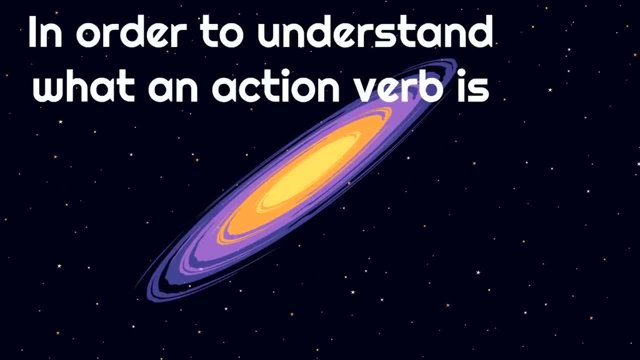 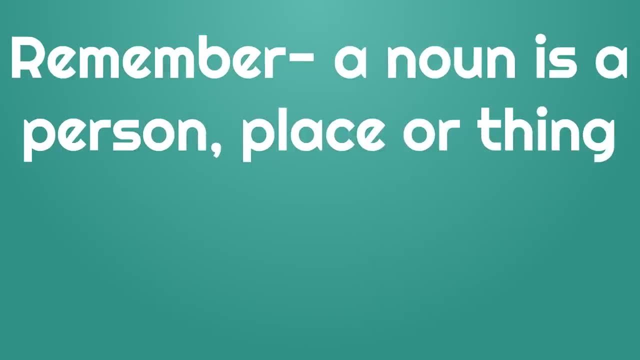 The truth is, in order to understand what an action verb is, you have to understand what a noun is. Remember: a noun is a person, place or thing. A person like a teacher. A place like a gas station. 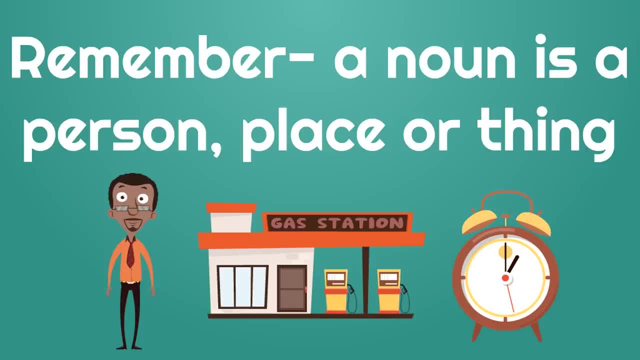 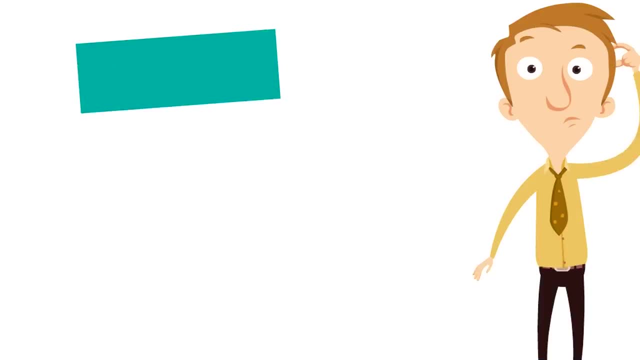 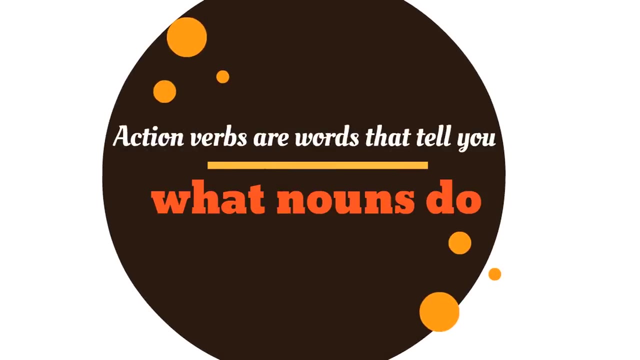 Or a thing like an alarm clock. If it's a person, place or thing, it's a noun. Okay, so what is an action verb? Well, action verbs, Action verbs, are words that tell you what nouns do. Oh, it's so cool. We'll say it again. 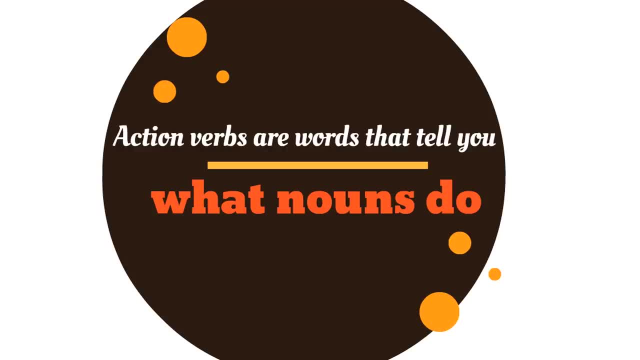 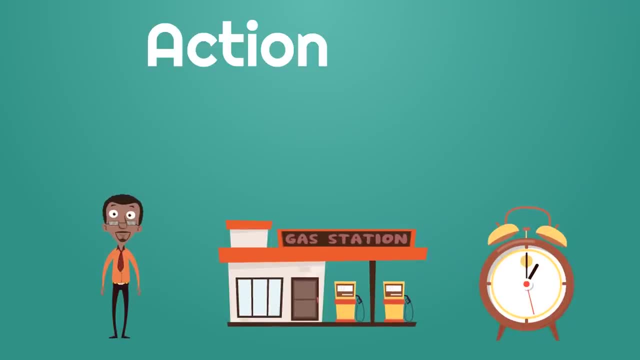 Action verbs are words that tell you what nouns do, And we'll give you some examples. All right, now we're going to look at some action verbs for the nouns we just saw. Remember, action words are words that tell you what nouns do. 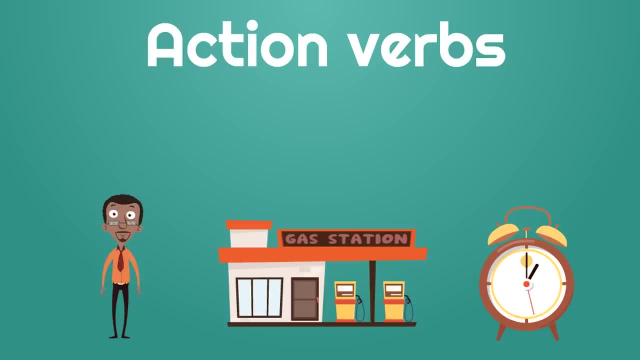 So our first one: what do teachers do? What does this teacher do? Yeah, he teaches. Teaches is a good action verb. It's what this noun does, what this teacher does. What else does this teacher do? This teacher helps. 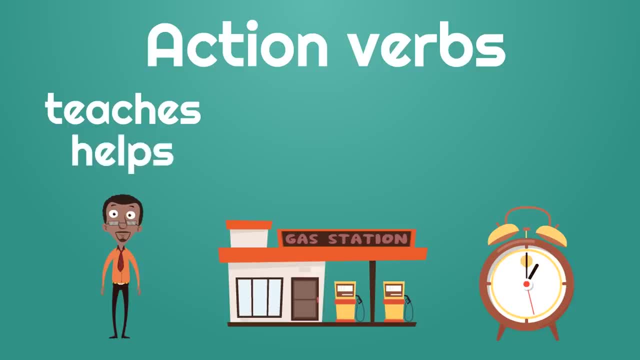 Yeah, All right on to the gas station. What does a gas station do? Well, a gas station sells, doesn't it? It sells gasoline and other things. What else does a gas station do? What's another action verb? Well, a gas station sells. 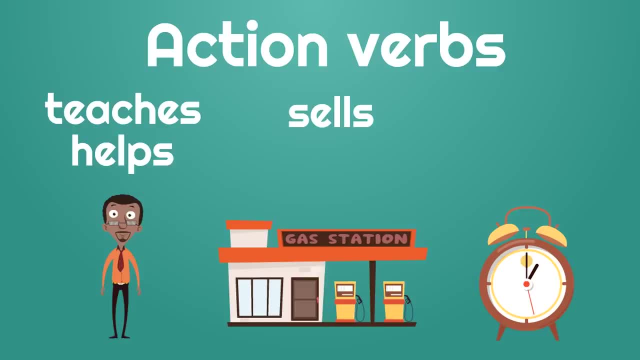 What else does a gas station do? What's another action verb for a gas station? Well, a gas station fuels. The gas station fuels your car. Fuels is an action verb. Great, let's try the alarm clock. What does an alarm clock do? 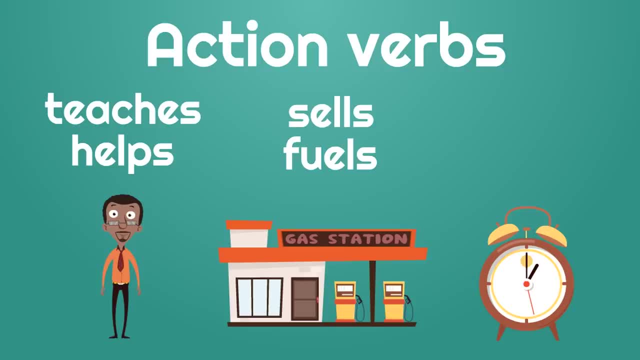 What are some action verbs that describe what an alarm clock does? Well, an alarm clock ticks, doesn't it? Tick, tick, tick, tick. That's one action verb for an alarm clock. Another action verb. let me give you a hint. 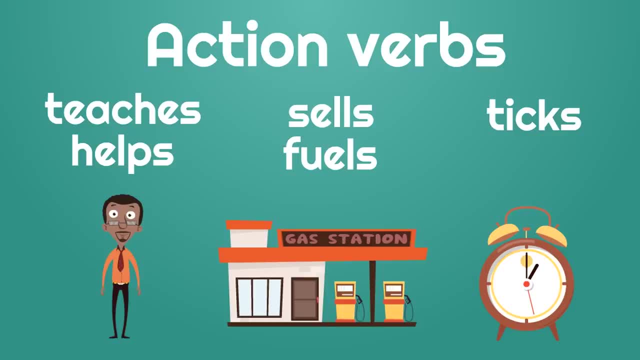 This is what an alarm clock does when you need to wake up. What does an alarm clock do when you need to wake up? It rings, Yeah, an action verb is rings. Action verbs describe what nouns do. A teacher teaches and helps. 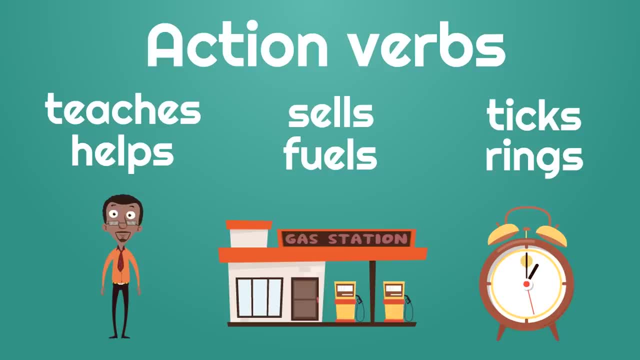 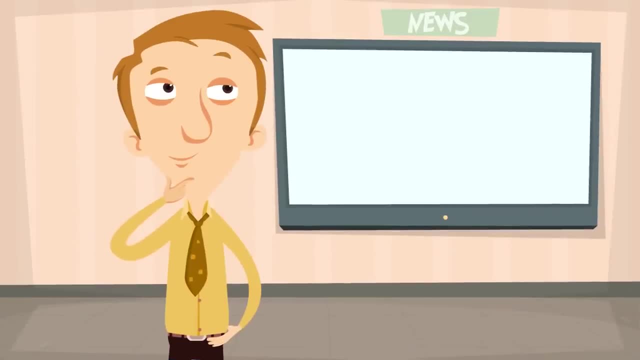 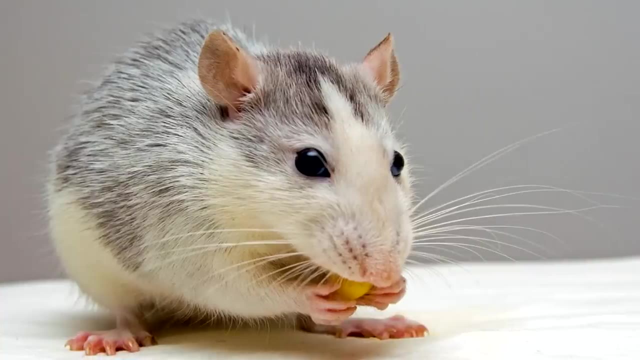 A gas station sells A gas station fuels, And an alarm clock ticks and rings. Huh, let's think of some more real life examples of action verbs. Awesome. here's a picture of a rat. Pretty cute for a rat. Most people think mice are cute. 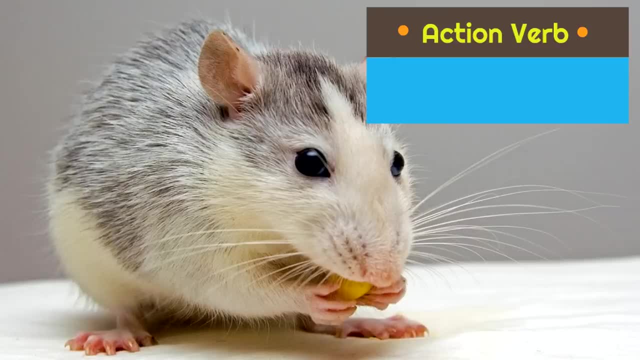 Mice are cute too. Rats can be cute, just so you understand. Now, what does this rat do in the picture? What is the action verb? What does this rat do? Yeah, this rat eats. Great job. eats is the action verb. It's describing what this noun does. 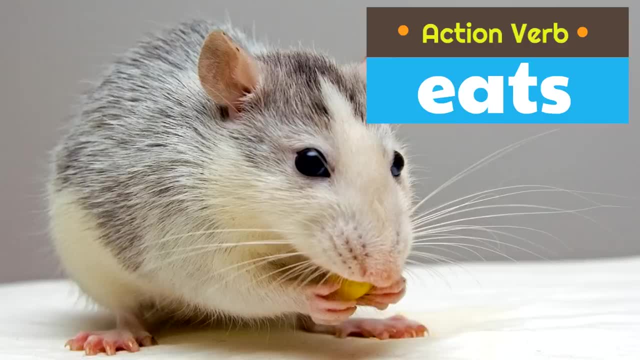 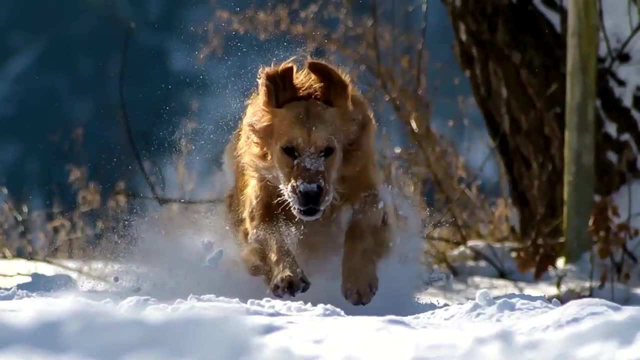 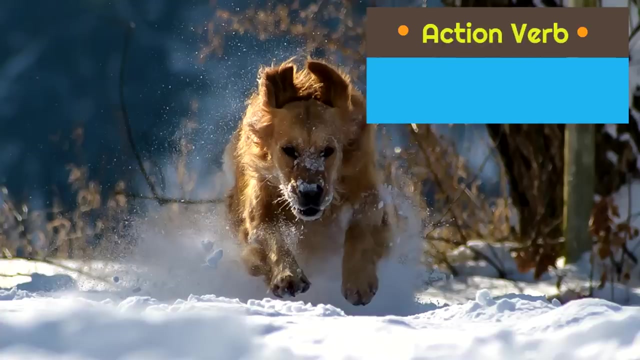 What does this rat do? this rat eats. eats is the action verb. Let's look at this picture. What does this dog do in the picture? What does this dog do? What's the action verb? Yeah, this dog runs. the action verb for this picture is runs. this dog runs. 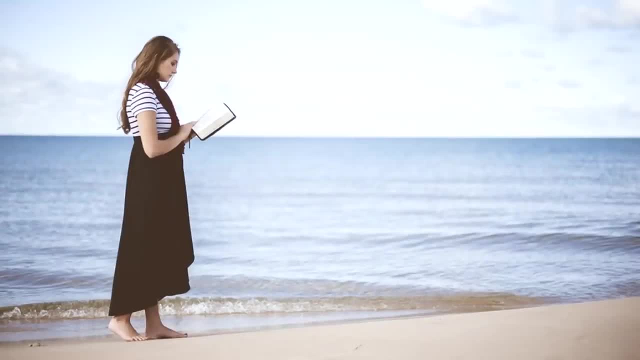 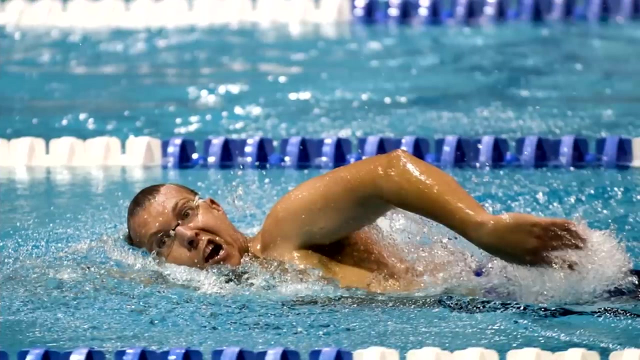 Cool, let's look at this one. What does this lady do in the picture? What does this lady do? What is the action verb? Uh-huh, This lady reads. Reads is the action verb. Good job, Wow, look at this. what does this man do in the picture? What's the action verb? 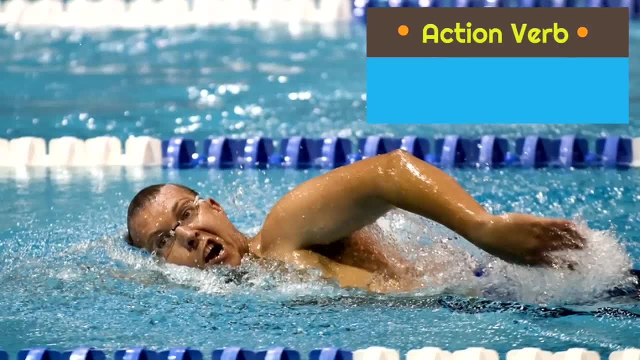 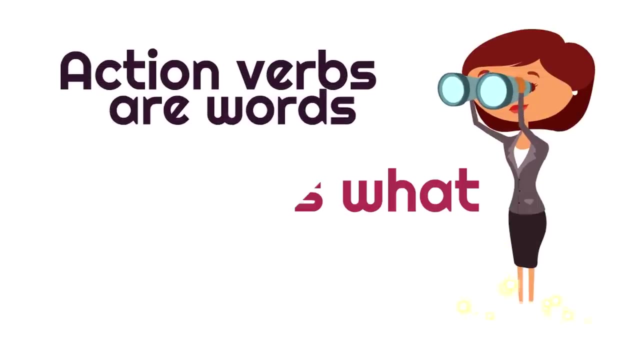 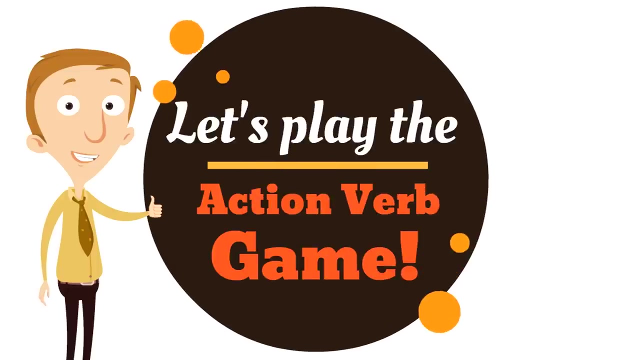 What does this man do? Aha, yeah, this man swims. Swims is the action verb. awesome. Action verbs are words that tell us what nouns do. All right, you're ready. You might not feel like it, You're ready. You know this action verb stuff. You're doing a great job. 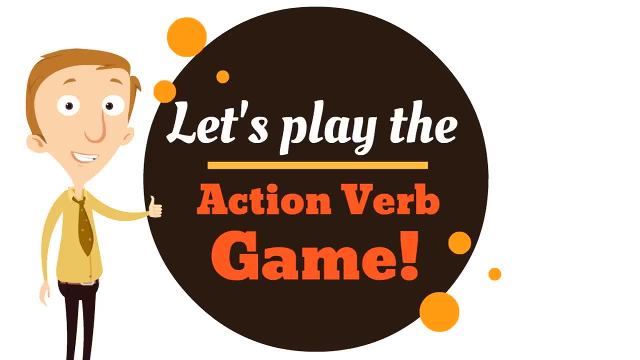 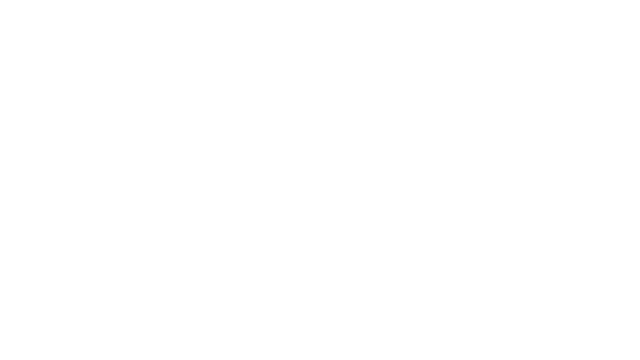 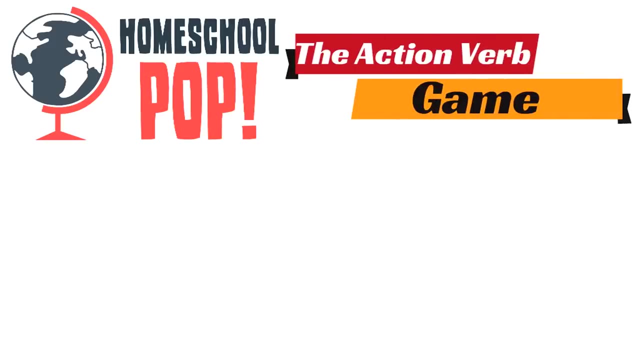 Let's play the action verb game. Yes, Okay. so here's how we play the action verb game. We're gonna show you a sentence and you tell us which Word you think is the action verb. Let's get started. Okay, here's our first one. the little girl sang. 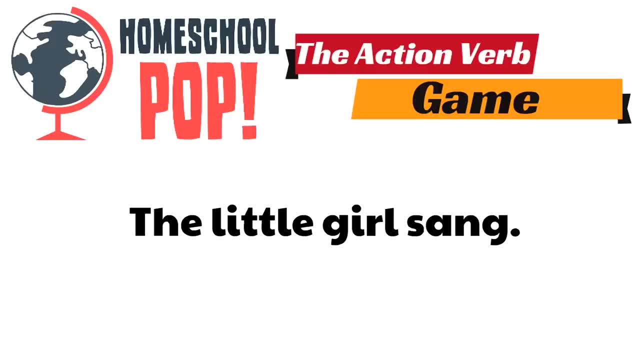 The little girl sang. which word is the action verb? Yeah, sang Sang is the action verb, because it tells us what the noun does. Good job, Let's try this one. he speaks to his mother. He speaks to his mother. Which were is the action verb? Aha. 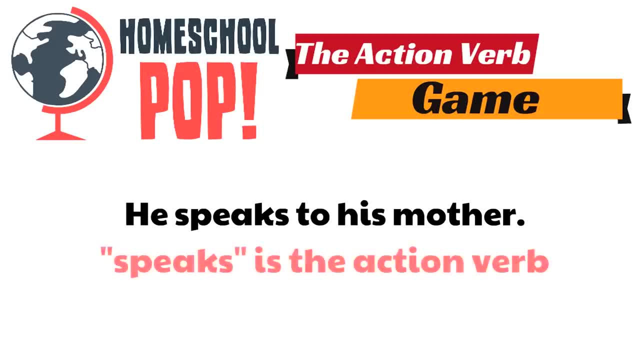 speaks. speaks is the action verb. It's the word that tells us what the noun does. the noun he speaks. Speaks is the action verb. Good job, Okay, let's look at this one now. they grow flowers. They grow flowers. Which word is the action verb? 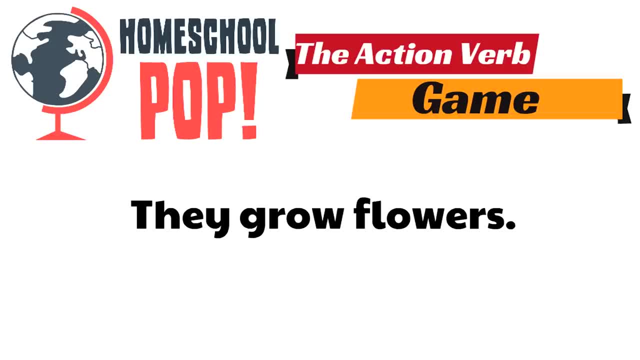 You've got the hang of this awesome Grow. grow is the action verb. It's the word that tells us what the noun does: Good job, good job. Okay, the last one: the kids watch homeschool pop. This is a cool one. The kids watch homeschool pop. which word is the action verb? 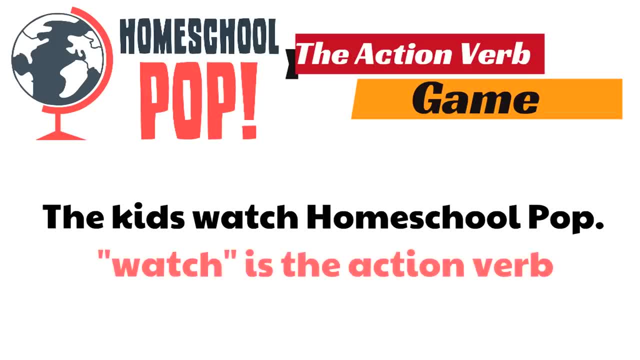 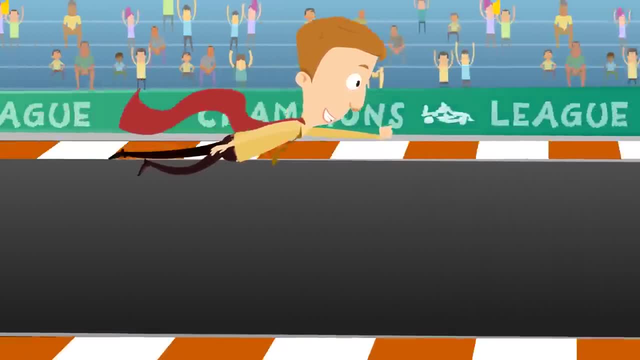 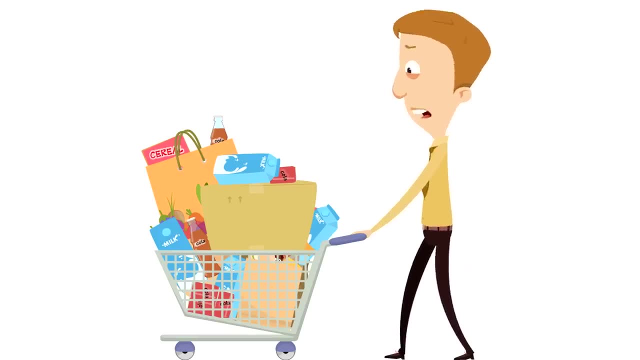 Yeah, watch is the action. to new adventures we fly. fly is an action verb, it's what i do. oh, this is such a heavy cart. oh, my goodness. oh, it's hard work. you know, a lot of times learning can be hard work too, but we hope that these videos are really helpful, make learning fun. 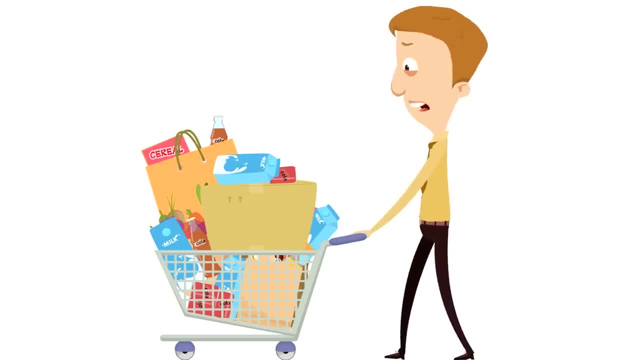 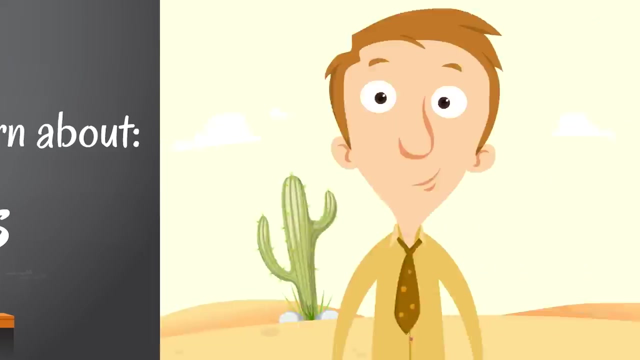 so that learning isn't hard like pushing this cart. oh, my goodness. all right. what's the next thing we should learn about? let's learn about pronouns: how to use them, how to spot them and how to have fun with them. of course, first we got to figure this out: what is a pronoun? 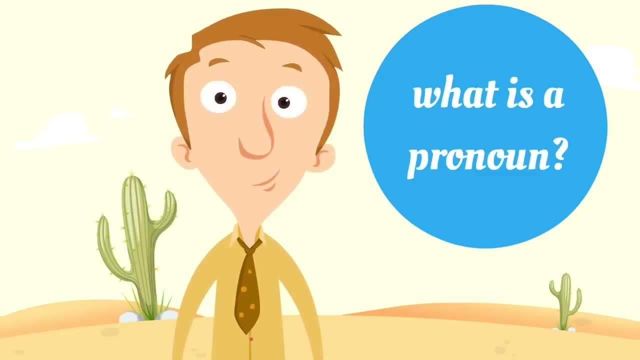 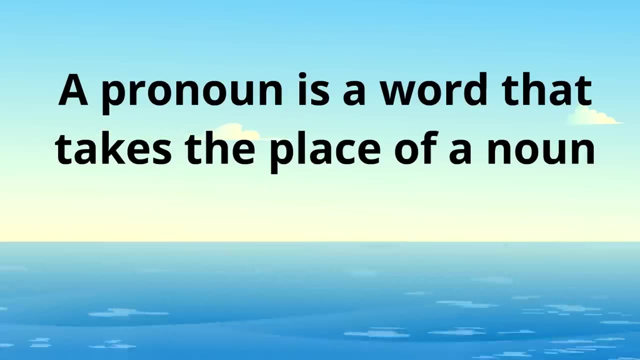 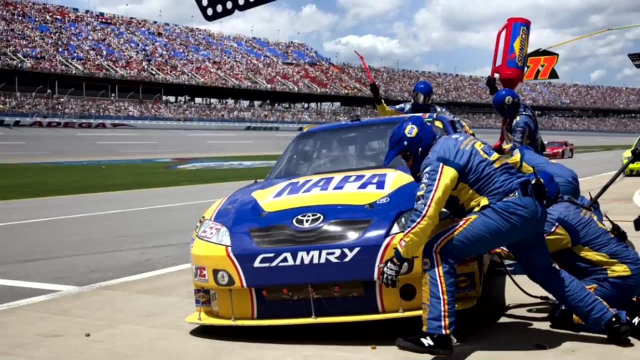 that's a good question. what is a pronoun? a pronoun is a word that a pronoun is a word that a pronoun is a word that takes the place of a noun. here we have a picture of a pit crew that is working on this stock car during a race. now this 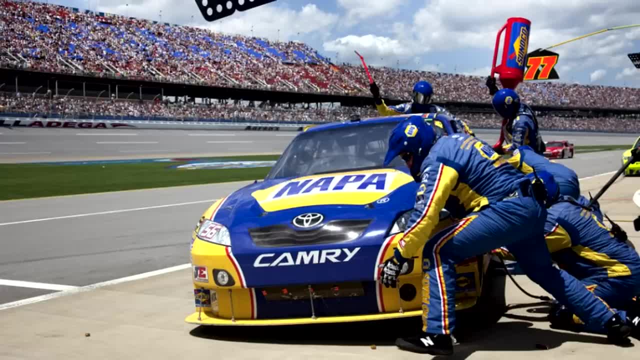 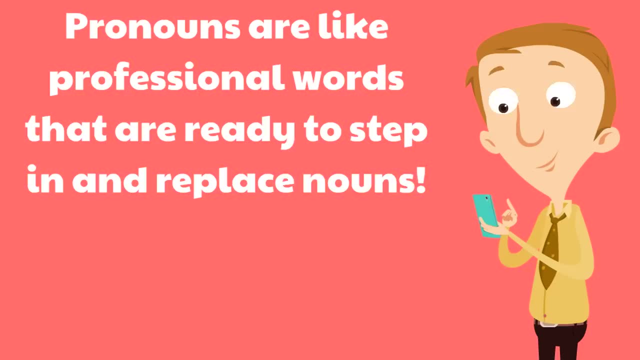 pit crew is made up of professional mechanics. these mechanics are pros. they're always ready to step in and do a very special job. pronouns are like professional words that are ready to step in and replace no Kind of like this pit crew stuck in a manicure. 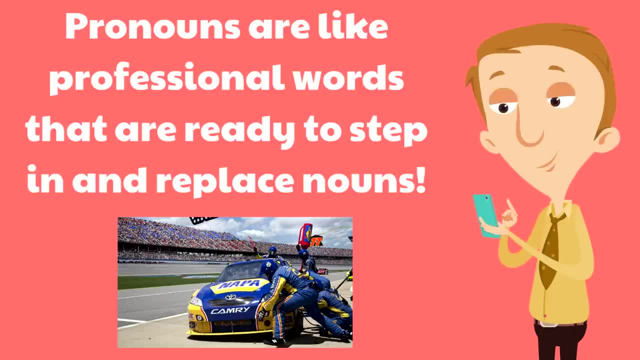 no kind of like this pit crew. they're professionals, they're ready for a special job, they're good at what they do. they're pros- pronouns are pros- at replacing nouns. pronouns are pros placing nouns cı. Maybe you can find something when you're making music. 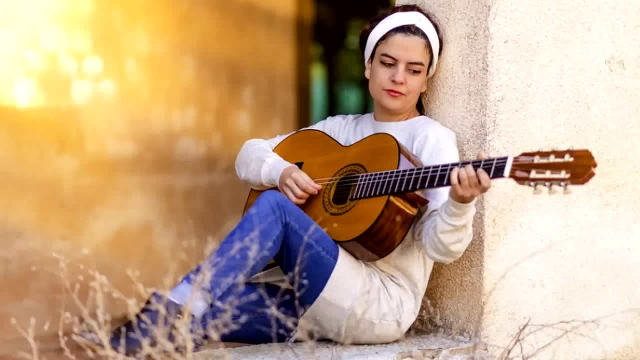 let's give you an example. okay, so here is a picture of a woman playing a guitar, a wonderful musical instrument. Let's say, this woman's name is Betty, so the sex album its арty аб Zoom to know about aguagaster- is Betty, so the sex album is Betty2. 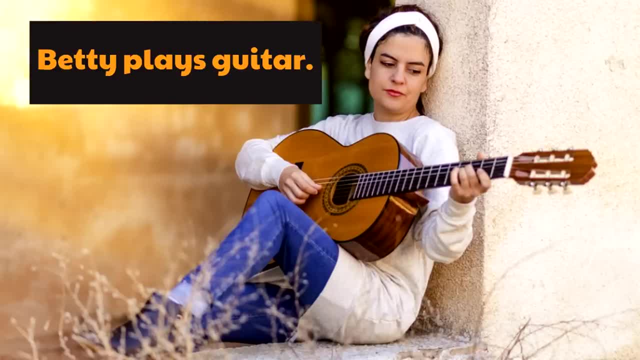 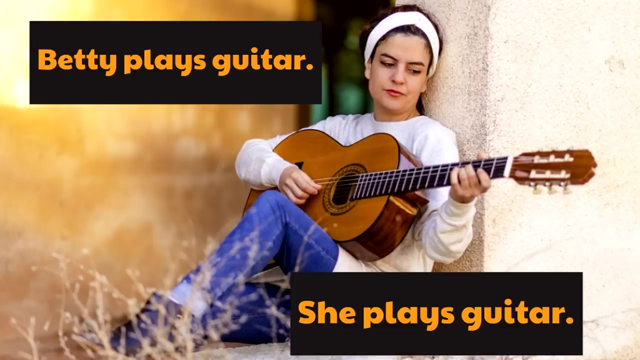 So the sentence is: Betty plays guitar. Betty plays guitar. Now let's change the sentence so it includes a pronoun: She plays guitar. She plays guitar. Did you see what happened there? Oh my goodness, that's so cool. 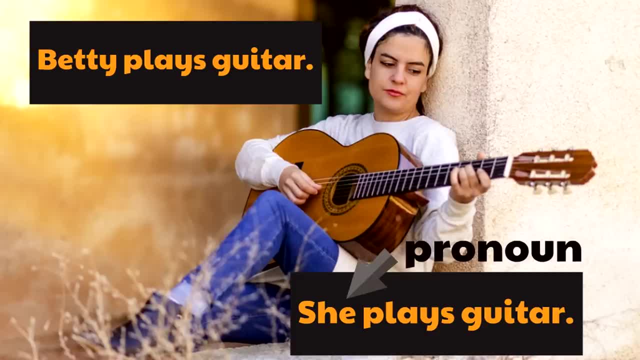 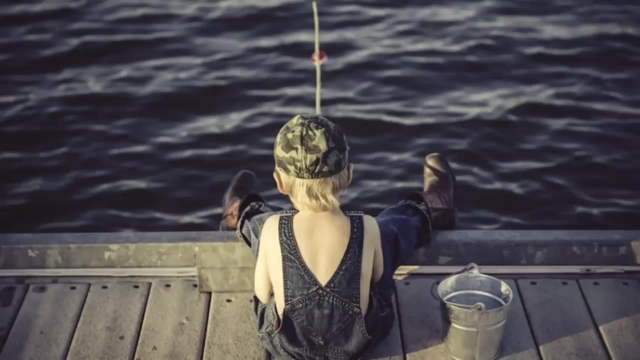 She is the pronoun, Because it is a word that takes the place of the noun, which is the name Betty. She replaced the word Betty. She is a pronoun. Okay, here's another one. Here's a picture of a boy who is fishing. 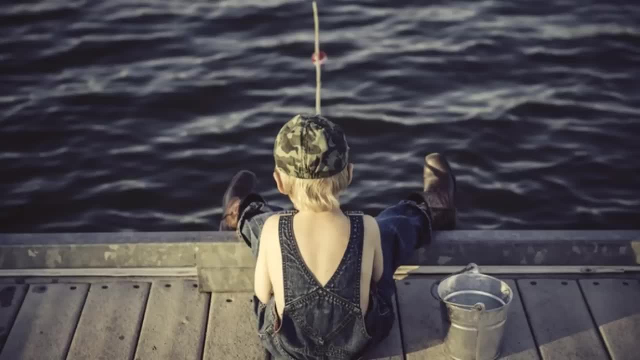 Let's say: this boy's name is Henry. okay, So the sentence is: Henry went fishing. Henry went fishing. Now let's change the sentence so it includes a pronoun. So the new sentence would be: he went fishing. 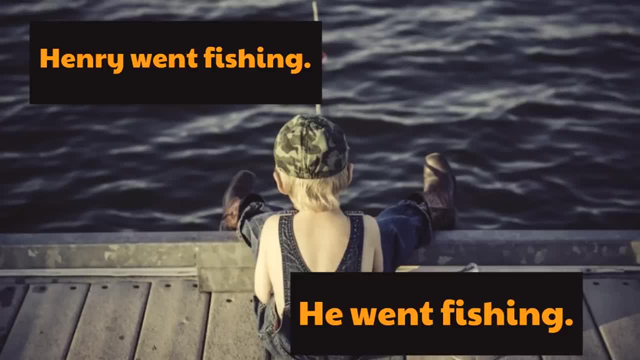 He went fishing. Isn't that cool. He is the pronoun Because it is a word that takes the place of the noun, which is the name Henry. He is the pronoun. Remember: a word like that takes the place of a noun. 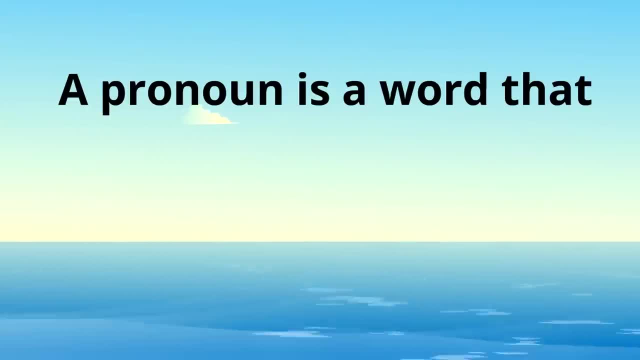 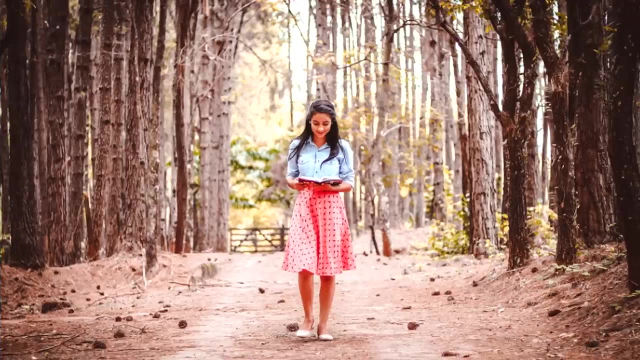 Remember, a pronoun is a word that takes the place of a noun. That's the job of a pronoun: to take the place of a noun. Okay, time for another example. Here is a picture of a young woman who's reading a book. 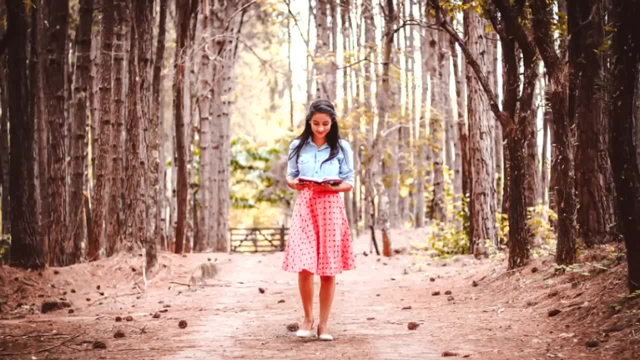 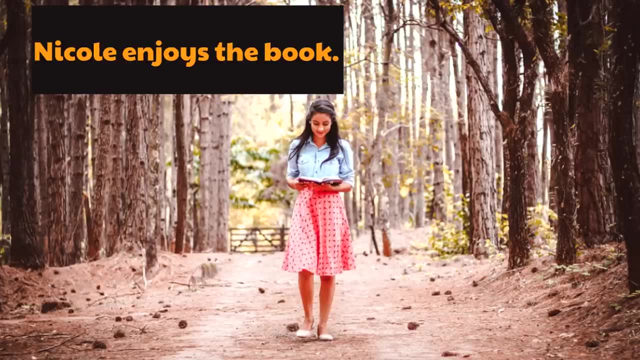 Let's say her name is Nicole And it looks like she's smiling a little bit, So let's make this the sentence: Nicole enjoys the book. Nicole enjoys the book. Now let's change the sentence so it includes a pronoun. 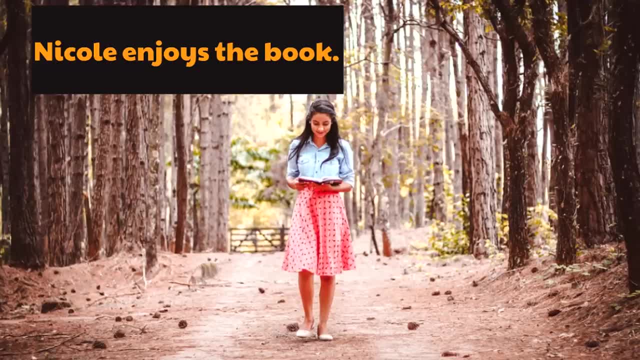 This time, instead of replacing a name with a pronoun, we're going to replace a common noun with a pronoun. We're going to replace book. So our new sentence is: Nicole enjoys it. Nicole enjoys the book. Nicole enjoys the book. 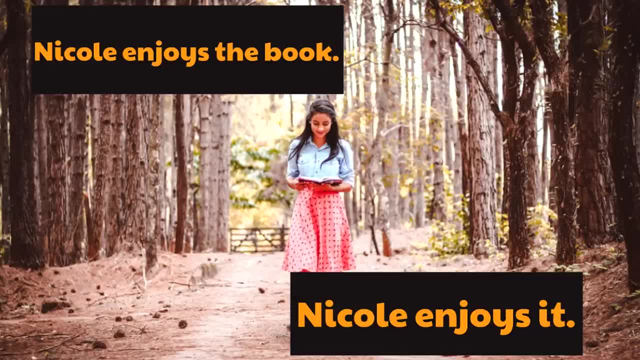 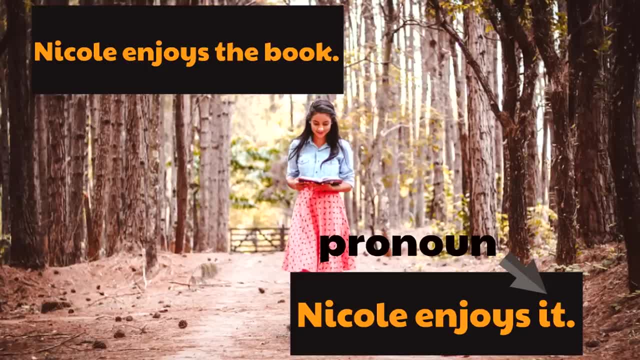 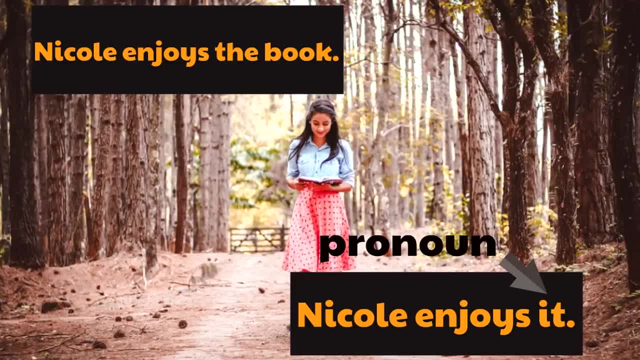 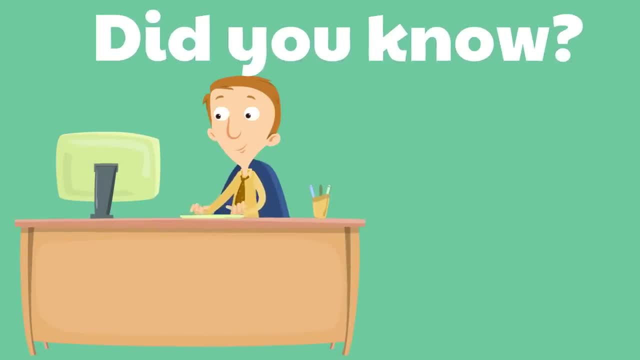 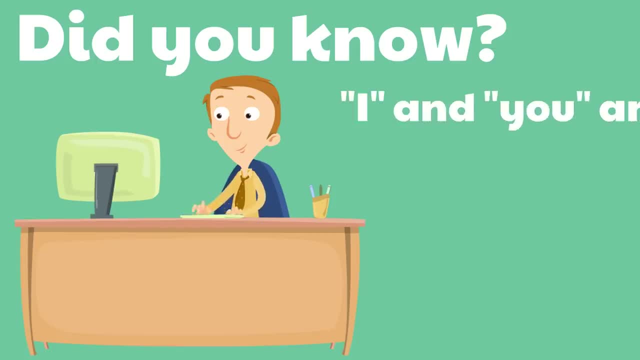 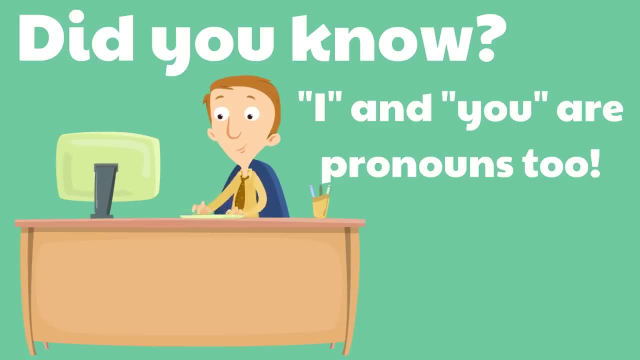 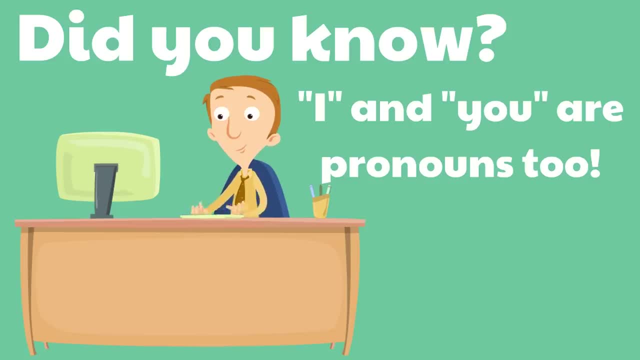 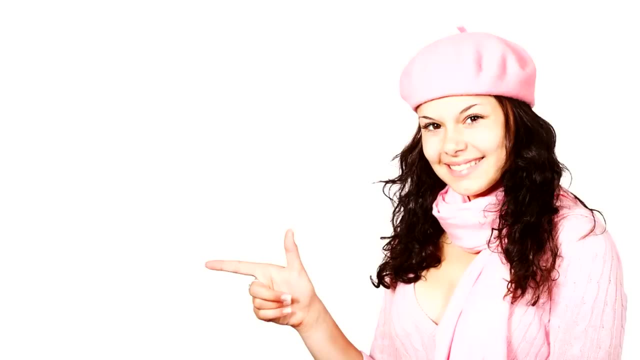 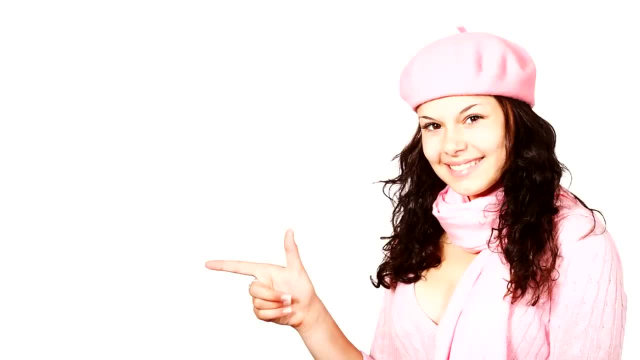 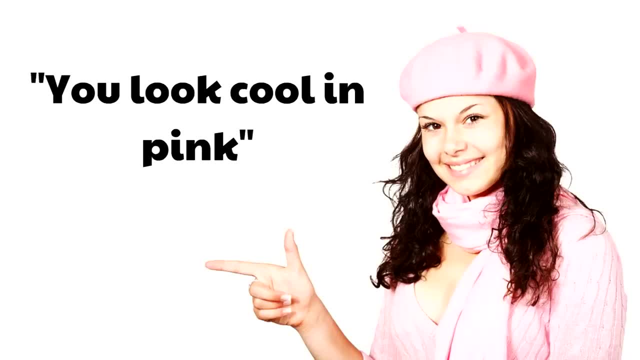 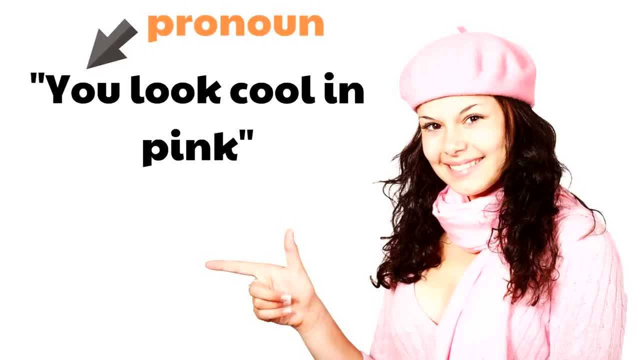 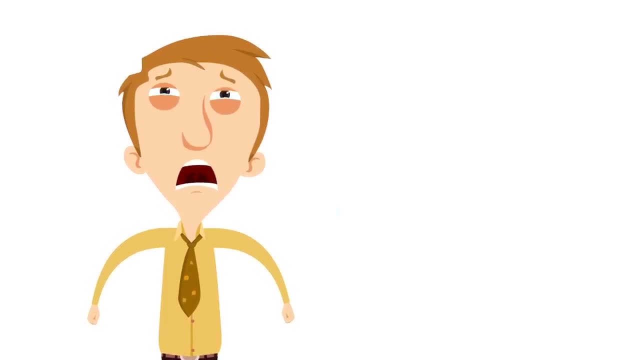 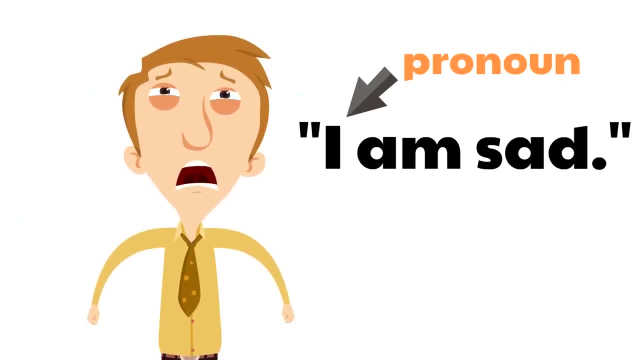 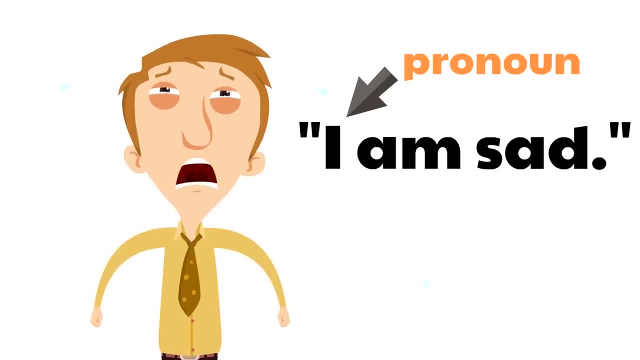 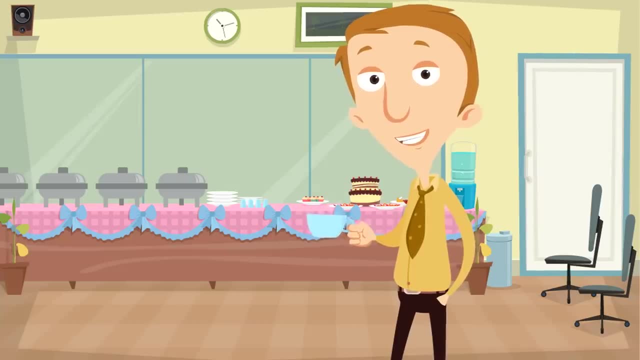 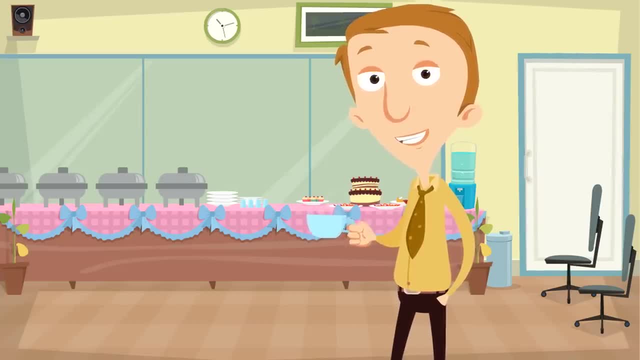 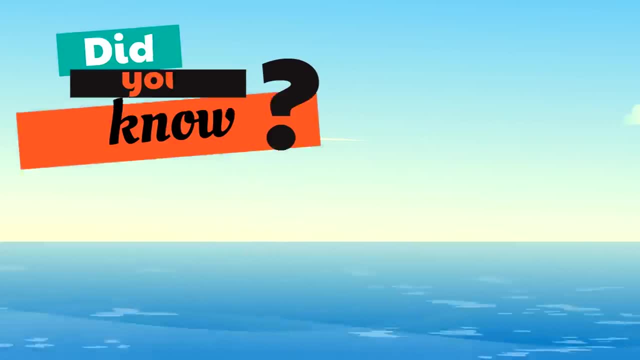 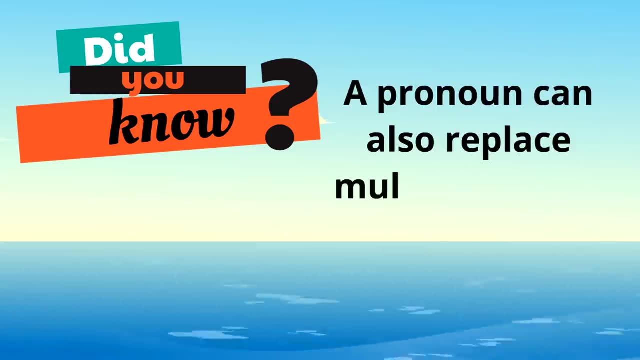 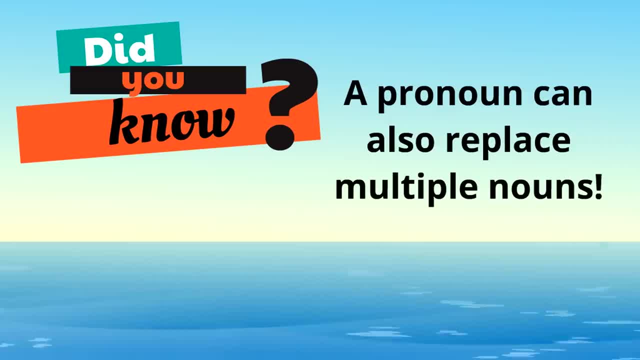 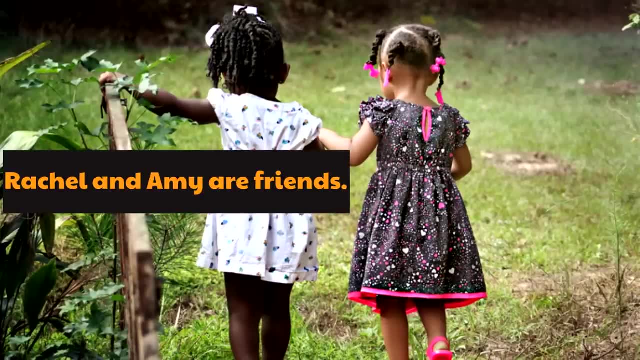 A pronoun can also replace multiple nouns. Let's say we have a sentence: Rachel and Amy are friends. Rachel and Amy are friends. Now let's try replacing two nouns, Rachel and Amy, with a pronoun. Our new sentence would be: they are friends. 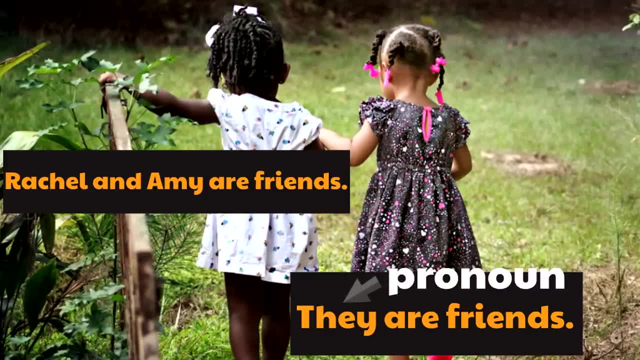 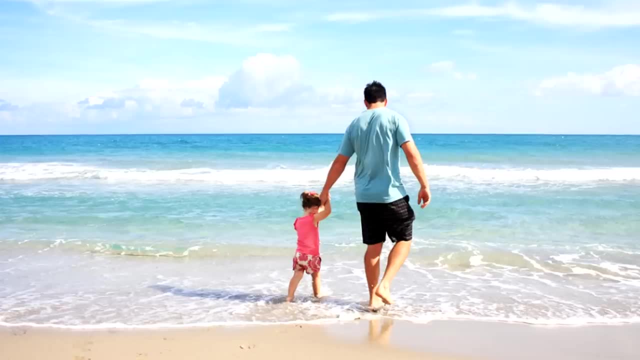 The word they is a pronoun because it's replacing the nouns Rachel and Amy. They is a pronoun. Let's try another plural pronoun That's a pronoun that replaces multiple nouns. Okay, let's say, this little girl likes to walk on the beach and she says this sentence: 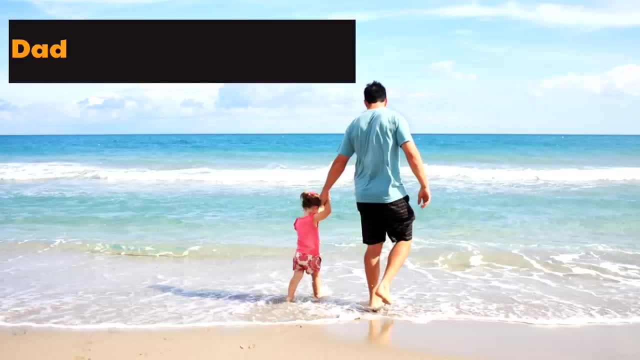 dad and I love the ocean. Now, this one's a little weird. The word dad is a proper noun because she calls him that. That's his name. that he's called by his daughter is dad. So dad in this sentence is a proper noun. 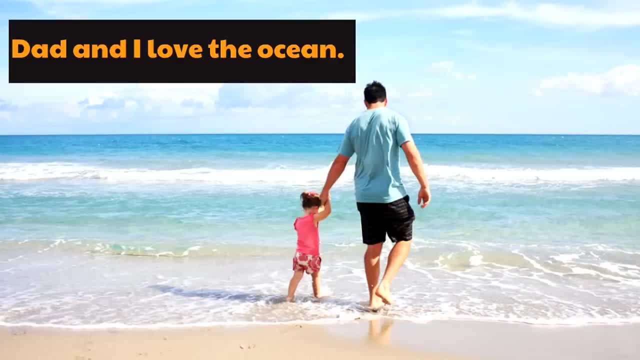 And the word I we know is a pronoun. So we are going to replace This proper noun and this pronoun with one single pronoun, a plural pronoun that will cover both of those nouns. Our new sentence is: we love the ocean. 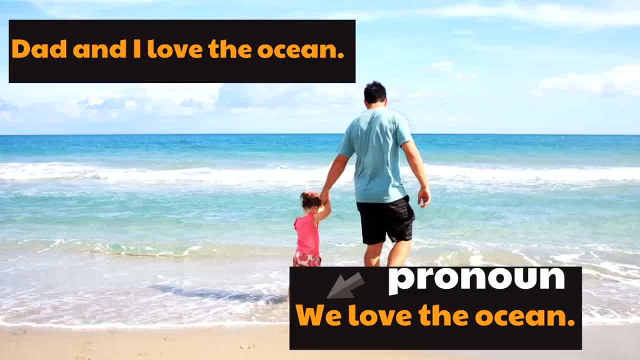 The word we is a pronoun. It's replacing the words dad and I. Dad and I are replaced with the pronoun we. That's a pronoun And notice it's a much shorter and more simple sentence. We love the ocean. 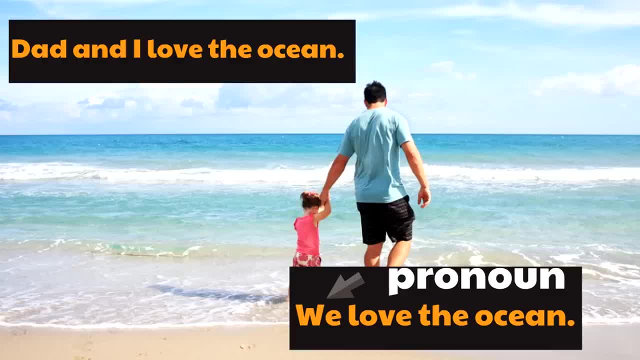 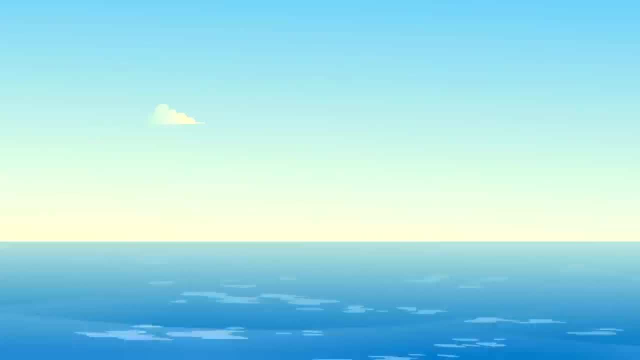 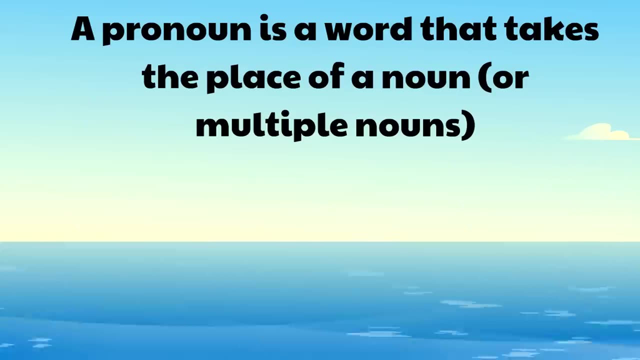 This is the power of pronouns. Pronouns can replace a single noun or they can replace multiple nouns. So to review a pronoun is a word that takes the place of a noun or multiple nouns. Here's a list of some of the more common ones. 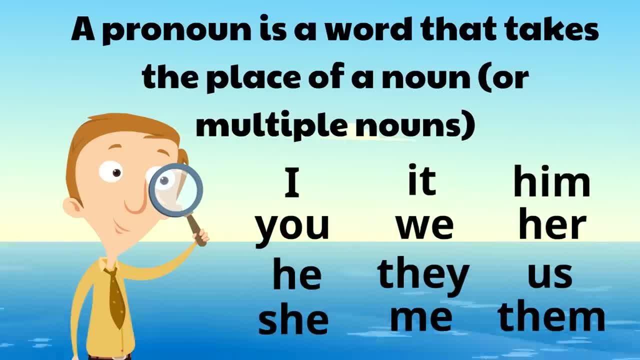 I, you, he, she, it, we, they, me, him, her, us, them. A noun is a person, place or thing, And a pronoun does the same thing. It's a professional word that replaces a noun or multiple nouns in a sentence. 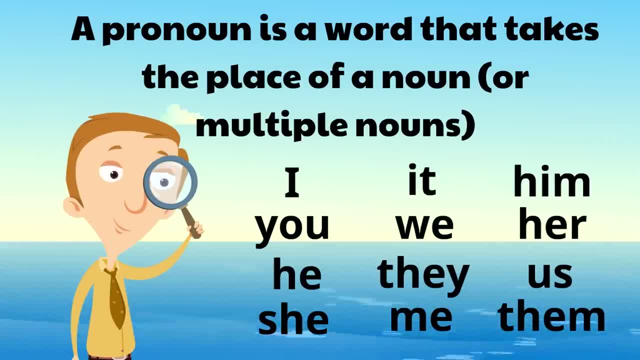 And here they are, And they're so much fun to use: I you, he she it, we, they, me, him, her, us them. The pronouns I you, he she it, we, they me, him, her, us them. 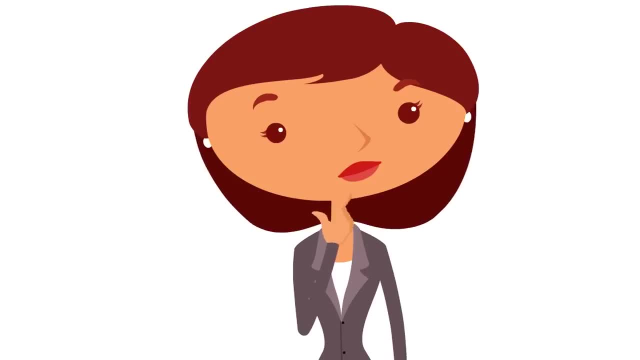 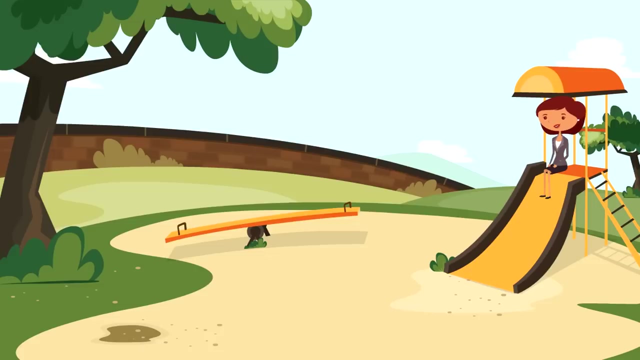 The pronouns. Hey, when is it going to be my turn? I want to be in this compilation video too. Okay, let's see I'm going to teach about rhyming. The park is so much fun. You know what else is fun? 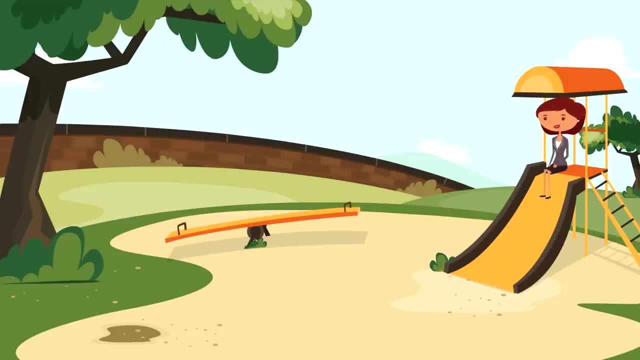 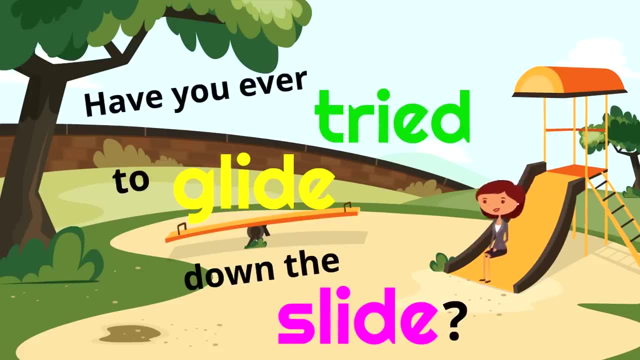 It's using rhyming words while you're at the park like this. Have you ever tried to glide down the slide? It's like a game. I love this. Whee, That was great, And you can practice rhyming anywhere. 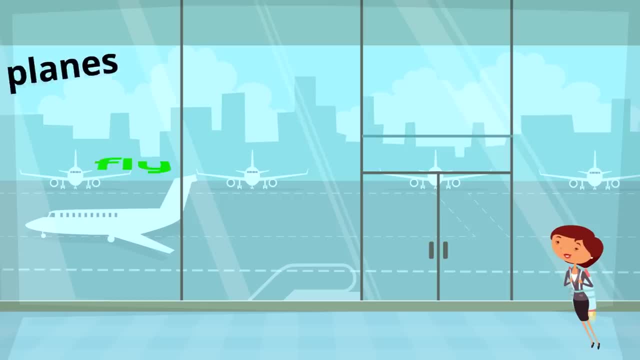 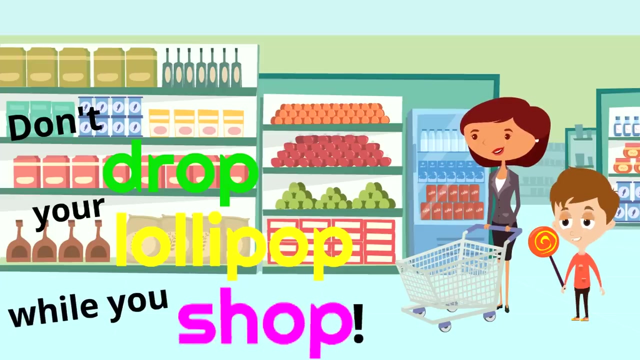 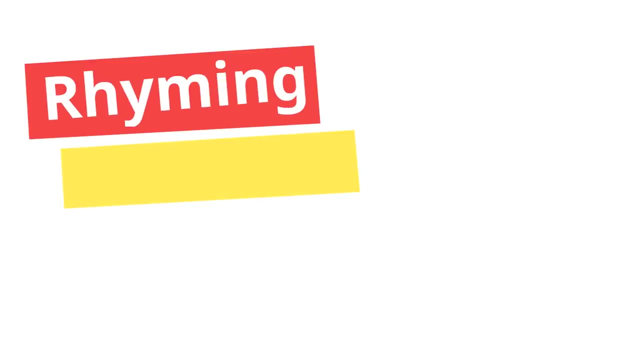 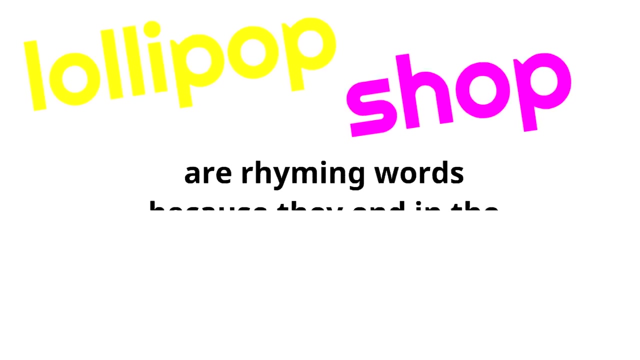 Like at an airport, The planes fly high up in the sky, Whoa. Or at the grocery store, Don't drop your lollipop while you shop. Oh man, Rhyming words are words that end in the same sound. Lollipop and shop are rhyming words because they end in the same sound. 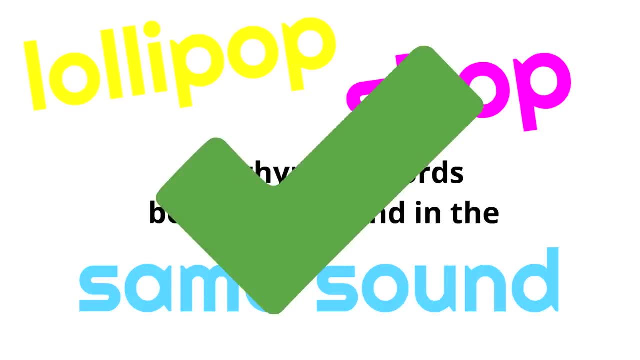 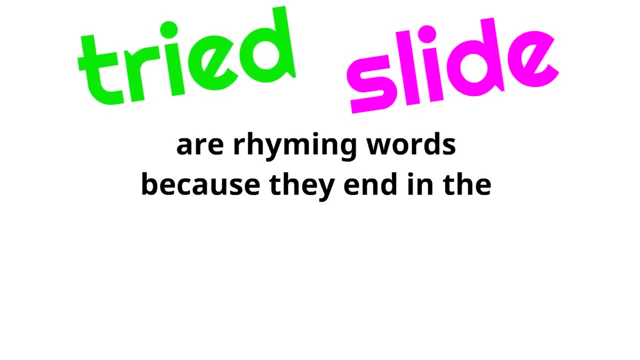 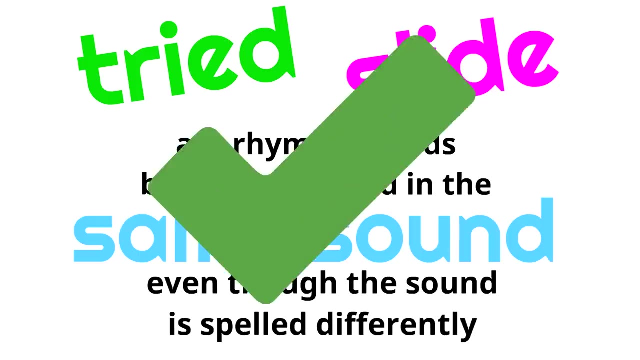 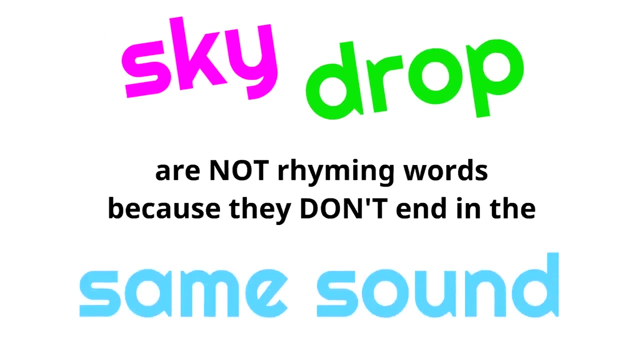 Lollipop shop. Tried and slide are rhyming words because they end in the same sound, even though the sound is spelled differently. Tried, slide, Sky and drop are not rhyming words because they don't end in the same sound. 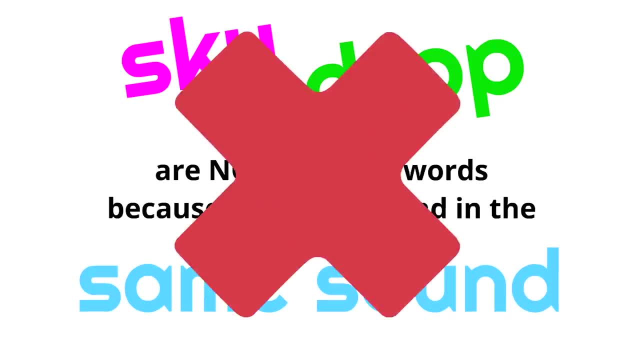 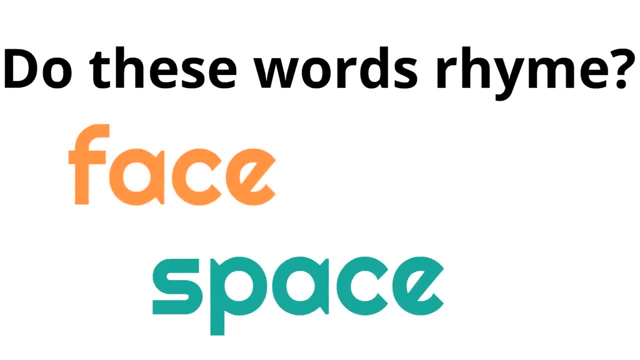 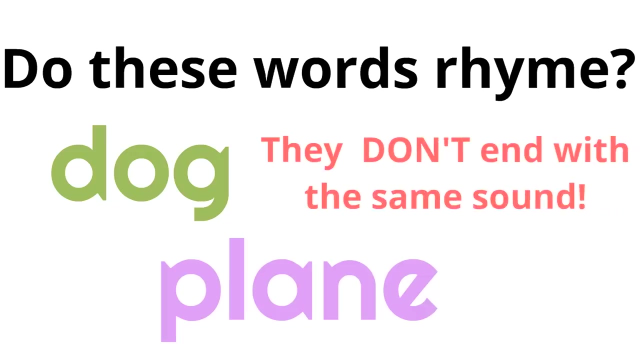 Sky drop. Do these words rhyme Face space- Great job. They rhyme because they end with the same sound. Do these words rhyme Dog plane- Very good, They don't rhyme because they don't end with the same sound. 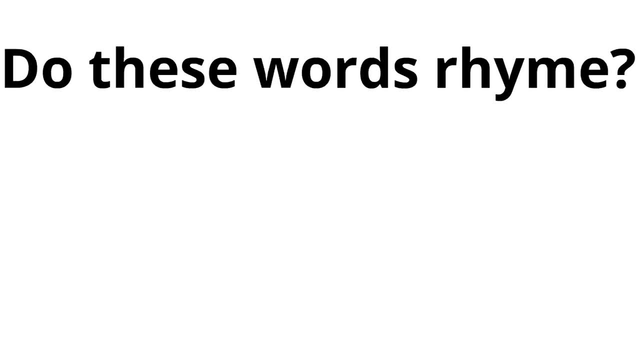 Do these words rhyme? Right, bright, That's it. They rhyme because they end with the same sound, even though the sound is spelled differently. You did great today: You learned that rhyming words are words that end in the same sound. 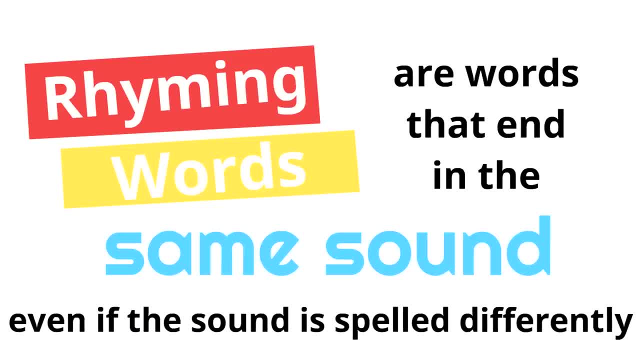 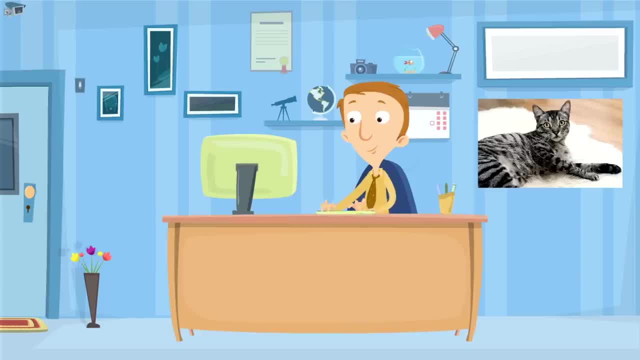 even if the sound is spelled differently. Have fun finding rhyming words. See you next time. We are so happy to have you with us. I mean, you are so awesome, You really are. Oh, you like my poster, Mr Whiskers' poster, you know. 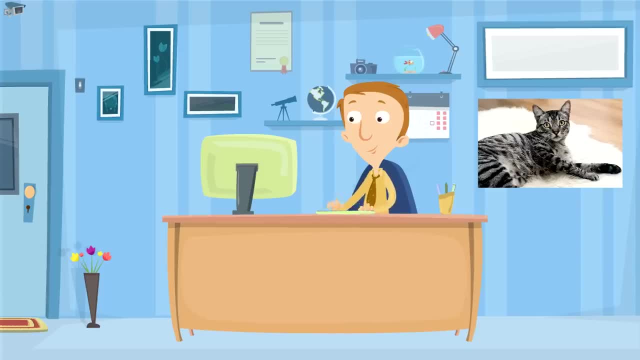 It's pretty cool. pretty cool, you know. It's a pretty cool poster, pretty cool cat too. I wonder what he would like to learn about next If he would learn from one of our videos. what would he like to learn next? 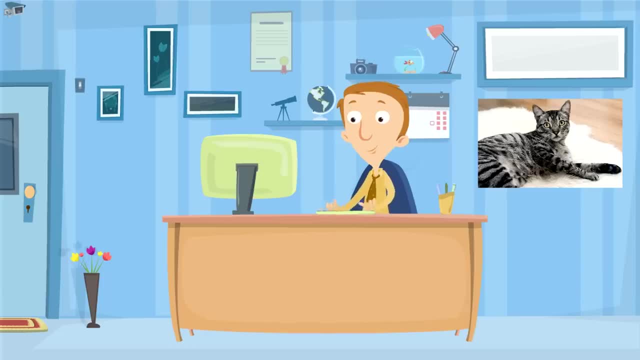 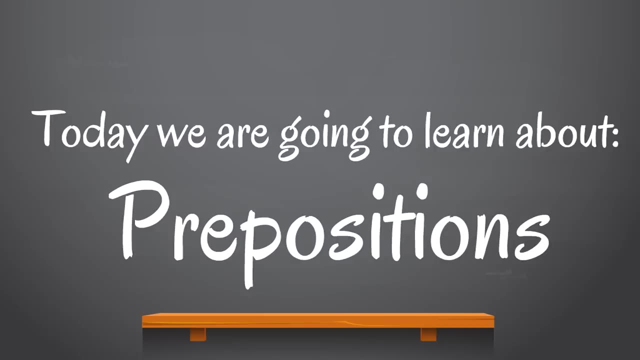 How about Let's learn about Prepositions? Yeah, Wow, What a cool sounding word. What are prepositions? You're about to find out, and then you'll just be able to say Prepositions And you'll know exactly what you're talking about. 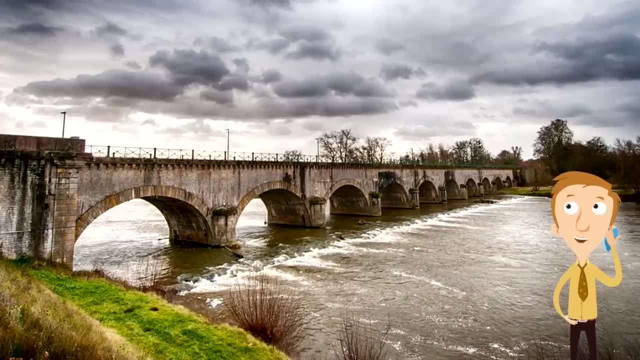 It's going to be cool. First, we want to show you this. Okay, you might be saying: Why are you showing us a bridge? Well, there's a good reason for that. There's a very good reason for that. We're going to just keep that a secret for now. 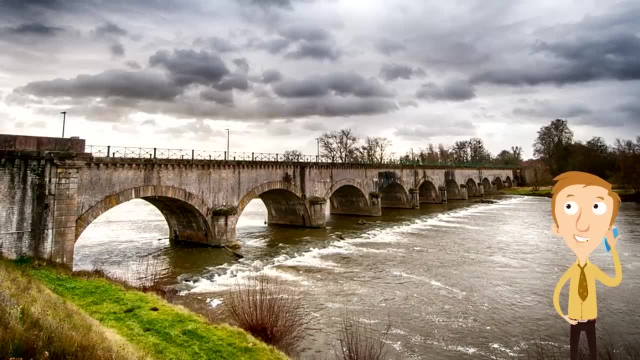 But for now, just look at this picture of a bridge. Bridges are so cool, aren't they? They're so cool. They're structures that connect two sides of things, don't they? And you can see the storm clouds are coming. 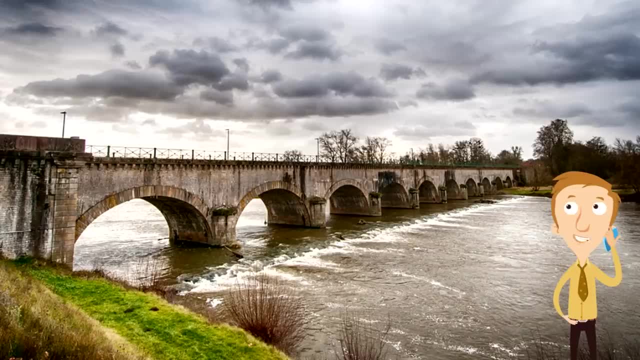 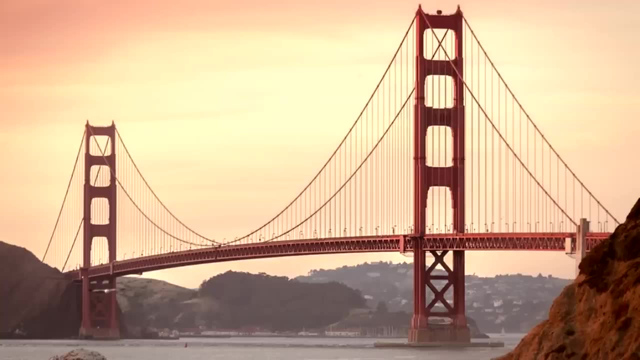 It's probably going to start raining. You know, the photographer probably was running for cover, You know, but this is a nice picture of a bridge. Here's another picture of a bridge. Do you know the name of this bridge? Pretty famous. 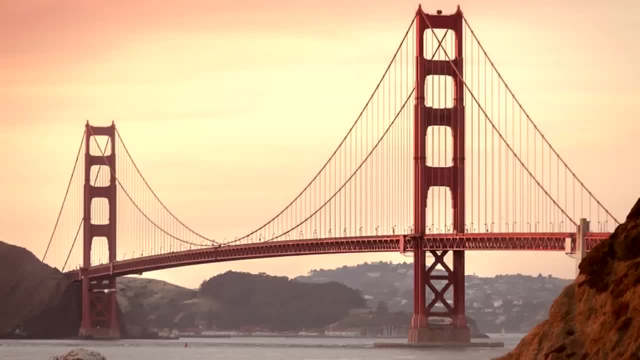 Pretty famous bridge. Okay, Yeah, the Golden Gate Bridge. Okay, the Golden Gate Bridge. If you didn't know that, you need to check out our video on the Golden Gate Bridge. Some fascinating facts there. You're going to love it. 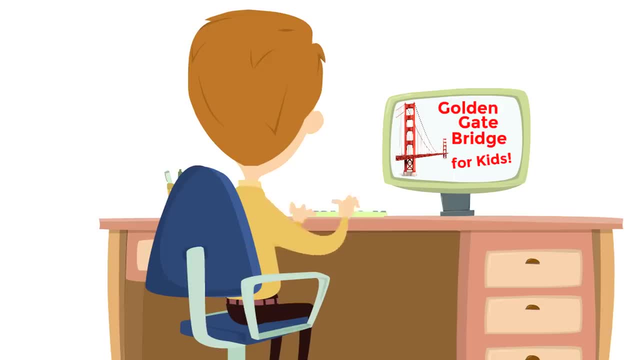 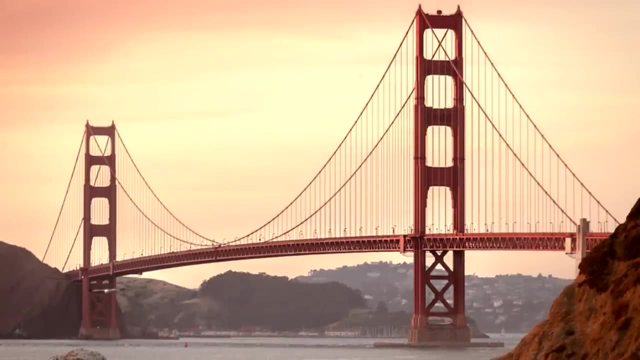 You're going to love sharing those with your friends and your family, And everyone's going to be like what? Let's look at the Golden Gate Bridge again. It's an amazing bridge, And a bridge connects two sides- A bridge. You might be wondering. what does this have to do with prepositions? 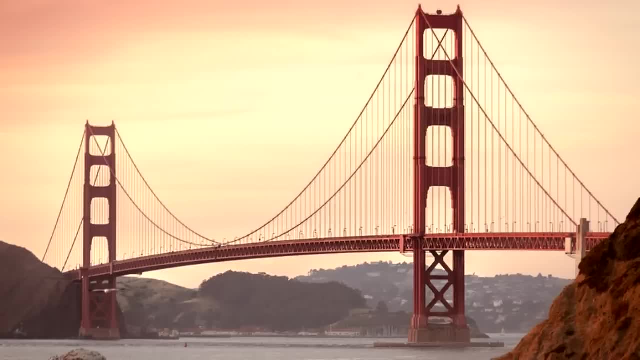 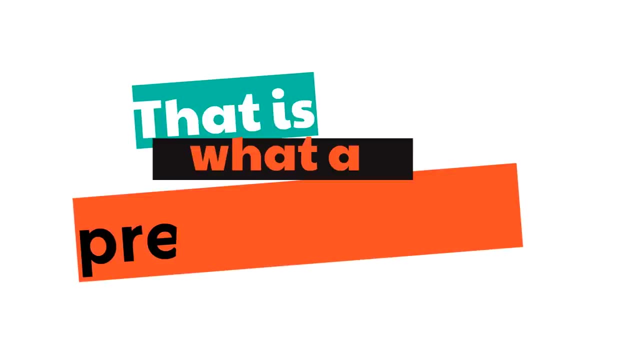 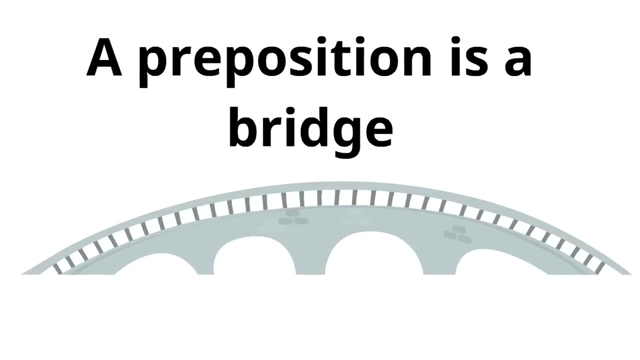 I thought we were talking about prepositions, not bridges. What is going on here? Well, That is what. a preposition is Okay, A bridge. A preposition is a bridge. Okay, In the world of words and grammar, it's not really a bridge. 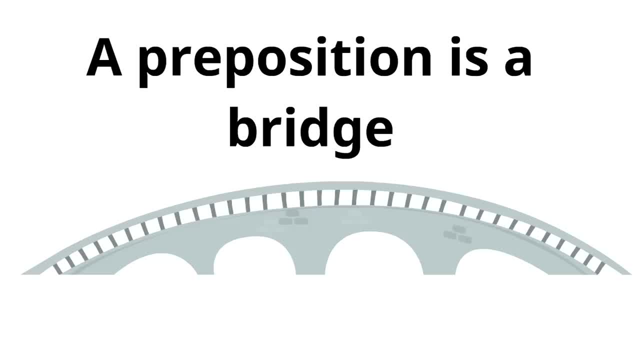 You can't drive a car on a preposition. Okay, That would be a little bit difficult And you wouldn't be able to do it. But a preposition works just like a bridge in the world of words. A preposition is a bridge. 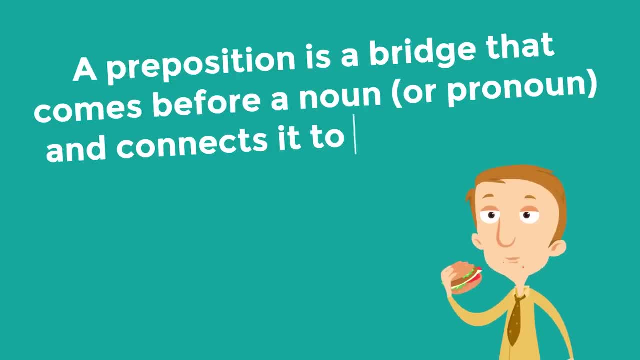 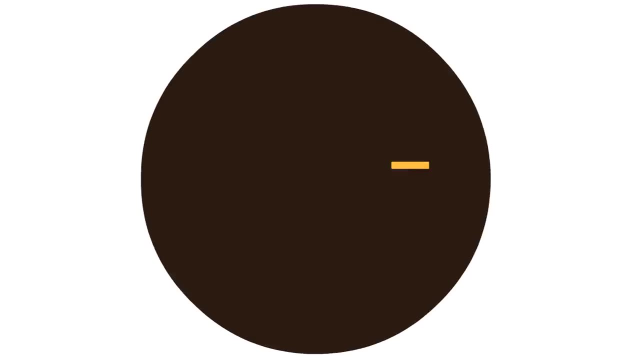 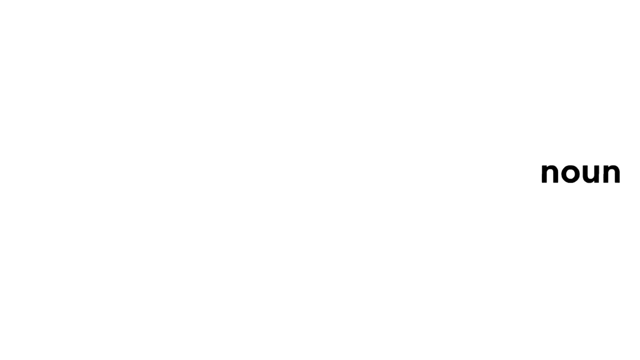 A preposition is a bridge that comes before a noun or pronoun and connects it to the rest of the sentence, And this is how it works. For example, let's say we've got a noun at the end here and then we've got the rest of the sentence. 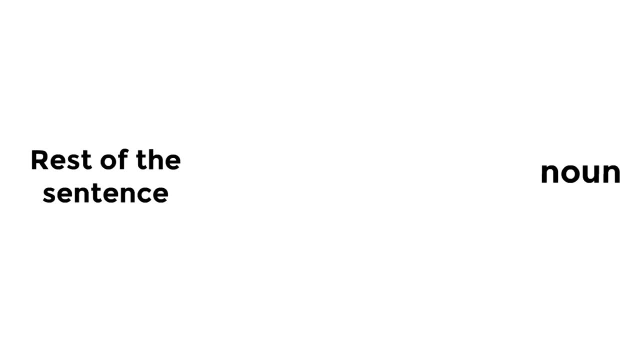 Now we've got a problem. There's a big gap. Something's got to go in between. Now, let's say, the part with the noun is my backpack And the rest of the sentence is: I put my book. I put my book. 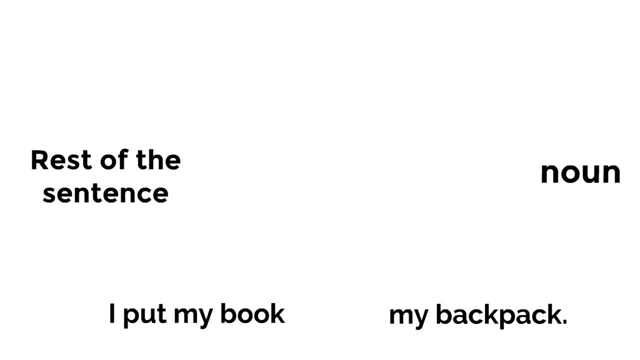 My backpack. There's a gap. It's a lonely backpack. We need a connecting word, We need a bridge. So we put in a preposition- Yeah, A preposition, A bridge word, A connecting word that will connect the noun at the end to the rest of the sentence. 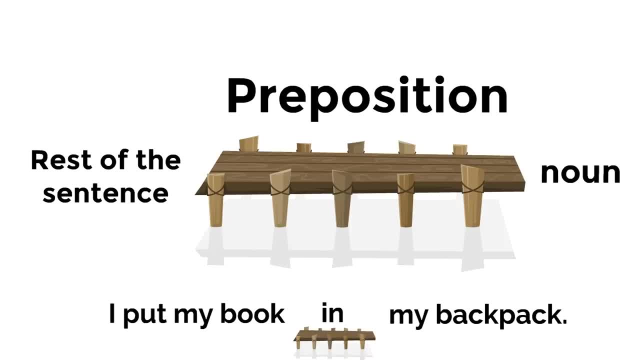 So we're going to use the preposition in. So it would read like this: I put my book in my backpack. Now the noun backpack is connected to the rest of the sentence. Yay, Yay, bridge, Yay prepositions. 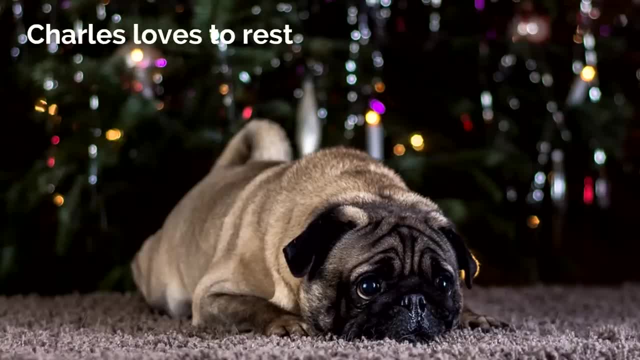 Let's look at this example. Charles loves to rest the floor. Uh-oh, there's a gap. We're going to need a bridge, We're going to need a preposition to connect floor to the rest of the sentence, aren't we? 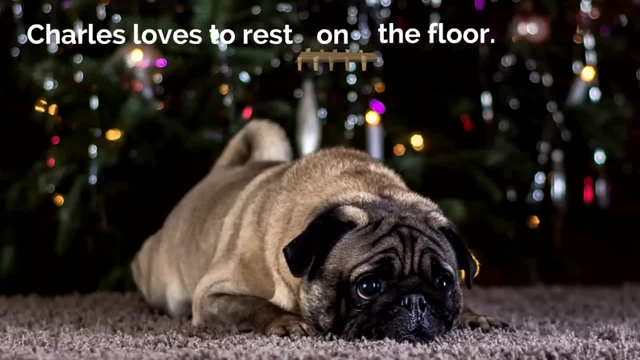 Let's try the preposition on. Charles loves to rest on the floor. Oh, it's perfect. On is connecting floor to the rest of the sentence. Charles loves to rest on the floor- Wow, that's perfect. That's perfect. 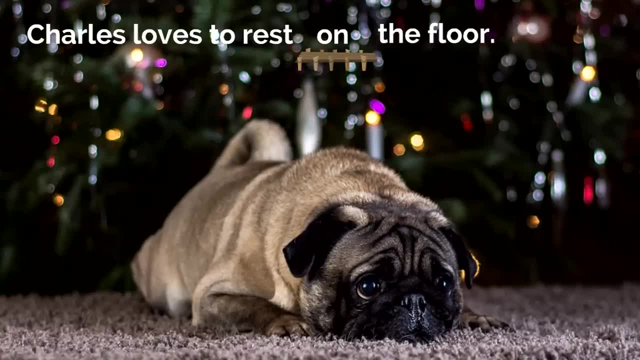 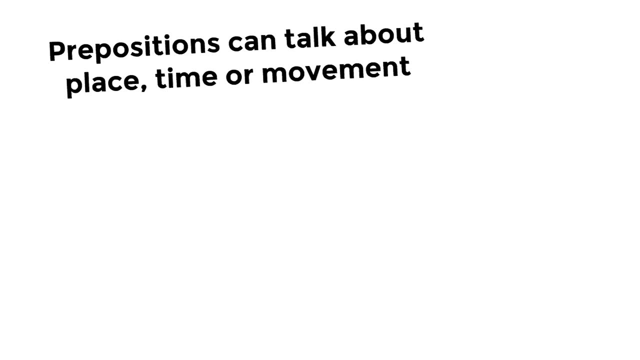 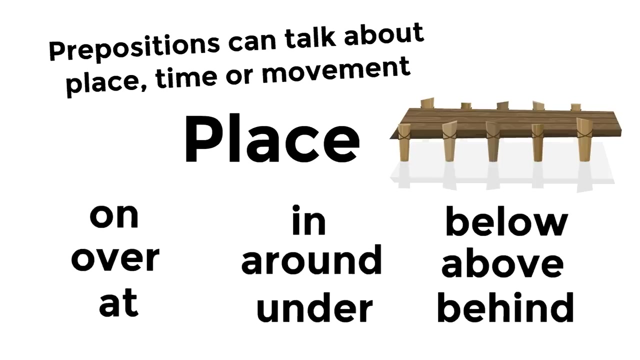 I love prepositions. Prepositions can talk about place, time or movement. Here's some examples of prepositions that talk about place, On, over, at, in, around, under, by, Under, below, above, behind. 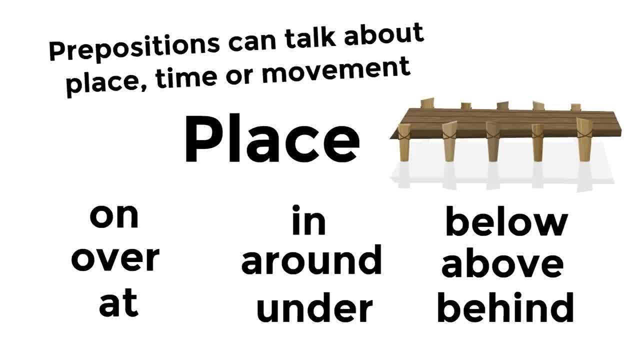 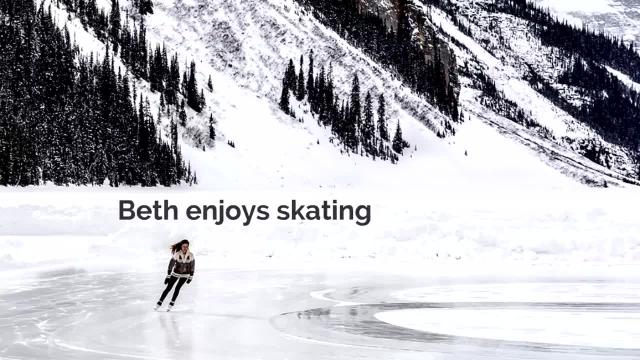 These are all prepositions that talk about place or placement. Isn't that interesting? Let's look at this example: Beth enjoys skating the lake. Uh-oh, there's a gap. We need a preposition. We're going to need a preposition that talks about place. 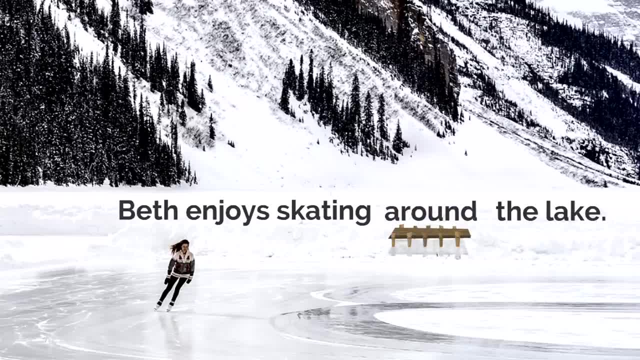 Let's try around. Beth enjoys skating around the lake. Oh, that's the perfect preposition for that. It connects lake to the rest of the sentence. Beth enjoys skating around the lake Prepositions. We said this already. They're pretty cool. 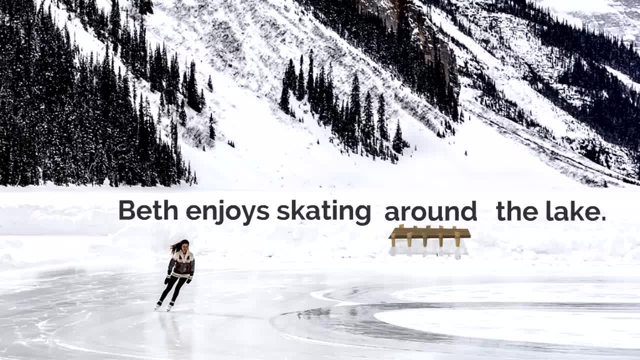 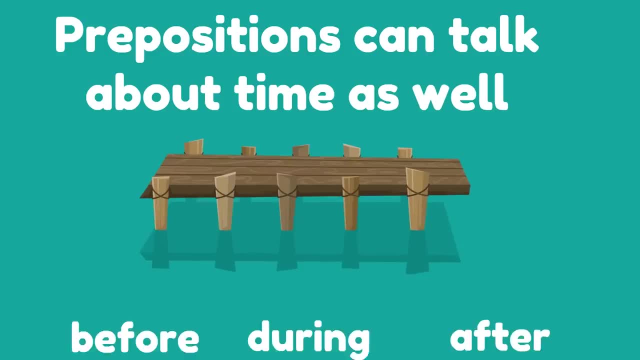 They're pretty awesome, Pretty amazing. All right, You got to connect. We need the connecting words, We need the bridges, We need prepositions. Now, prepositions can talk about time as well. Look at these prepositions: Before, during, after. 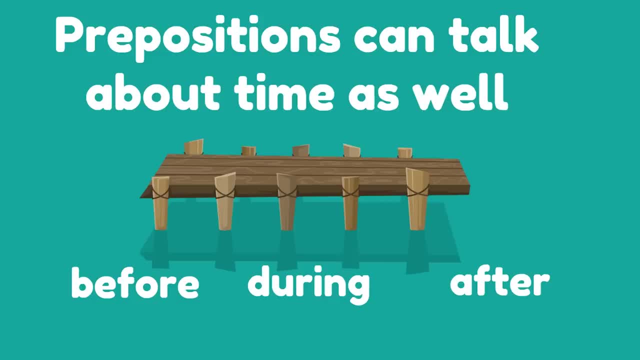 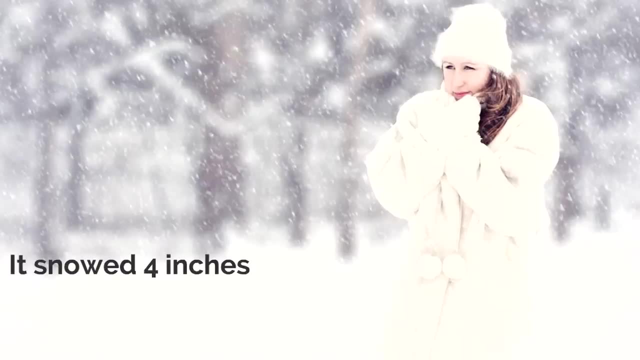 These are prepositions. These are bridge words, connecting words. They're prepositions that talk about time. Look at this example: It snowed four inches the day. Oh, we're definitely going to need a preposition there, aren't we? 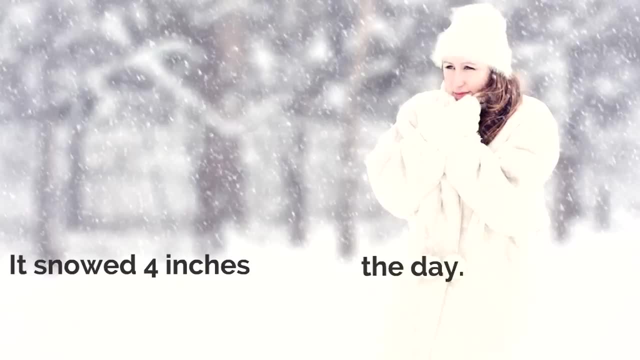 Oh, my goodness, What's a preposition we could use for this sentence. Let's try the preposition during, During. So our sentence would read: it snowed four inches during the day. Wow, that's perfect. That's the perfect bridge word. 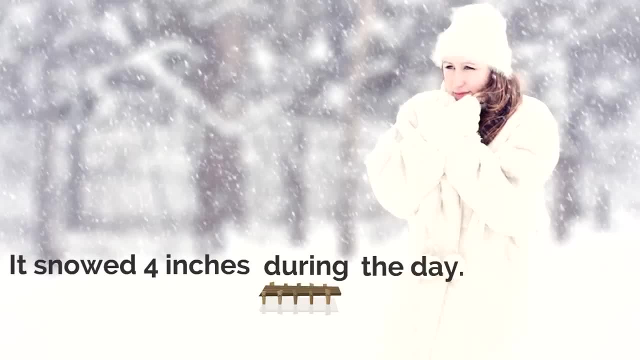 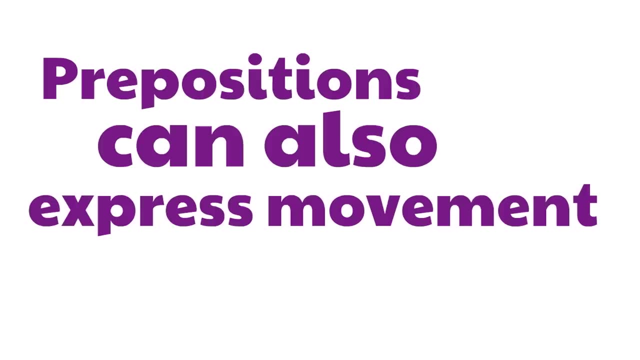 The perfect connecting word, The perfect preposition. Now, prepositions can also express movement. Whoa, Like these prepositions: Through, towards, to Into, across, along. These are prepositions, bridge words, connecting words that express movement. 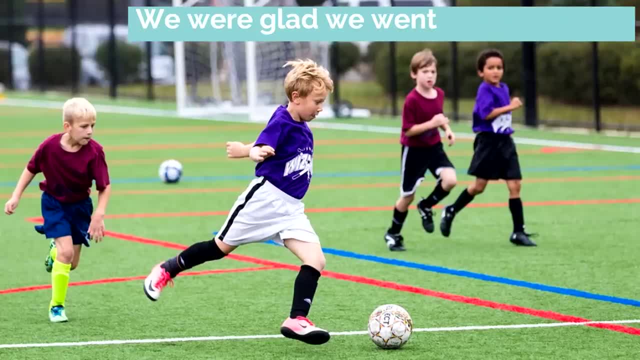 Let's try this one. We were glad we went the game. Uh-oh, We're definitely going to need a preposition. We have to connect game to the rest of the sentence. Let's try to. We were glad we went to the game. 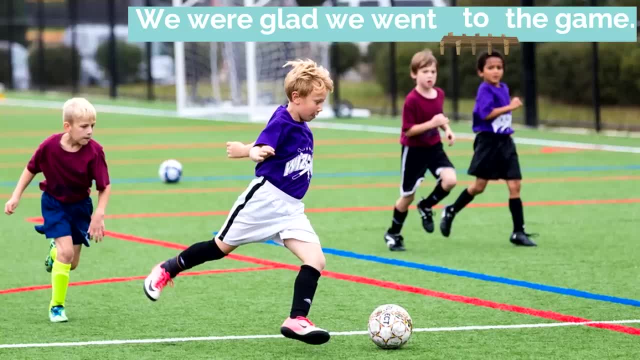 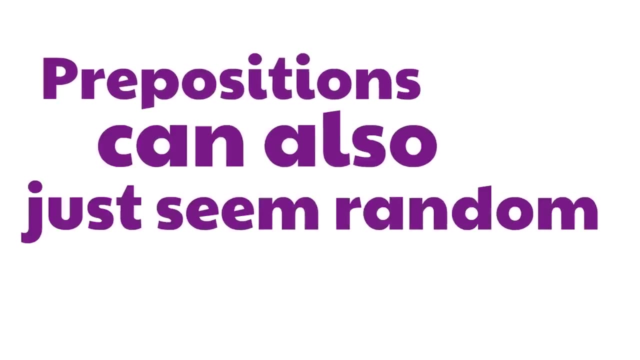 To is one of the prepositions that express movement. We were glad we went to the game And now the word game is connected to the rest of the sentence. Prepositions can also just seem random, Like about, of and from. 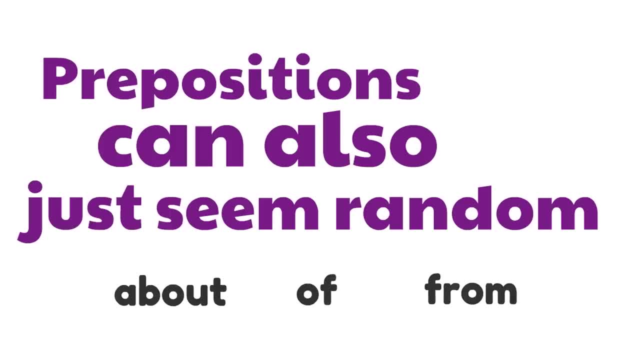 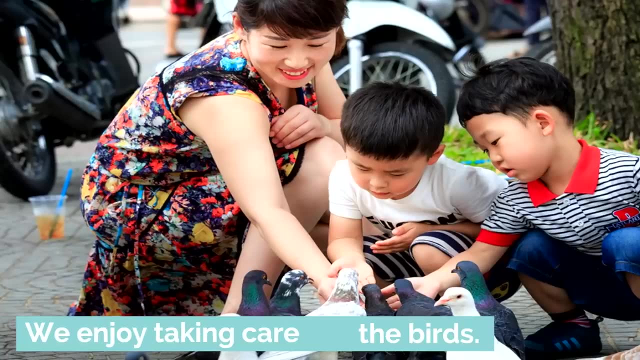 You can just memorize these words as prepositions, because they do kind of seem random. About. of and from are all prepositions too. Here's our next sentence: We enjoy taking care the birds. Uh-oh, There's a gap. 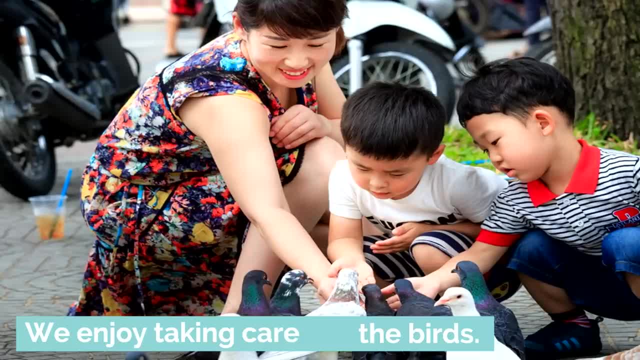 We're going to need to fill that with a bridge word, a preposition, aren't we? What is a preposition that you think would go well there? Which one do you think fits in that like a puzzle? We enjoy taking care the birds. 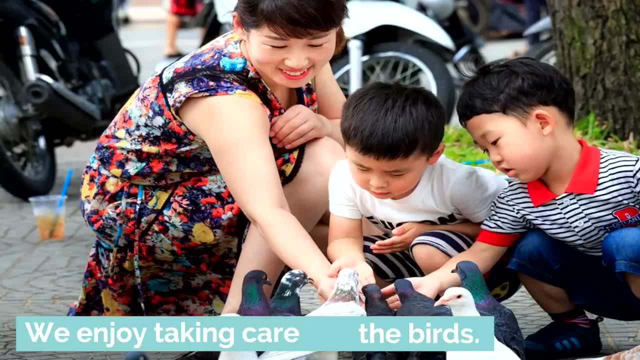 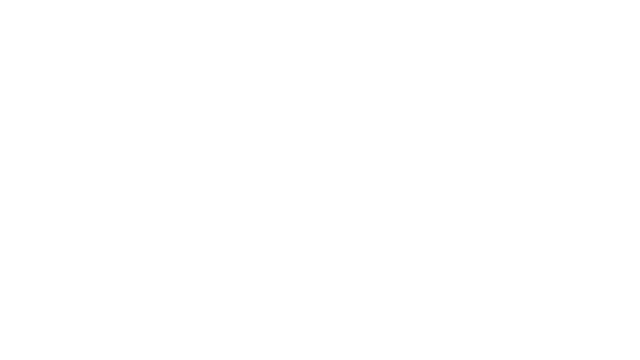 Yeah, of of We enjoy taking care of the birds. Of is a preposition. It's a bridge word connecting birds with the rest of the sentence. Now here's something that can be tricky: Prepositions can also appear at the beginning of a sentence. 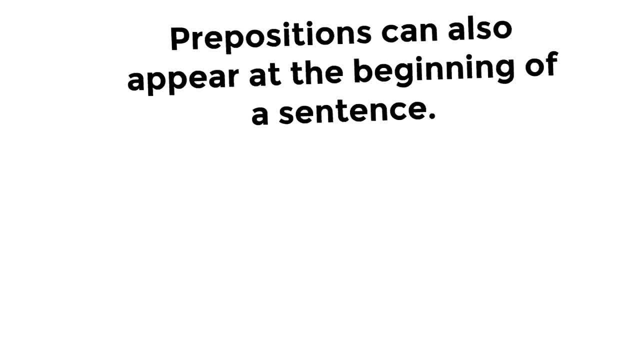 The preposition still has a noun coming after it, and then there's the rest of the sentence, But the preposition is still connecting the noun to the rest of the sentence. Let's show you With an example. All right, Here we go. 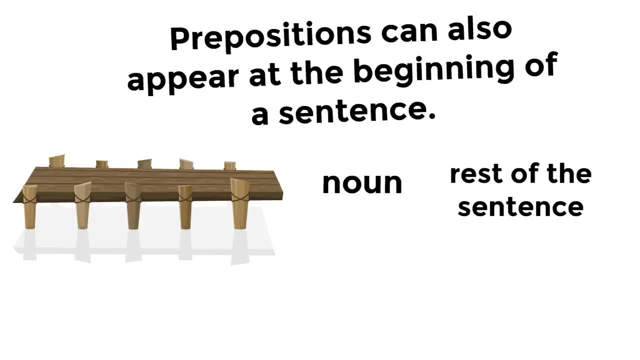 Prepositions can also appear at the beginning of a sentence, For example: All right, Here we go After dinner. Ooh, After is a preposition. After dinner, I enjoy reading a book. Wow, Now notice, it's still a bridge word and it's still connecting dinner. that's the noun. 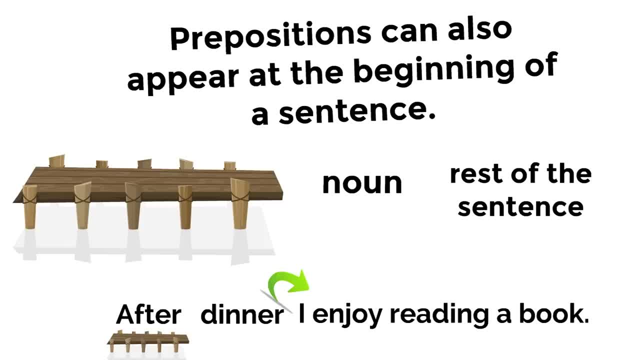 to the rest of the sentence. even though it appears at the beginning, It's still a bridge word, still a connecting word. So if you see a preposition at the beginning of a sentence, don't freak out, It's okay. 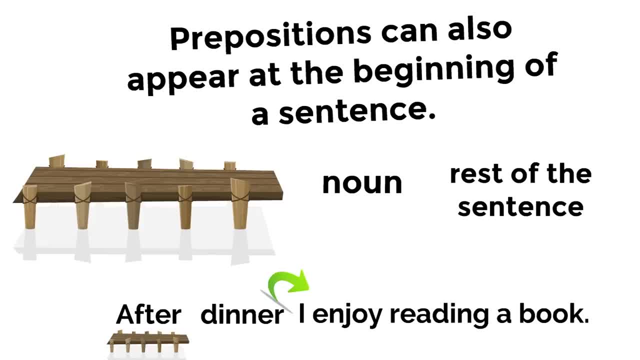 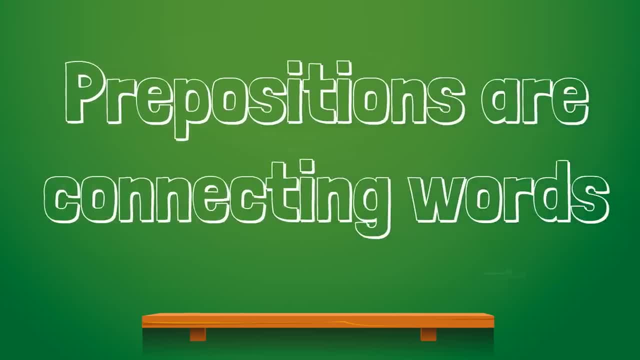 Sometimes they go there. Prepositions are connecting words And, wow, just like bridges. they're a great time, They're awesome And they just they're just cool. They're just cool. Who else is a fan of prepositions? 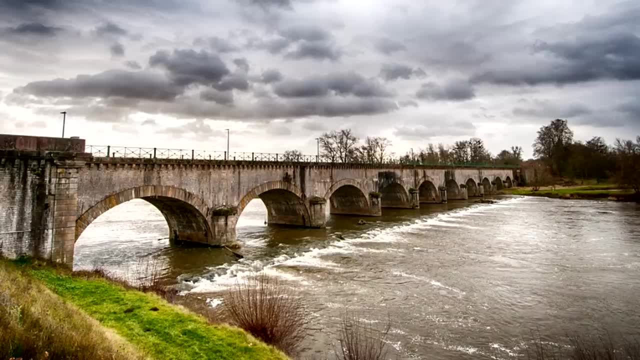 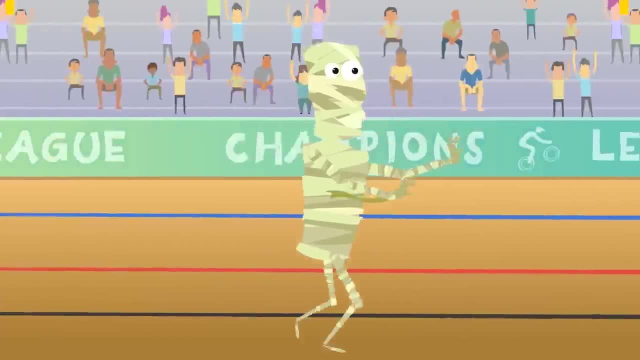 Anybody, Anybody, No one. You like prepositions? now, right, You love them. right, You love prepositions. They're connecting words, They're bridge words. Wow, You're doing such a great job in your race. 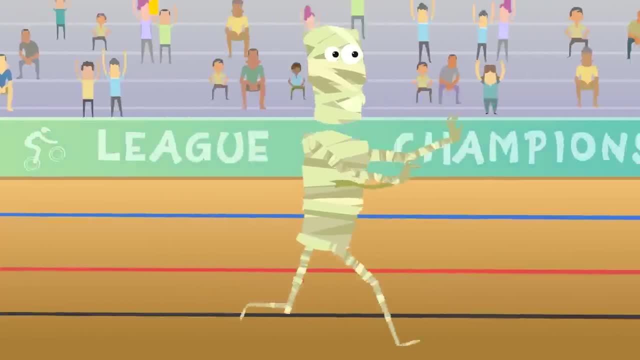 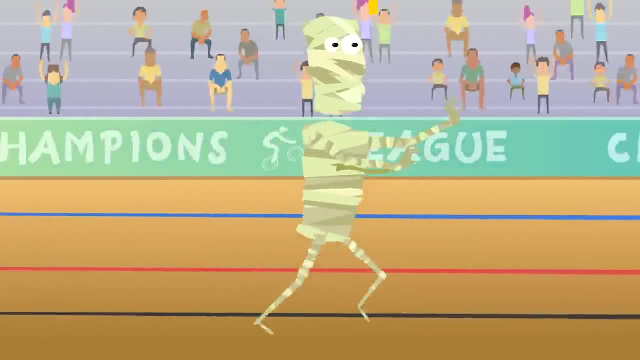 I had no idea you were an athlete. okay, I mean, with all that cloth wrapped around you, you're doing great. You're doing a great job, Just like these kids are doing a great job learning, In fact. how about this? 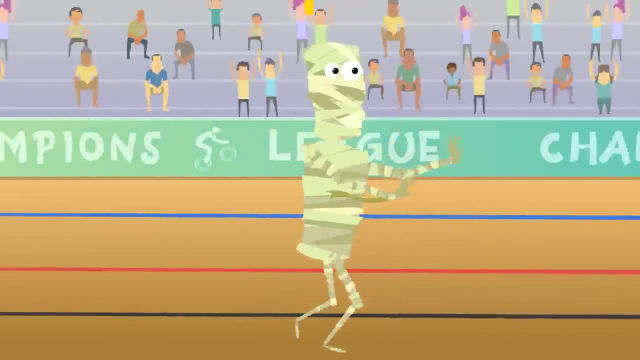 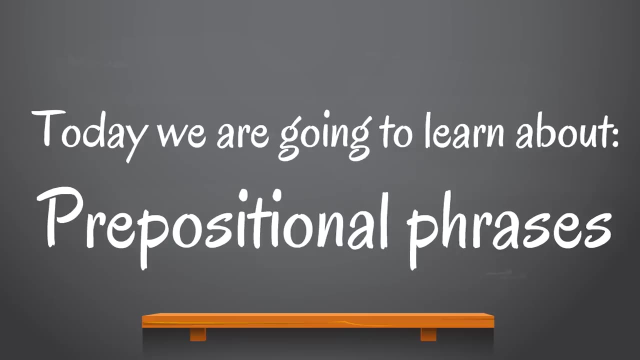 The next thing we're going to learn about is prepositional phrases. Do you know what those are? Prepositional phrases? You're about to understand them. They are very cool. They are very, very cool. Prepositional phrases are incredible. 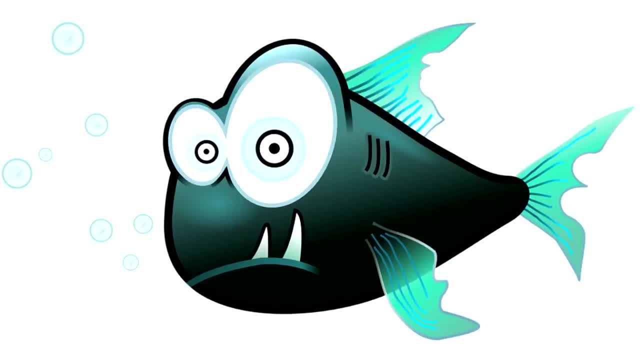 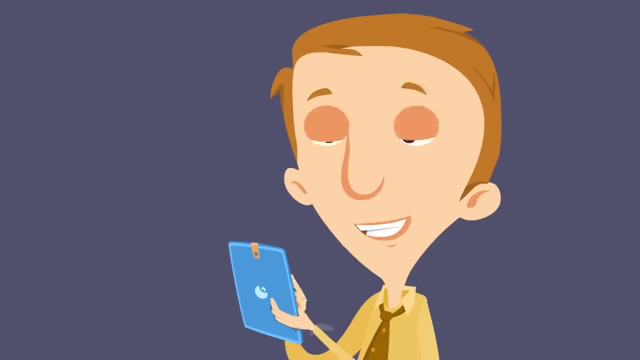 Once you know them, everyone's going to be like what You know what that is And you'll be like yep, yep, prepositional phrases. I got it. I watched the video Before we learn that we have to answer this question. 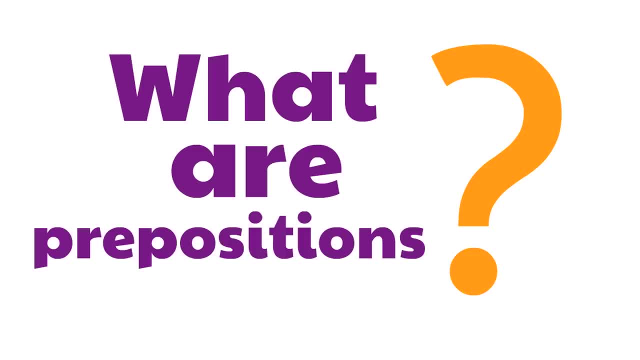 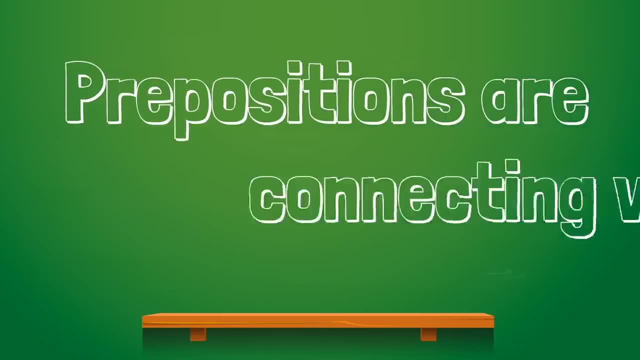 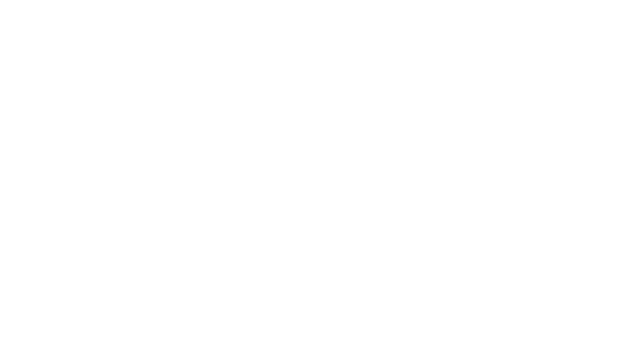 What are prepositions? We can't know what a prepositional phrase is without knowing what prepositions are. Well, prepositions are connecting words. It's pretty simple: They're connecting words. Prepositions are connecting words that act like bridges. 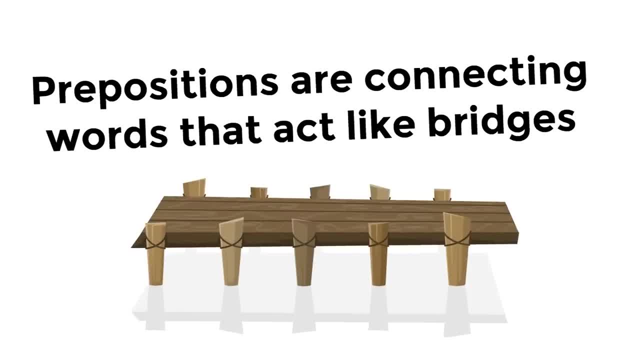 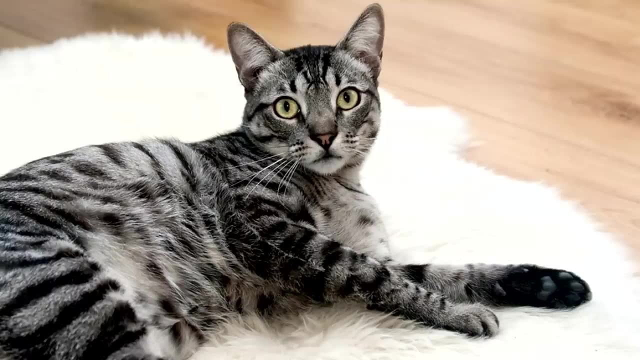 Like this bridge- Whoa, Wow, What a cool bridge, A wooden bridge. A bridge connects from one side to the next And in a similar way, prepositions are connecting words. They're like bridges in the word kingdom, Mr Whiskers. 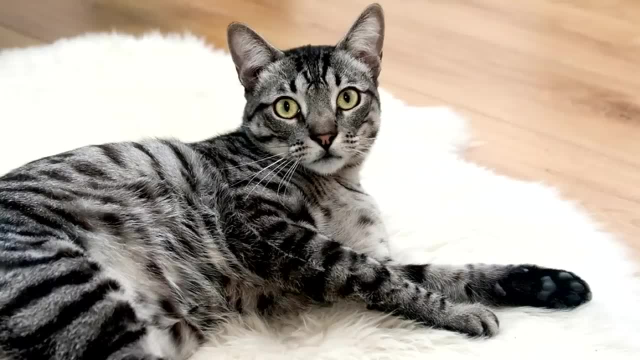 Oh, What are you doing up right now? You're supposed to be sleeping. You're supposed to stay up during the night and sleep during the day. I don't know what's going on with your internal clock. We're in the middle of talking about prepositions- how prepositions are like bridges. 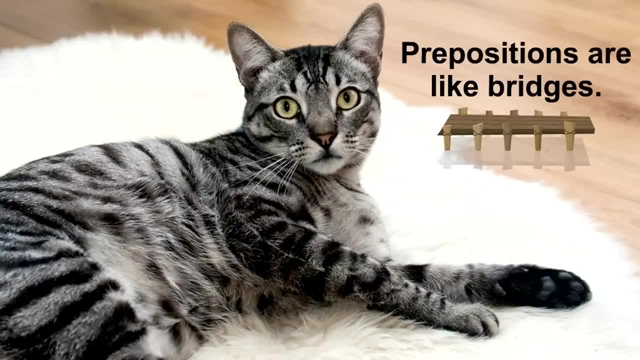 They're like the bridges of the word kingdom: They connect, They're connecting words, They're great words, And I'm in the middle of a review. Listen, If you'll just hold up, Play with a special bouncy ball, Okay. 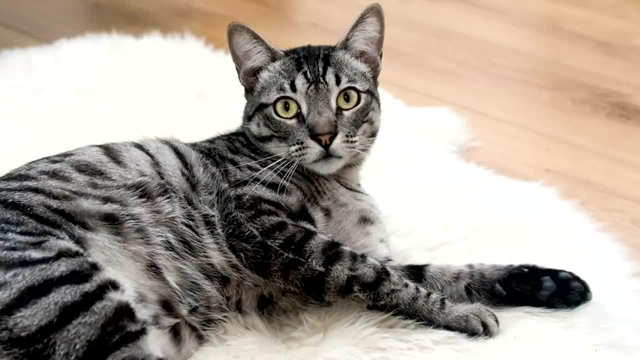 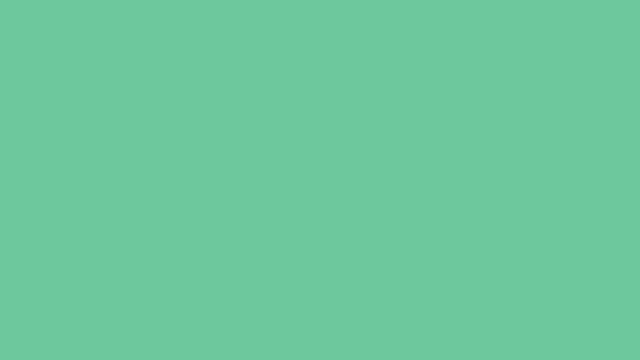 And the little thing with the string, You know, And the little feather, You know, You'll think you're attacking a bird. Okay, Can you just wait just a moment? So prepositions are like bridges that connect a noun to the rest of the sentence. 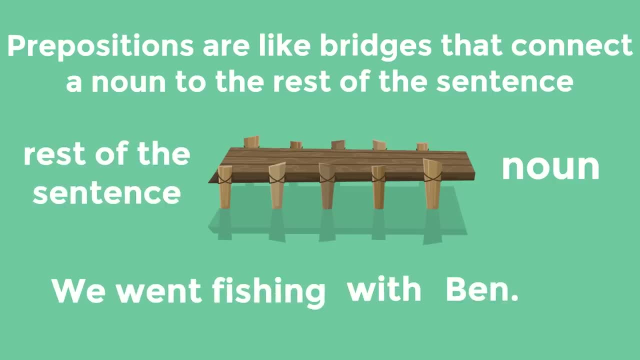 For example, we went fishing with Ben. With is the preposition, Because it's connecting Ben to the rest of the sentence. We went fishing with Ben. It's connecting Ben with the idea of going fishing. We went fishing with Ben With is a connecting word. 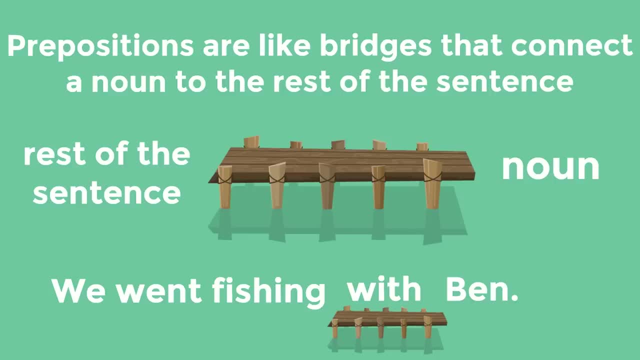 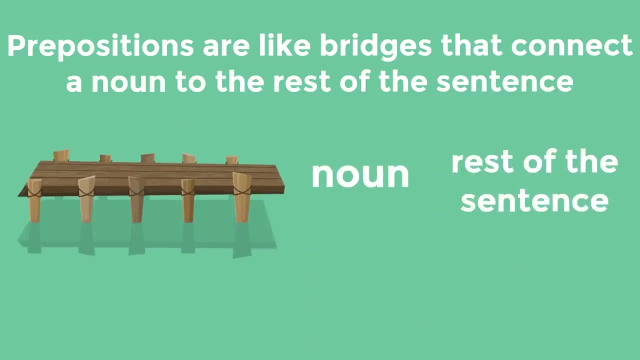 A bridge. The word with is a preposition. Now, sometimes a preposition is at the beginning of a sentence, but it still comes before a noun, connecting that noun to the rest of the sentence. Okay, Look at this example. After dinner, she read a book. The word after is a preposition. It's connecting the word dinner, the noun, to the rest of the sentence. She read a book. After dinner, she read a book. 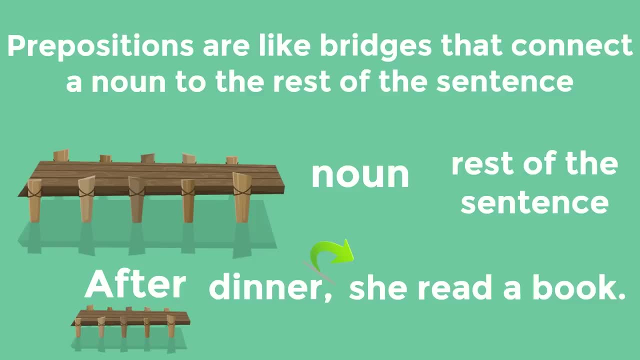 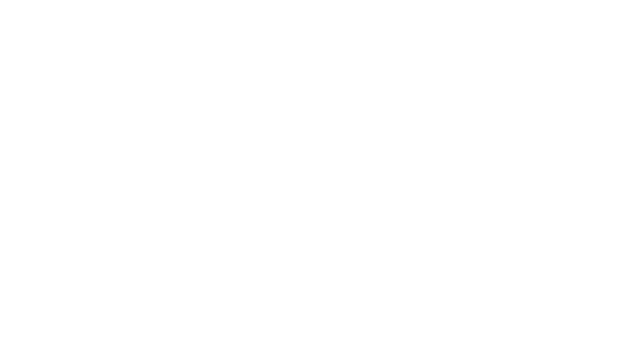 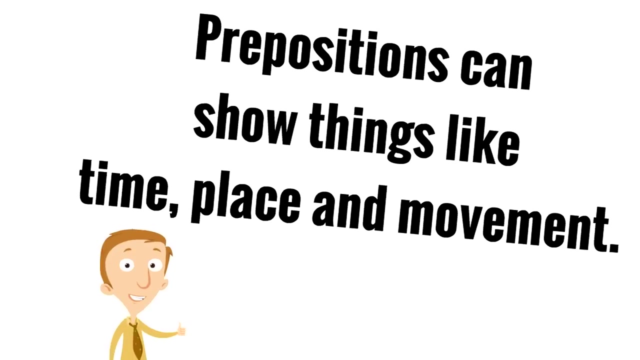 It's still a connecting word, It's still a bridge word, It's a preposition, even though it's at the beginning of the sentence. Prepositions can show things like time, place and movement. Cool Yeah, they're really interesting words that can do a whole lot. 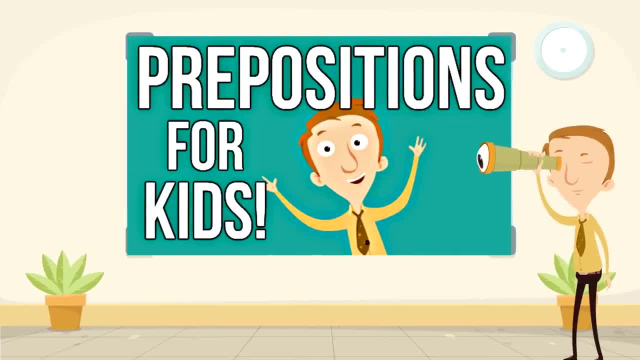 If you want to learn more about prepositions, we have a video that's pretty cool that talks about prepositions in more detail. After this video, you'll see a button that you can click to go straight to this video and we'll share more about the different types of prepositions and things like that. 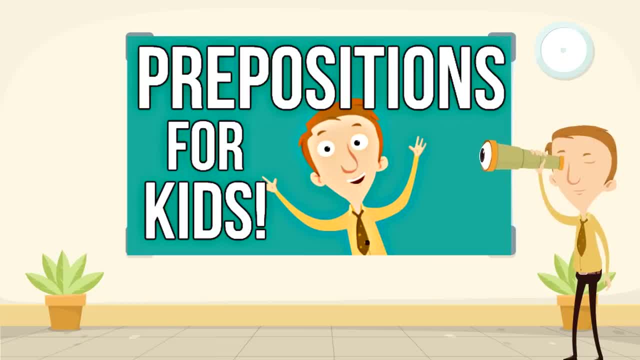 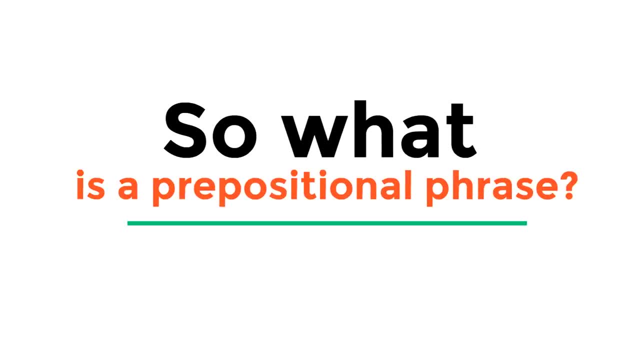 But for now? Now, what you need to know is: prepositions are connecting words. Okay, so what is a prepositional phrase? We know that a preposition is a bridge word, a connecting word, but what is a prepositional phrase? 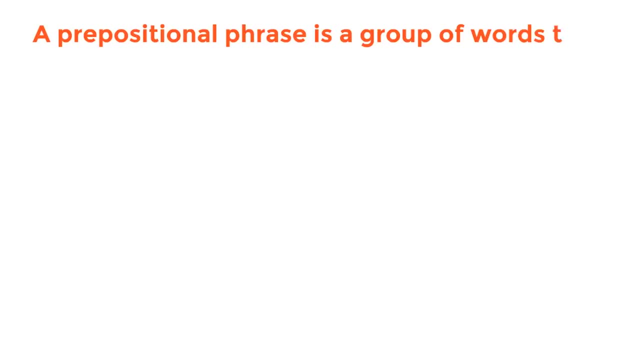 Well, a prepositional phrase is a group of words that begins with the preposition and ends with something called the object of the preposition. Now, when we think of prepositions, we think about the prepositional article. Remember the sentence from earlier? 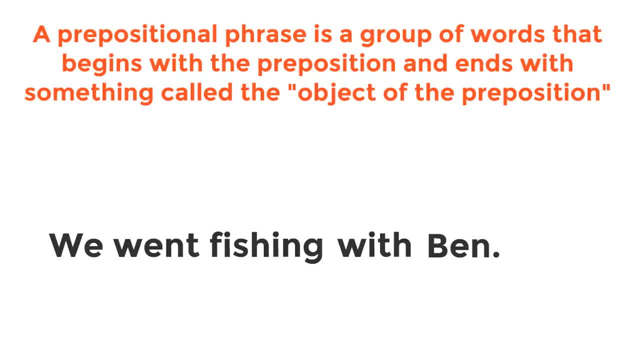 We went fishing with Ben. We went fishing with Ben, Remember. the word with is the preposition because it's connecting the noun, which is the word Ben, to the rest of the sentence. But we went fishing with Ben. 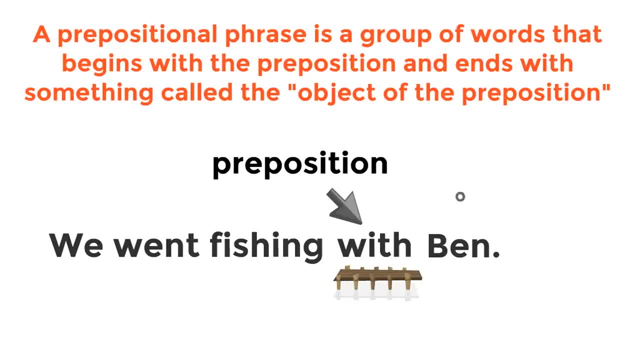 Now, this is so cool. Do you see this noun that comes after the preposition, This word Ben? Do you see this noun that comes after the preposition, This word Ben? This is called the object of the preposition. 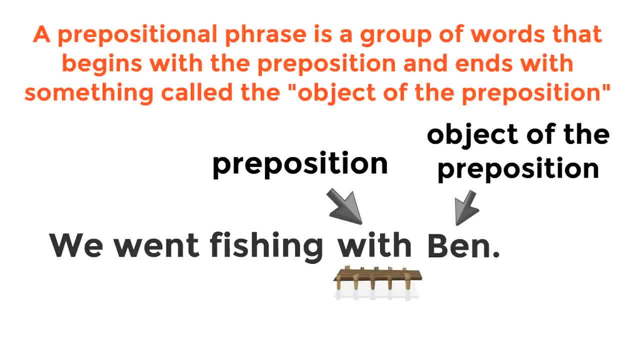 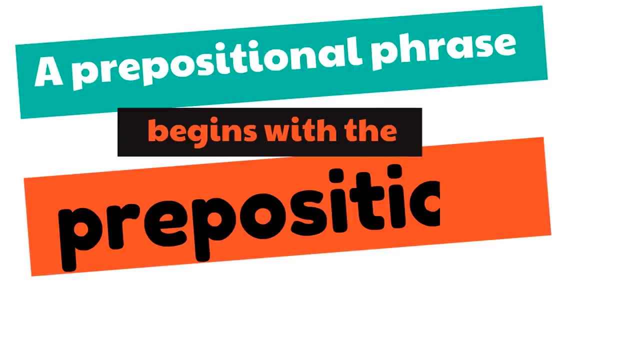 The noun that follows the preposition is always called the object of the preposition. Now remember: a prepositional phrase begins with the preposition and ends with the object of the preposition. So in our sentence the prepositional phrase is with Ben. 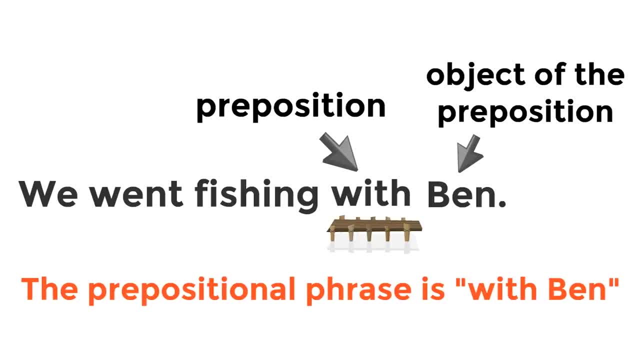 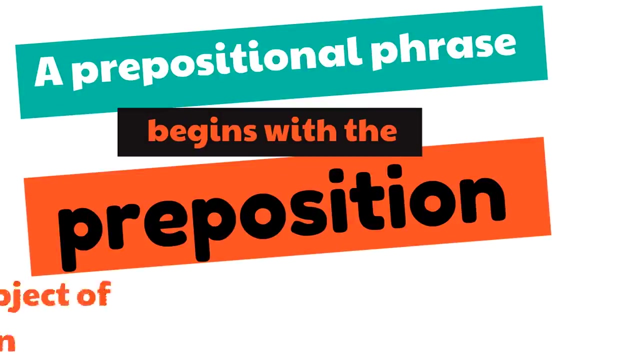 With Ben. with is the preposition, so it starts the phrase and the object of the preposition ends the phrase. So the prepositional phrase only has how many words? Yeah, two words. The prepositional phrase is with Ben. Remember, a prepositional phrase begins with the preposition and ends with the object of the preposition. 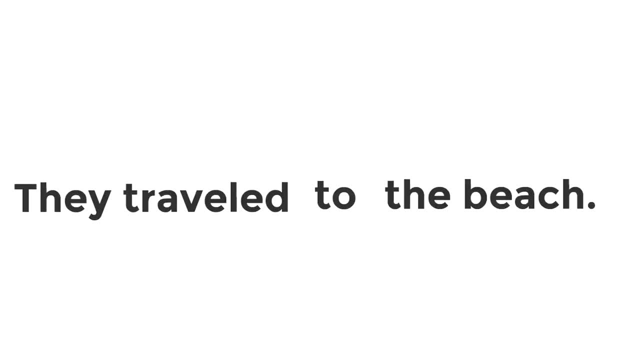 Okay, let's give this one a try. They traveled to the beach. They traveled to the beach. Well, the word to is the preposition here It's the connecting word, that's connecting beach to the rest of the sentence. They traveled. 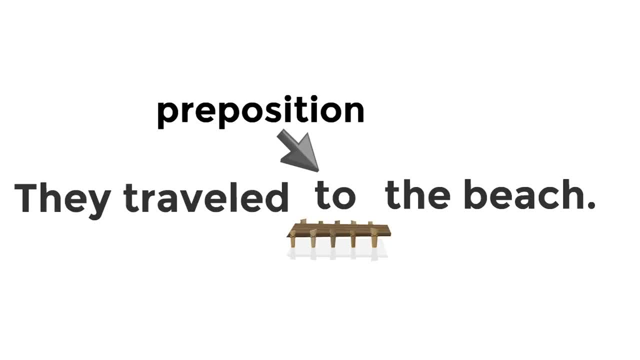 Okay, which word is the object of the preposition? Yeah, just say the word Uh-huh. Yeah, beach. Beach is the object of the preposition. It's the noun that is following the preposition. That means the prepositional phrase is to the beach. 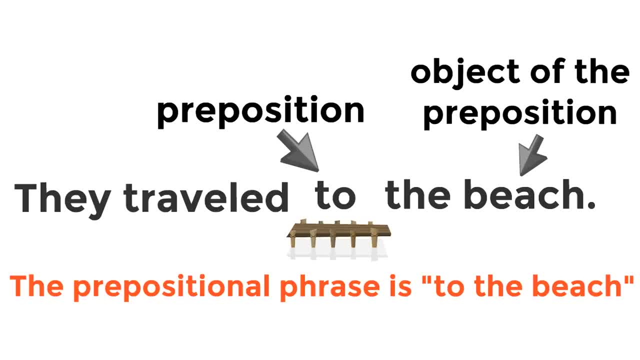 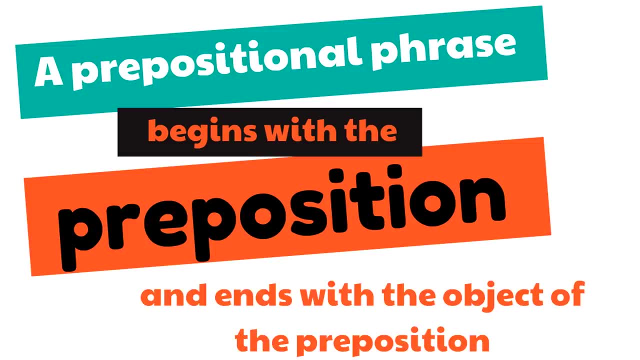 There are three words in this prepositional phrase. Remember, a prepositional phrase begins with the preposition and ends with the object of the preposition. It's the noun that is following the preposition and ends with the object of the preposition. 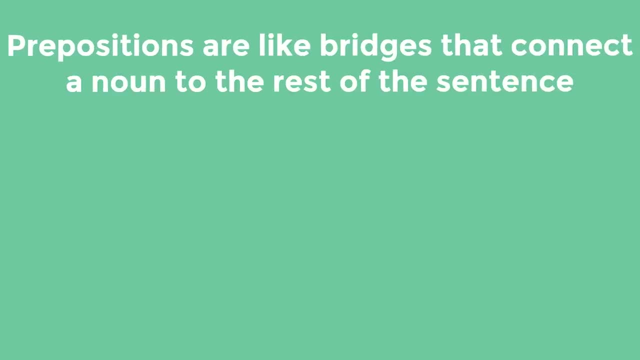 Prepositions are like bridges that connect a noun to the rest of the sentence. Sometimes a preposition appears at the beginning of a sentence, followed by the object of the preposition, which is just the noun that follows the preposition, and then the rest of the sentence. 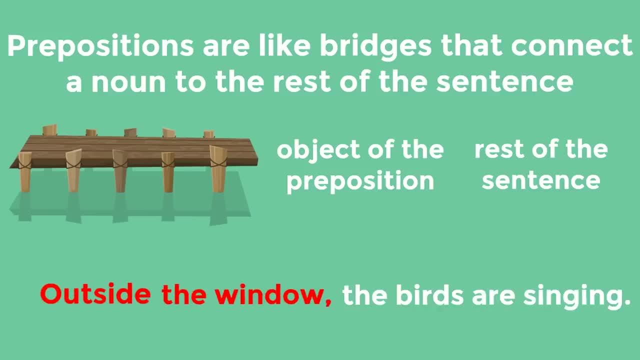 Look at this sentence: Outside the window, the birds are singing. Outside the window is the prepositional phrase. The word outside starts the phrase out because it is the preposition And the word window is the object of the preposition. ending the prepositional phrase. 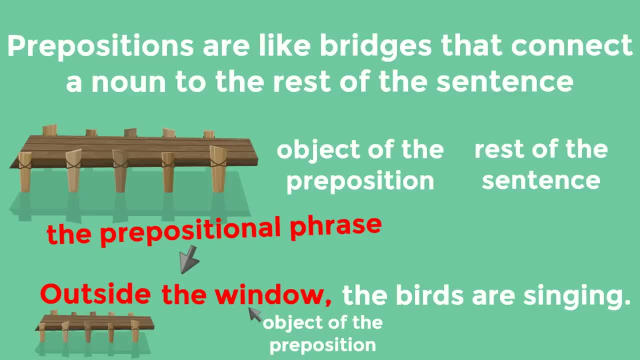 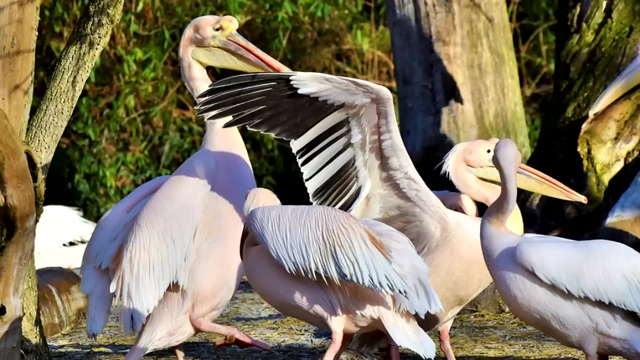 Pretty simple. Wouldn't it be funny if the birds outside the window singing were these? I mean, oh my goodness, pelicans are awesome and they actually don't sing, They just make sounds like. And if you don't believe me, listen. 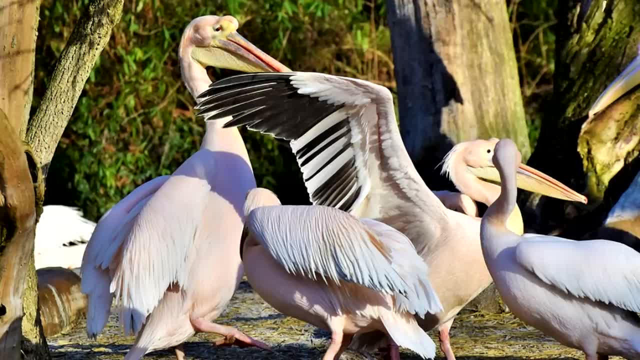 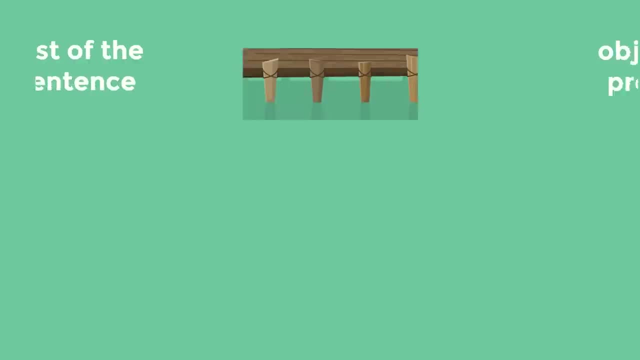 Look it up. Look it up online. alright, Listen to the sounds they make. Let's get back to prepositional phrases. We're going to give one final example, and in this one the preposition is more in the middle of the sentence instead of at the beginning. 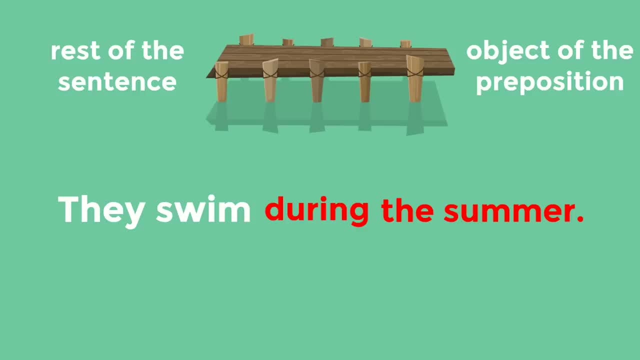 They swim during the summer. They swim during the summer. During the summer is the prepositional phrase, During is the preposition. so it starts the prepositional phrase, And summer is the object of the preposition, ending the prepositional phrase. 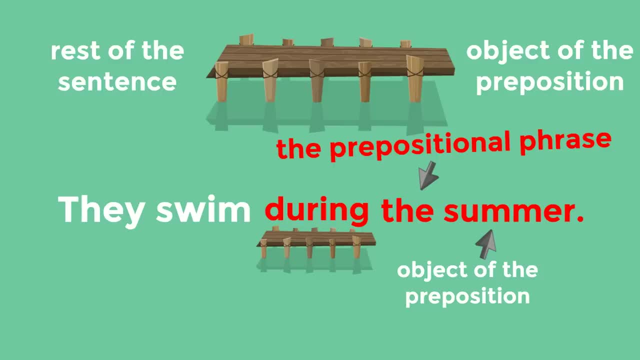 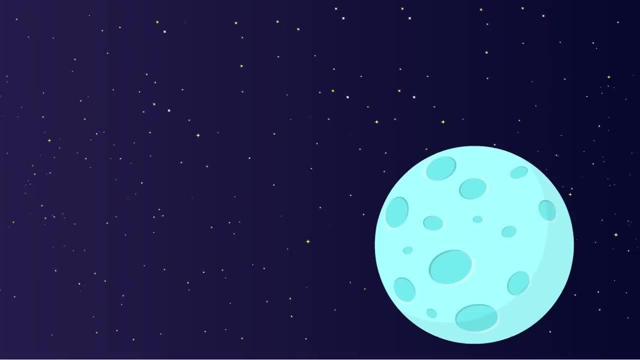 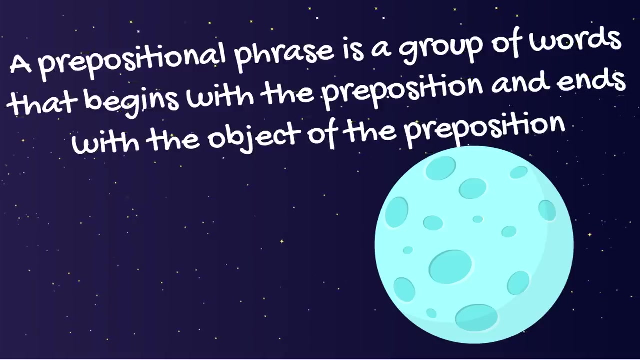 So the prepositional phrase has three words. During the summer, Okay, we're in space. Well, a prepositional phrase is a group of words that begins with the preposition and ends with the object of the preposition. Wow, there you go. 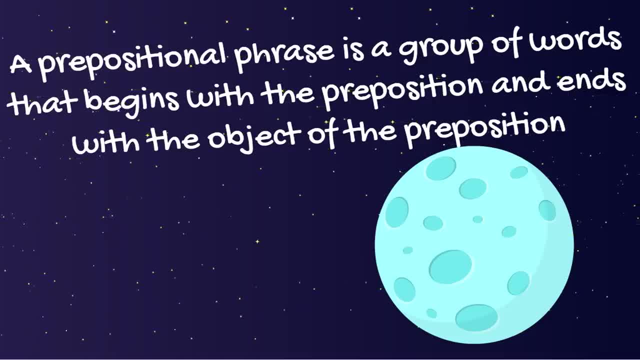 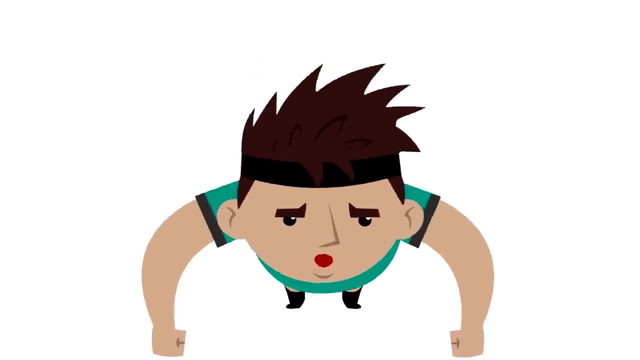 A prepositional phrase. Now you know what that means. You have been doing a great job, just like Mike who's doing these push-ups. You know he knows it's important to stay fit and to exercise and to stay healthy. 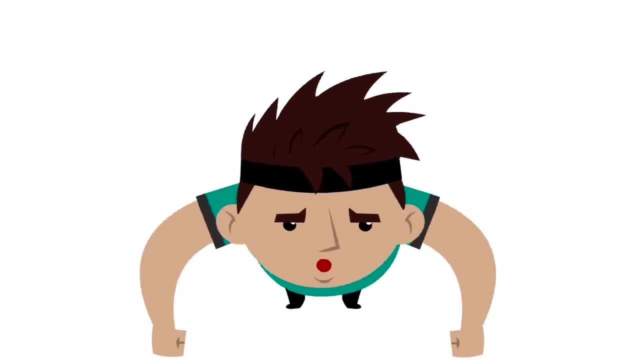 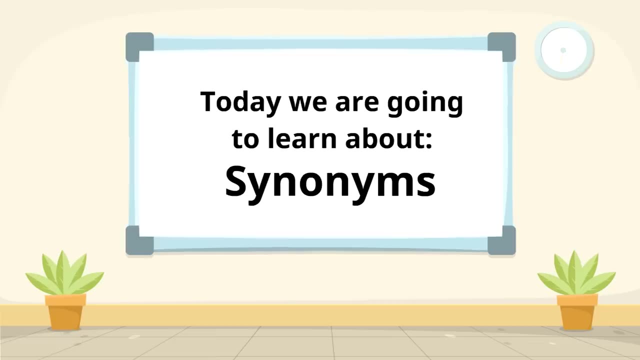 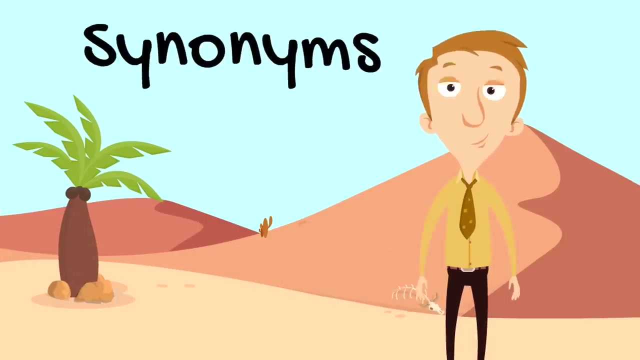 And you're like exercising your mind right now, which is super cool. And next we are going to learn about Synonyms. We're going to learn what synonyms are and how you can spot them. So what are synonyms? Well, synonyms are words with the same meaning or almost the same meaning. 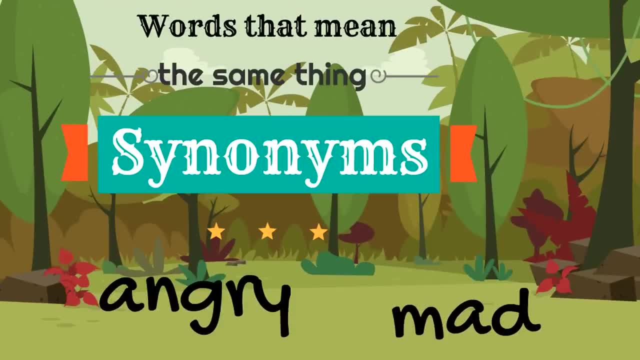 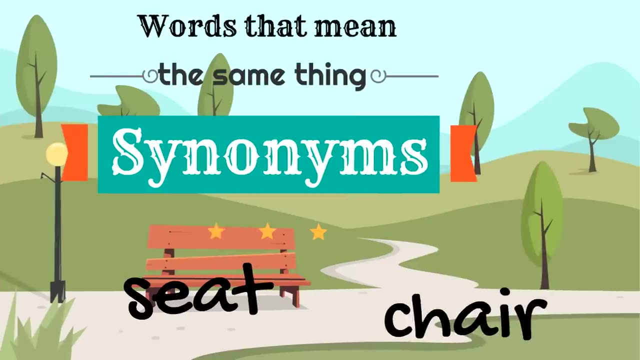 Words that mean the same thing are synonyms, like the words angry and mad, Angry and mad, Angry and mad and mad have the same meaning. They are synonyms. Words that have the same meaning are synonyms, like the words seat and chair. They mean the same thing. A seat is a chair and a chair. 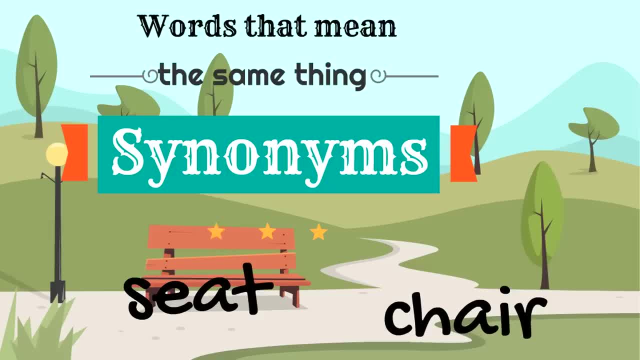 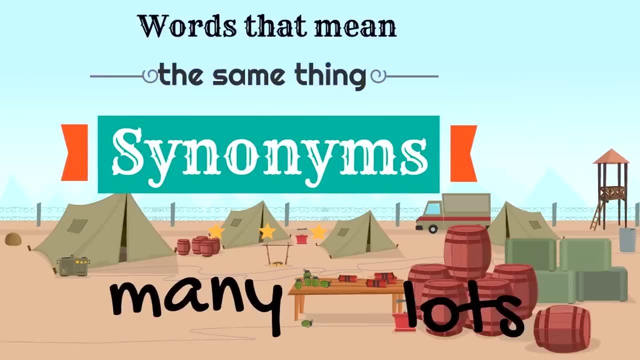 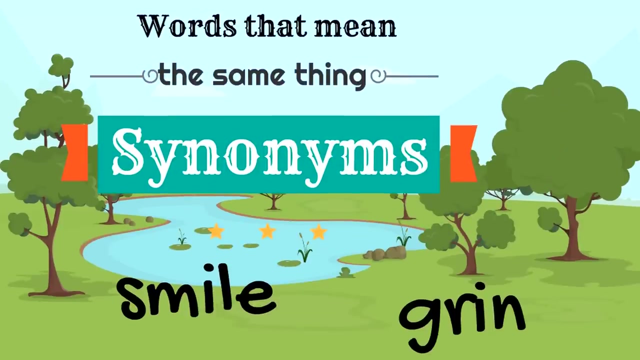 is a seat. Those are synonyms. The words many and lots: they mean the same thing. Words that mean the same thing are synonyms. So many and lots are synonyms. They mean the same thing. Look at these two words, smile and grin. Those words are words that mean. 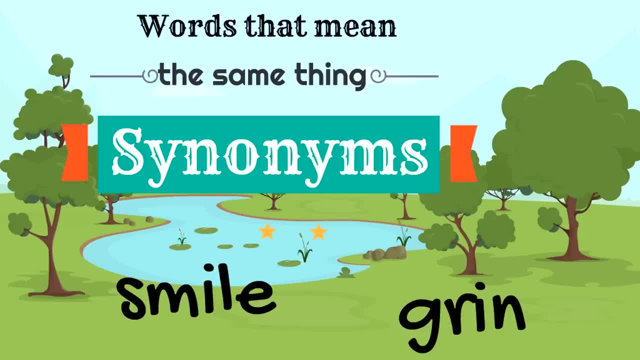 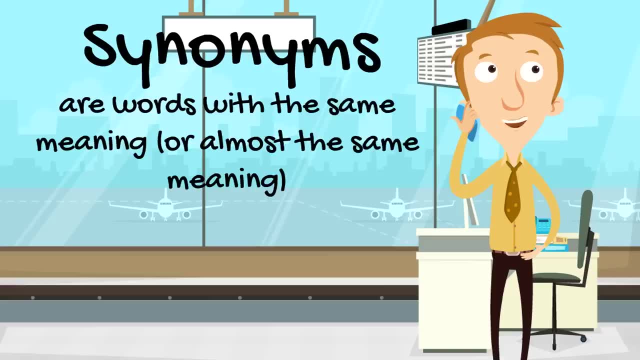 the same thing, They're synonyms. Hopefully, with those examples you're seeing that synonyms are words with the same meaning, But in our definition earlier, synonyms are also words that have almost the same meaning. The words aren't exactly the same in meaning, but they are very, very similar. So we're going to 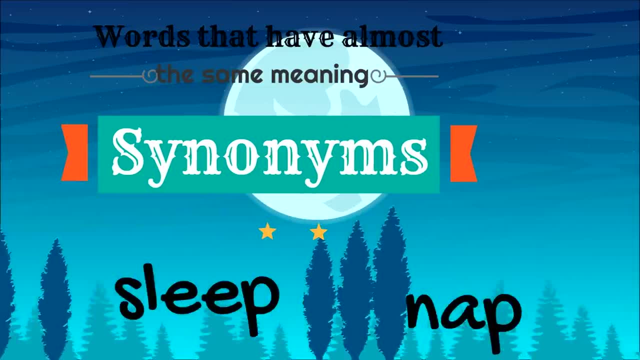 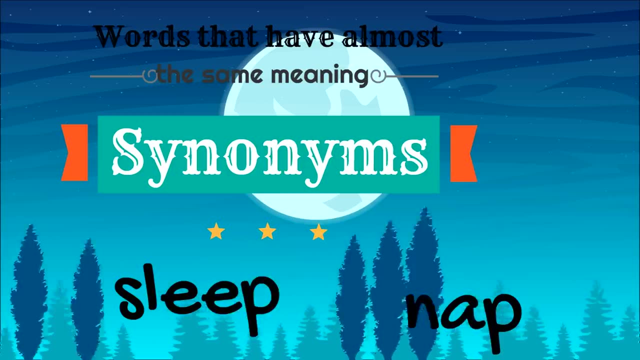 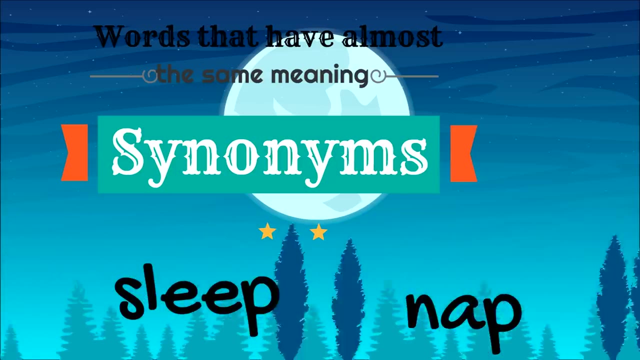 look at some of those synonyms. Sleep and nap are great examples of synonyms that have almost the same meaning. The meaning isn't exactly the same, but it's basically the same, because napping is a type of sleeping, but not all sleep is a. 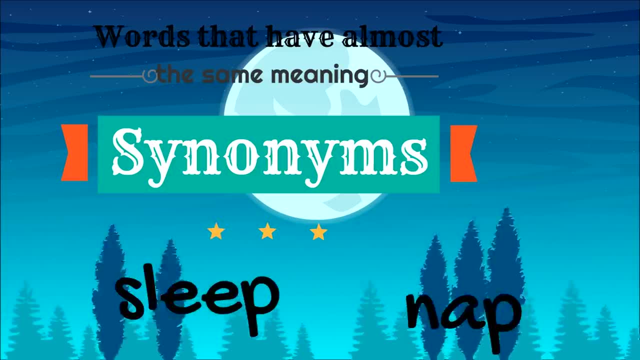 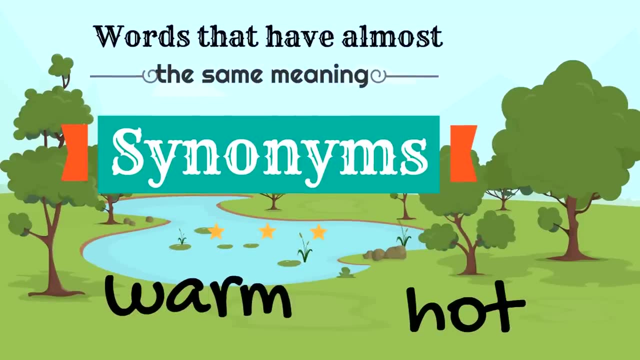 nap, But they're basically the same, So they're still synonyms. Look at these: warm and hot- These are synonyms. Now, hot is harder than warm, So they're not the exact same meaning, but they're very similar meanings, so they 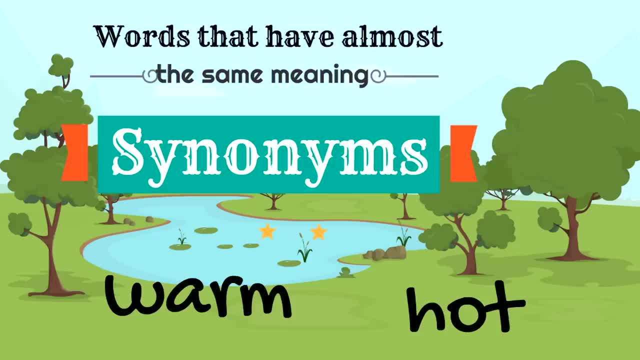 are still synonyms. Shop and store are also synonyms. Now, a store is usually bigger than a shop, but they mean basically the same thing: it's a place you buy things. so they are still synonyms. because they have almost the same meaning, they are still synonyms. well, there you have it. synonyms are words that have the same. 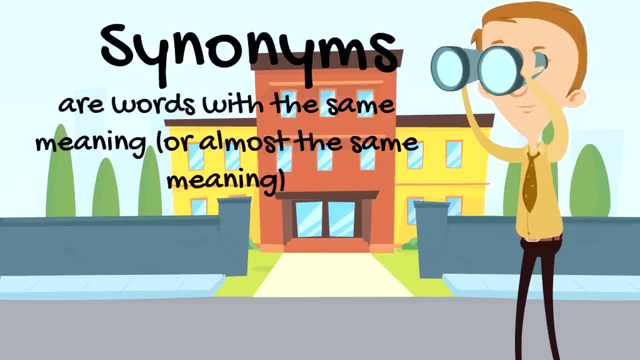 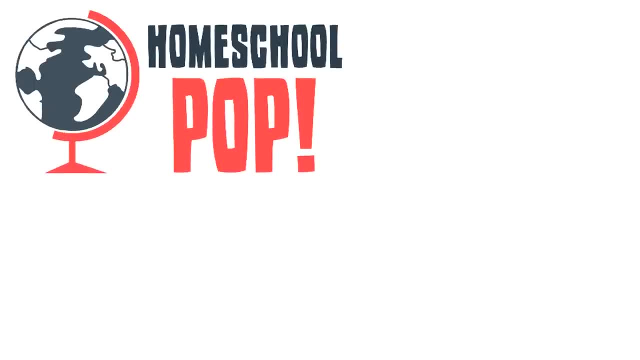 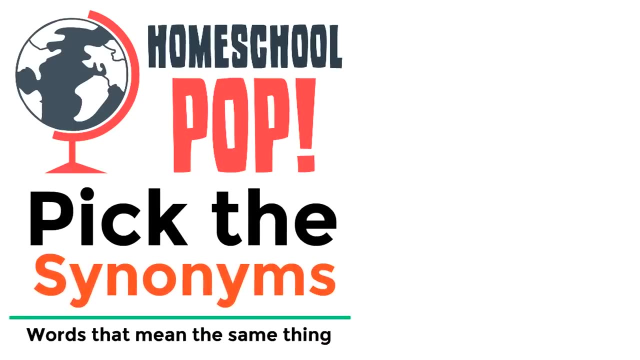 meaning, or almost the same meaning. now we want to find out how much you have learned. we want to play a game that we call pick the synonyms. we're gonna show several words and you pick out which of the words are the synonyms. here we go fast, best quick. which two of these words are the synonyms? yeah, fast and quick. 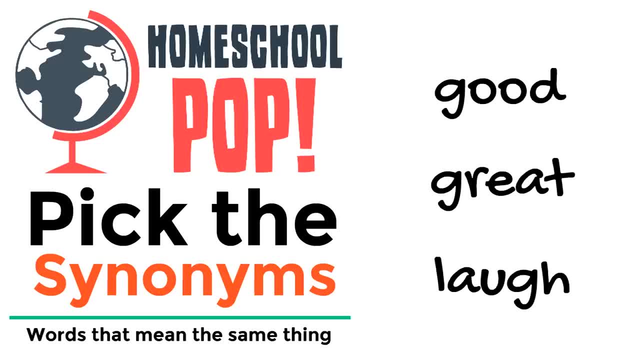 try these good, great laugh. which are the synonyms? yeah, good and great. try this: tug pop, pull. which two are the synonyms? yeah, tug and pull. hey, here we go. road bike, bicycle. which two are the synonyms? yeah, bike and bicycle. great job. last one: beautiful, pretty and glad. which two are synonyms? yeah, beautiful. 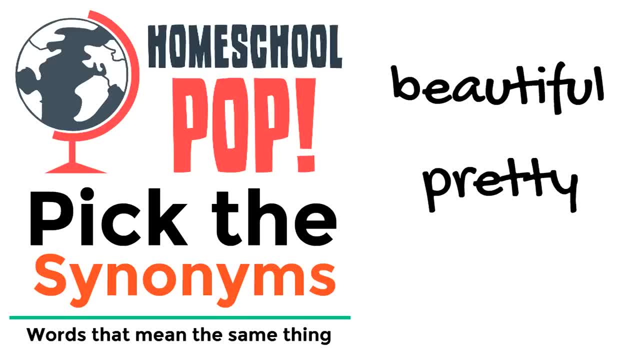 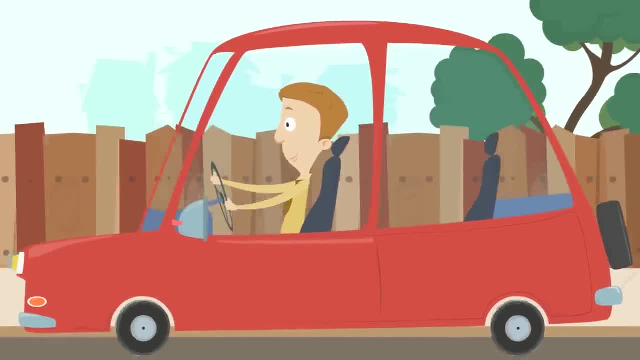 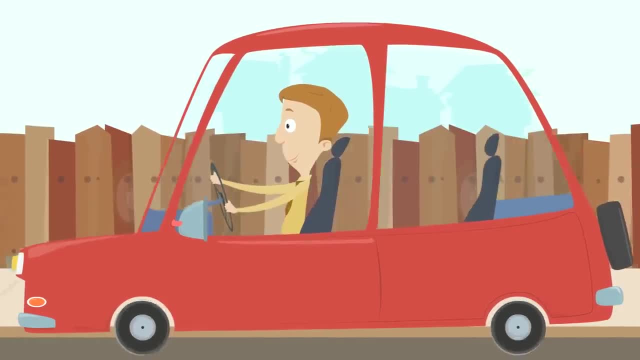 pretty and glad. which two are synonyms? Yeah, beautiful and pretty, Great job. Well, next time you see two words that mean the same thing, you can say you know what Those are synonyms. Thanks for watching. We had so much fun. 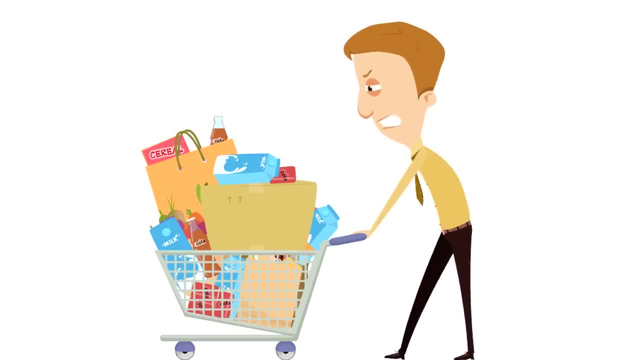 Oh, this is such a heavy cart. Oh, my goodness. Oh, it's hard work. You know, a lot of times learning can be hard work too, But we hope that these videos are really helpful, make learning fun, so that learning isn't hard like pushing this cart. 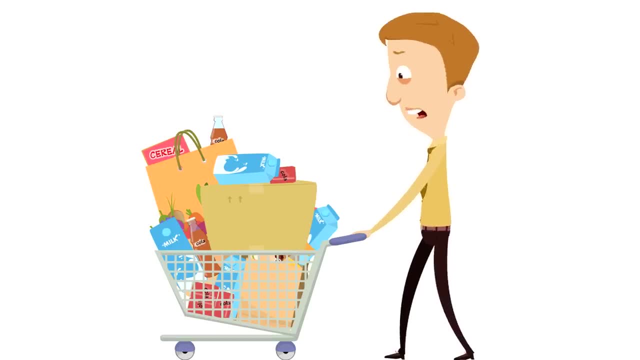 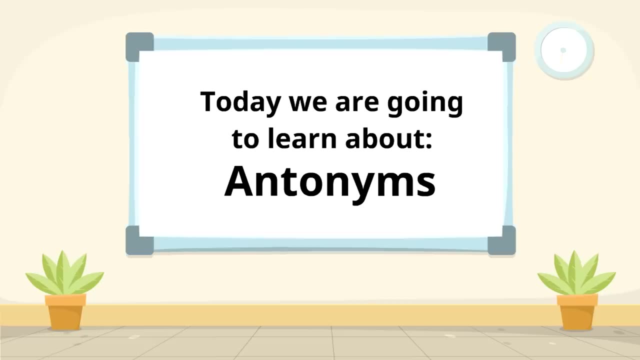 Oh, my goodness. All right, What's the next thing we should learn about? Let's learn about Antonyms: What antonyms are Antonyms, What antonyms are, And how to pick them out. So today we're learning about antonyms. 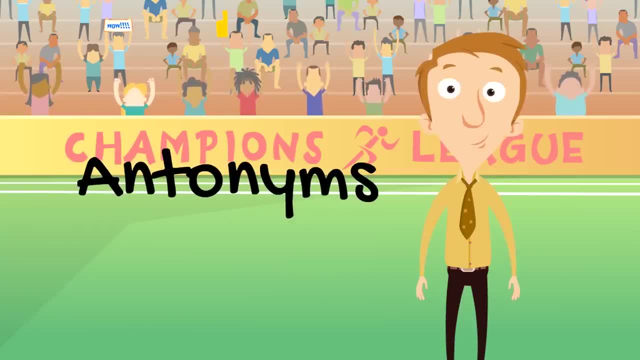 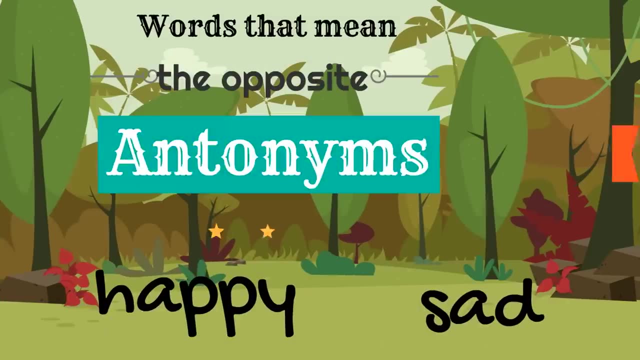 Antonyms are words with the opposite meaning. They're words that mean the opposite thing. Here's an example of antonyms: Happy and sad. These two words mean the opposite thing. That makes these antonyms? Happy and sad mean the opposite things. 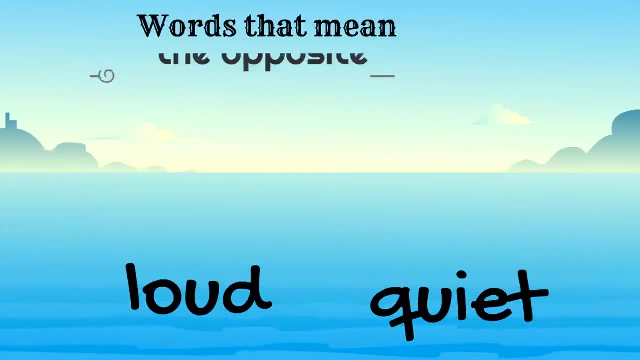 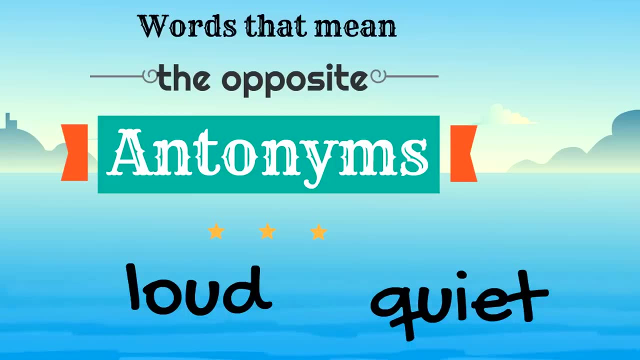 They're antonyms. They're words that mean the opposite. Words that mean the opposite are antonyms, like loud and quiet. Loud is loud, but quiet is like a whisper. Loud and quiet are antonyms. How about these antonyms? Hot and cold? 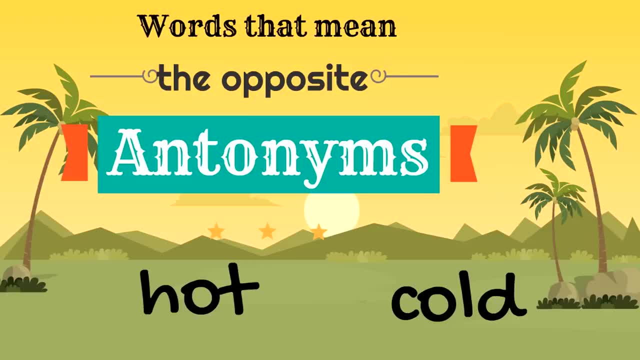 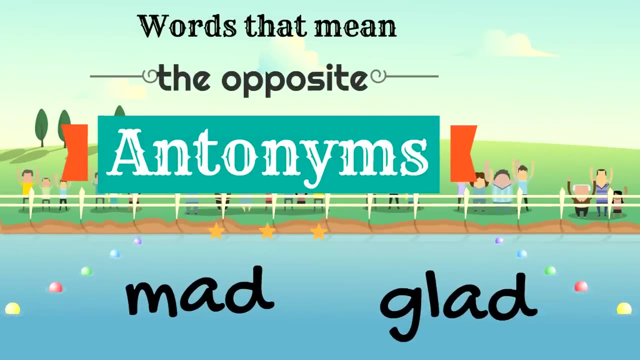 Hot and cold mean the opposite things. That means they're antonyms, They're opposites. Hot and cold, They're words that mean the opposite thing. Antonyms are words that mean the opposite thing, like mad and glad. They're completely different. 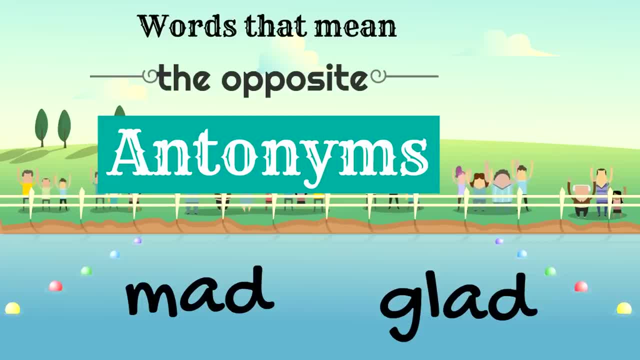 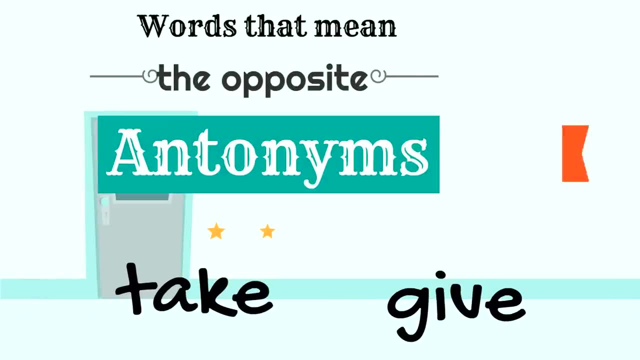 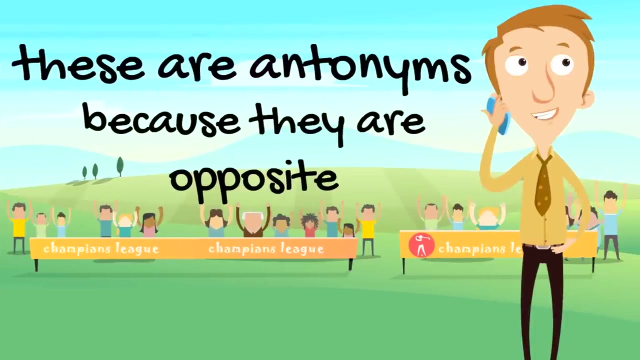 They're opposite. These words are antonyms. Mad and glad are antonyms. What about these antonyms Take and give? Take and give are words that mean the opposite thing. They are antonyms. Take and give are antonyms. Take and give are antonyms. 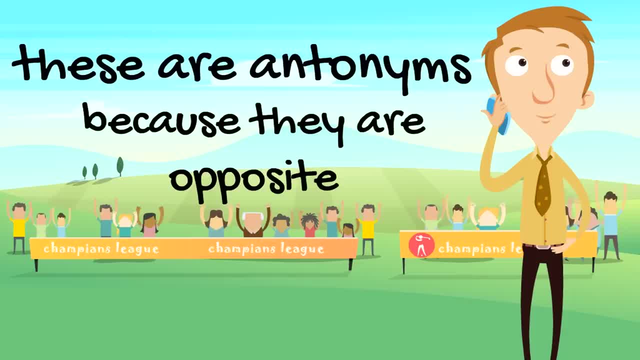 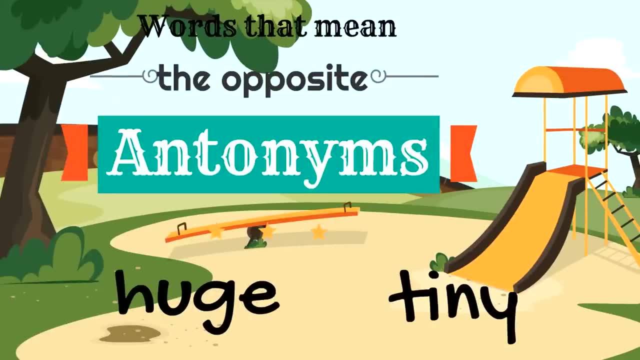 These are antonyms because they are opposite. These are antonyms because they are opposite. Look at these Huge and tiny. Huge is really really big and tiny is really really small. They mean the opposite thing. They are antonyms. 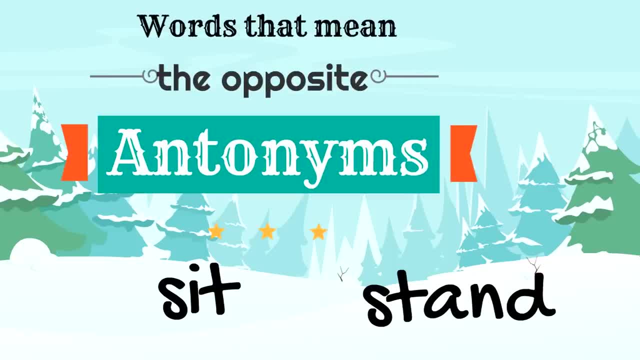 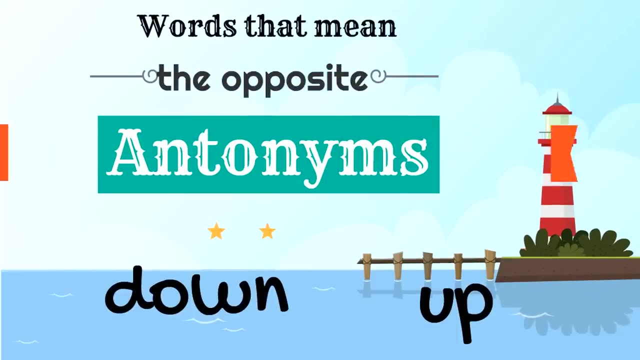 Here are more antonyms. Here are more antonyms Words that mean the opposite thing: Sit and stand. Those are completely different. They're the opposite. Sit and stand are antonyms. Antonyms are words that mean the opposite thing, like down and up. Down and up are yep antonyms. 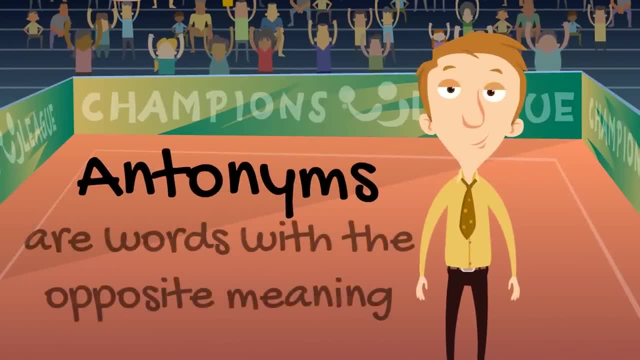 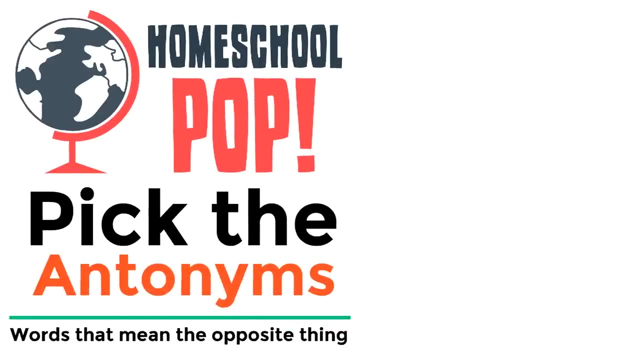 As you're learning, antonyms are words with the opposite meaning, And I think you're understanding this now. so what we're going to be doing is we're going to be doing a fun little game. We're going to play a game called Pick the Antonyms, which means we're going to be picking. 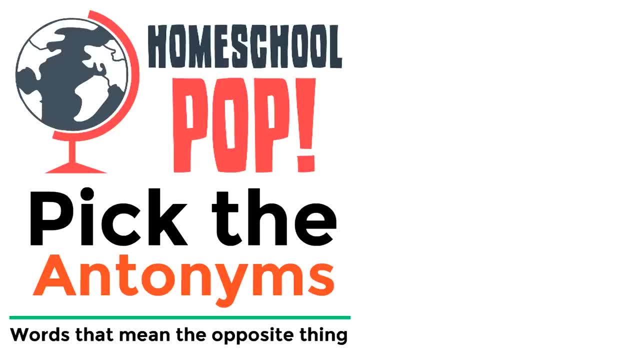 the words that mean the opposite thing. All right, I hope you're ready, I hope you're excited, and let's get started. So here are words. Here are words: Tall, big and short. Two of these words are antonyms. Which ones are? 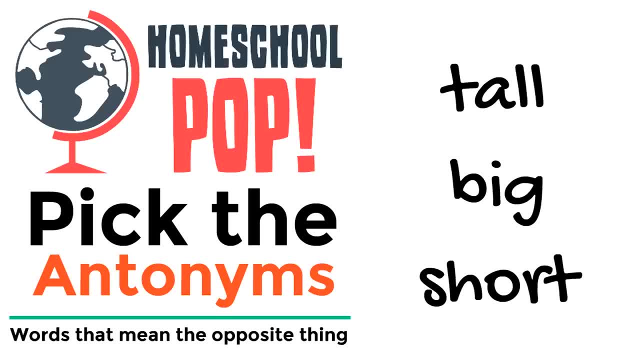 antonyms. I'm going to need your help. Tall, big and short. Which two words are the antonyms? Yeah, tall and short, They mean the opposite things. They're the antonyms. What about these? Sell, buy and show? Which of these words are antonyms? Remember antonyms? 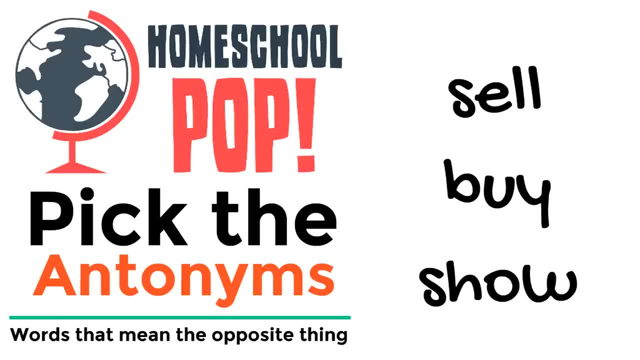 were looking for the opposite. Which two words mean the opposite thing: Sell, buy and show. Yeah, sell and buy are the antonyms. They mean the opposite thing. Here's the next one: Go will won't, Go will, won't. Which two words are the antonyms? 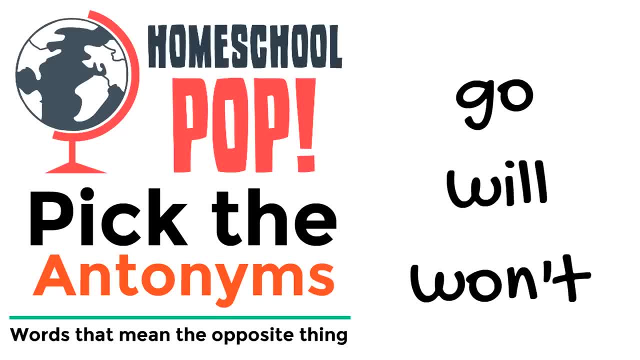 Yeah, will and won't are the antonyms, and we know they're antonyms because, uh-huh, they mean the opposite thing. Here's our last one: Over ground. under Which of these words are antonyms Over ground? 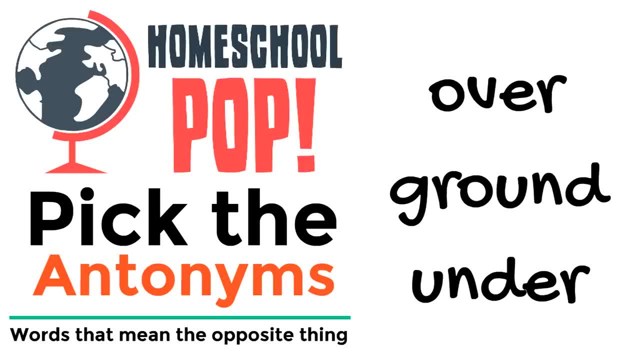 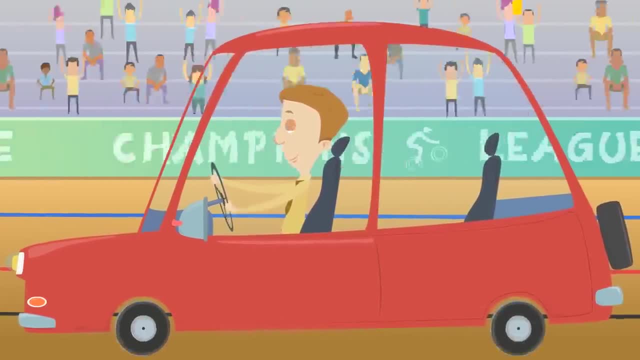 under Uh-huh. yes, Over and under are the antonyms. They mean the opposite thing. Awesome job. Well, we're going to speed along. but next time you see words that mean the opposite things, you can say to yourself: hey, those are antonyms. 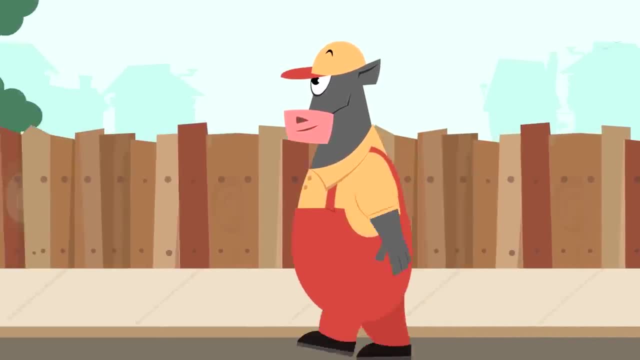 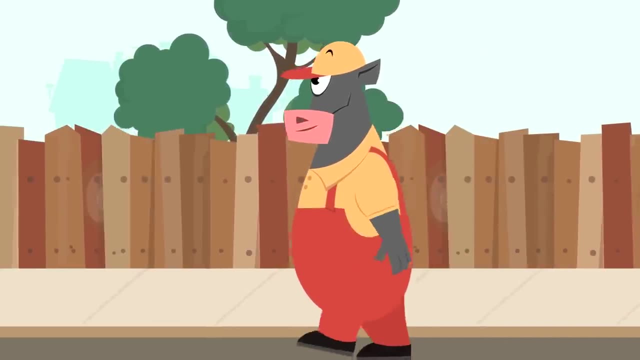 Oh, wow, look, it's the homophone cow. Homophone cow Ho- homophone cow. You- you just walking, you're just- you're just going to ignore me. I- I see how it is Okay, so you're upset that we haven't included you in other videos. What do you call this? 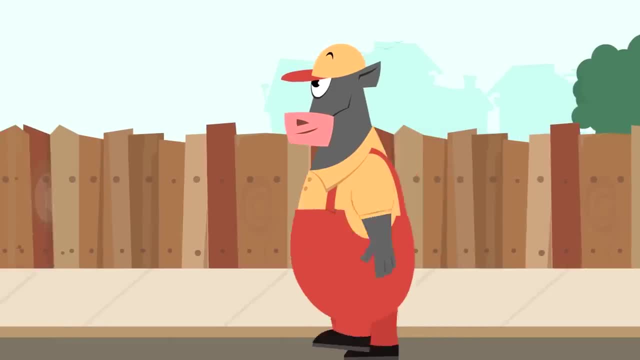 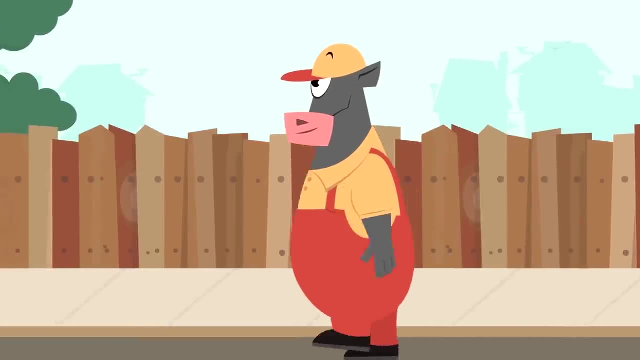 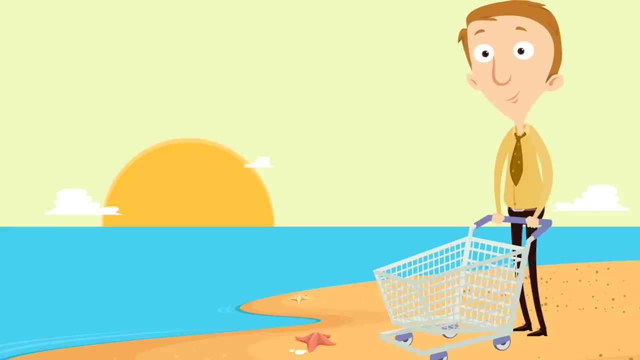 you know you're in a compilation video. that's cool too. all right, I need to talk to the homophone cow, but in the meantime, let's learn about sentence fragments. the beach is so wonderful, isn't it? don't you just love the beach? I'm standing here. 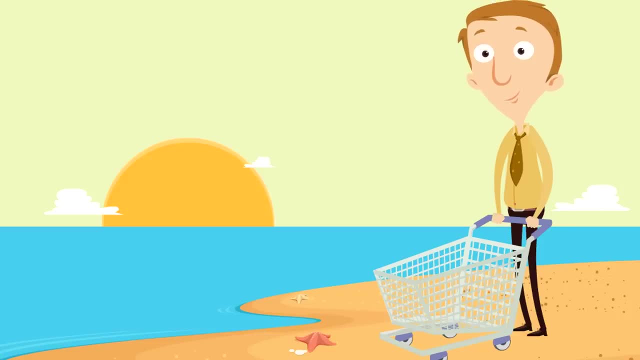 with my shopping cart and there's one word that comes to mind when I'm standing here looking at the sun setting: this is complete. what else could you want? you're standing on a beach. don't make fun of the shopping cart and I might find something on the beach. okay, you don't bring a shopping cart to the 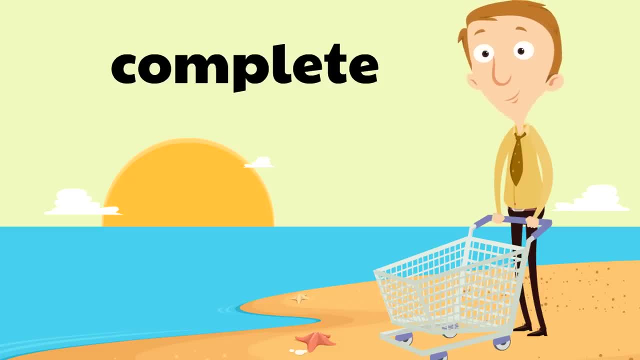 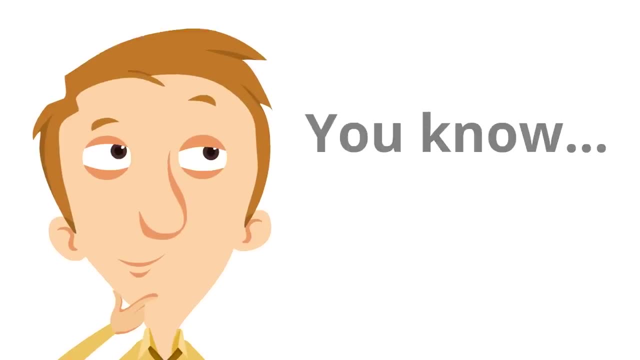 beach. that's weird. okay, I've got a shopping cart. I feel complete. this is complete to me. this makes me feel happy. you know sentences can be like that too. you see sentences like to be complete. you know sentences can be like that too. you see sentences like to be complete. 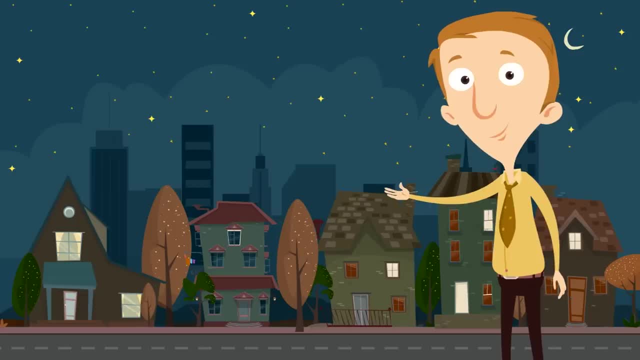 they love to be complete. a sentence always has a subject and a verb. a sentence wants to be complete because without a subject and a verb, it's not a sentence anymore. in fact, it's something else. it's a sentence fragment. but let me not get too far ahead of myself. always remember a. 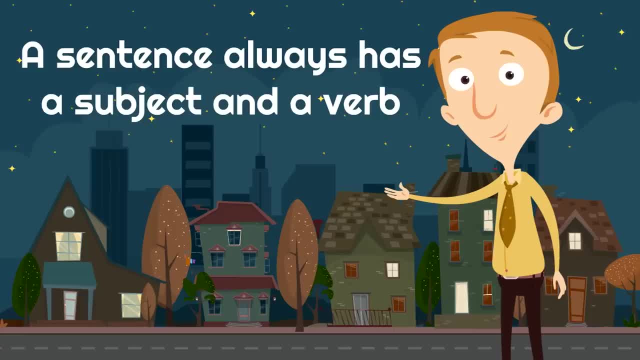 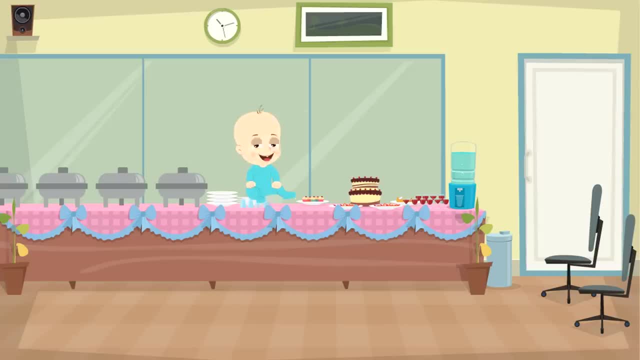 sentence has to have a subject and a verb, kind of like every cool birthday party has to have a baby and Chomsky, I mean, I mean the baby, maybe Chomsky, I haven't forgotten about the hat. I haven't forgotten about the hat. yeah, So you can come to my party, but 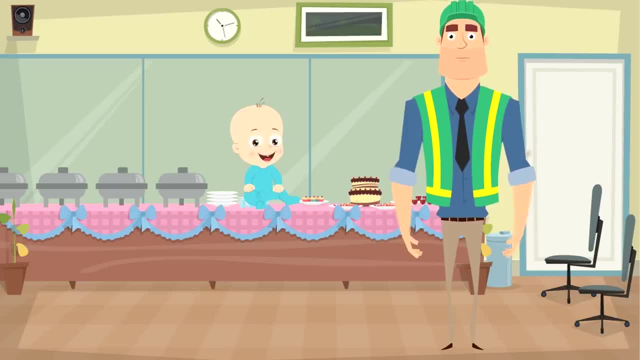 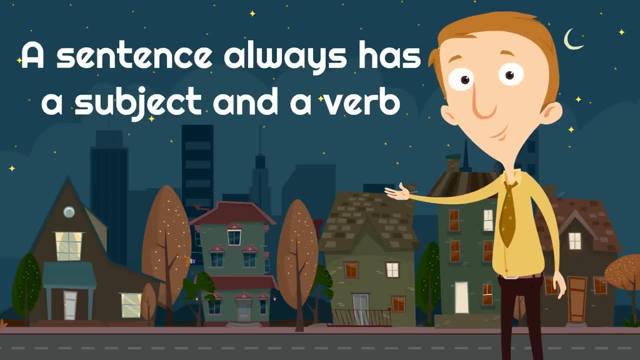 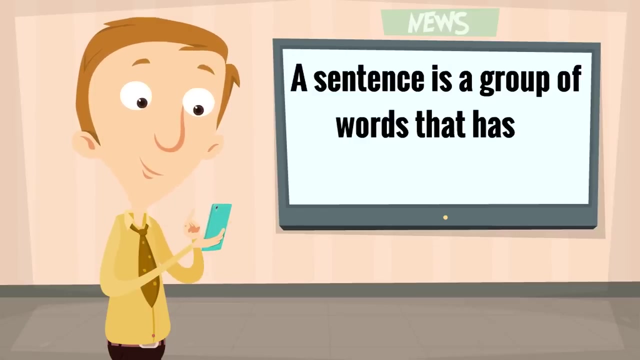 it's still. it's still raw, It still still hurts, Still hurts. Alright, let's get back again. So a sentence always has a subject and a verb. That means a sentence is a group of words that has a subject and a verb. It 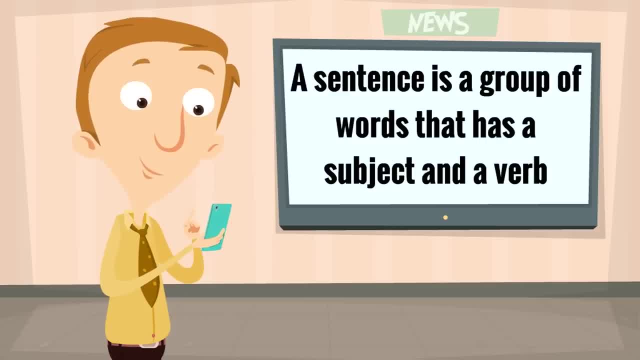 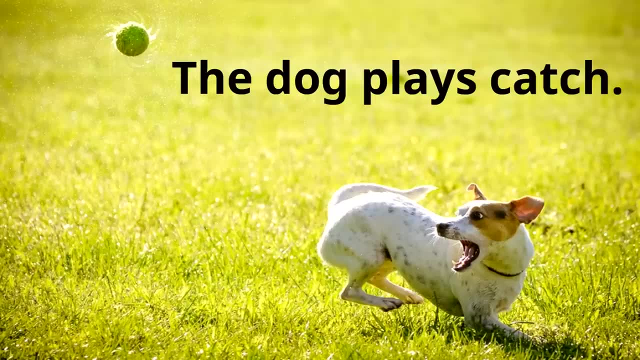 needs to have both, otherwise it's not a sentence. A sentence is a group of words that has a subject and a verb, like this: The dog plays catch. Does it have a subject and a verb? Yeah, The subject is the word dog and the verb. 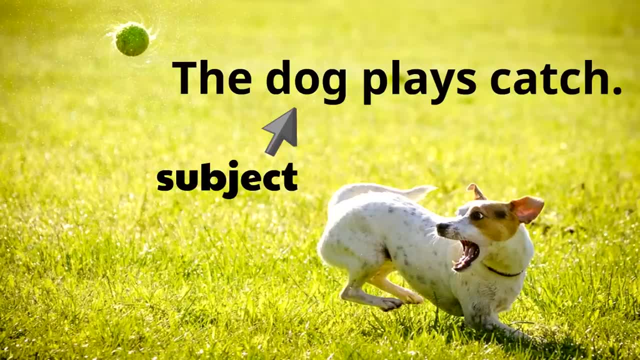 which word? which word is the verb? yeah, plays. this is a sentence. it has a subject in a verb, which means it's expressing a complete thought. this is complete. there's a subject, there's a verb. we know what's going on and there's no way this dog is catching this ball. or maybe this dog will catch the ball? who? 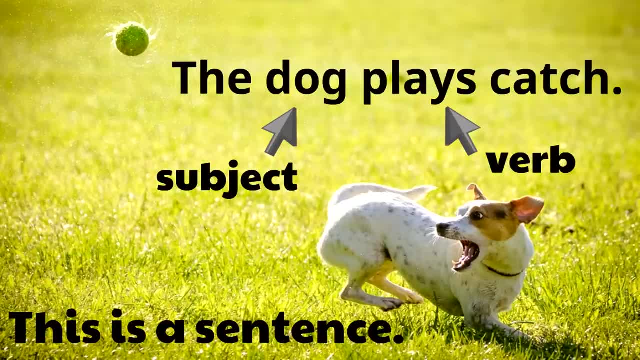 knows. let us know in the comments which one you think will happen. you think he's gonna catch it or do you think it's gonna fall to the ground? who knows? but this is a sentence. this is complete. it has a subject and a verb. it's a sentence. 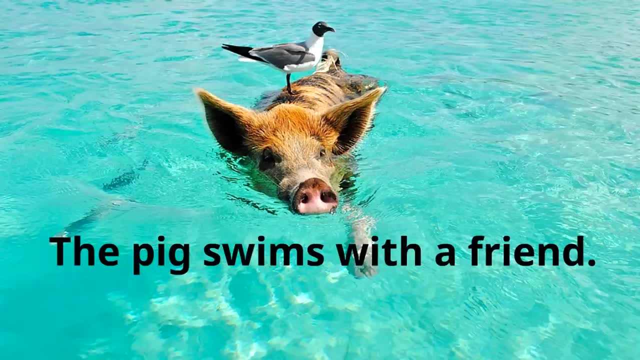 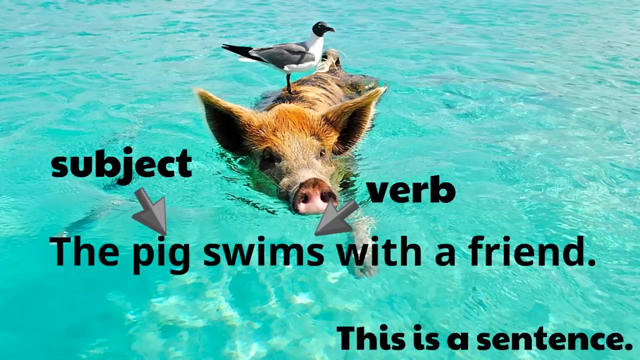 or look at this one: the pig swims with a friend. the pig swims with a friend. is there a subject and is there a verb as well? well, yeah, the subject is pig, the pig, but is there a verb? which word is the verb? yeah, swims, so this has a subject and a verb. this is a sentence, I mean it's got a subject. 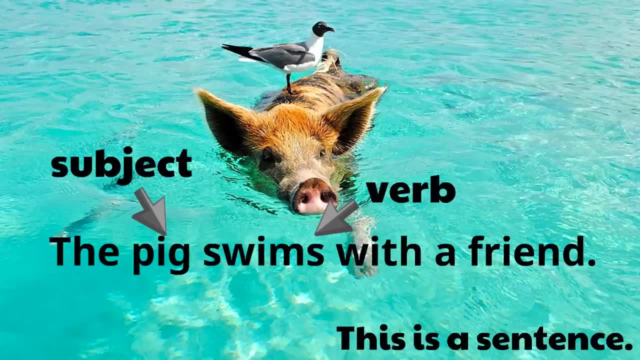 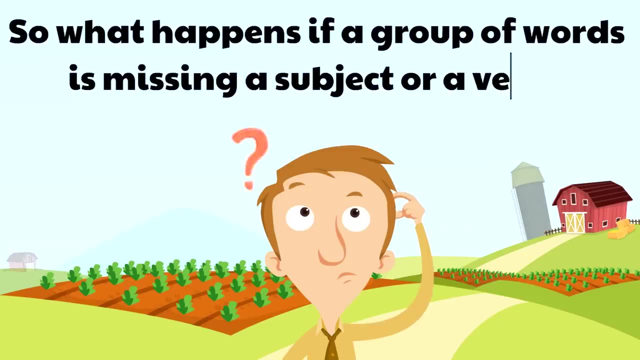 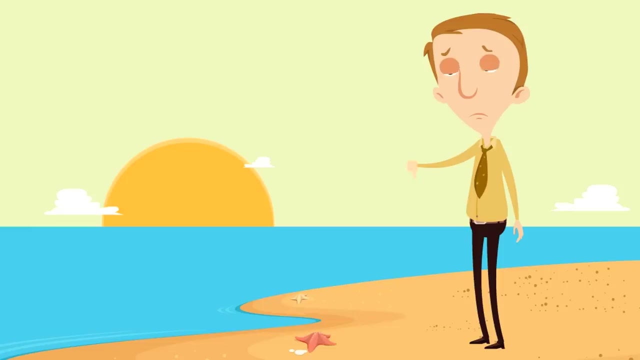 and it's got a verb and it's expressing a complete thought. it's not missing anything, it's complete, it's got the subject, it's got the verb, it is a sentence. so what happens if a group of words is missing a subject or a verb? well then, it's kind of like me on the beach without my shopping cart. you 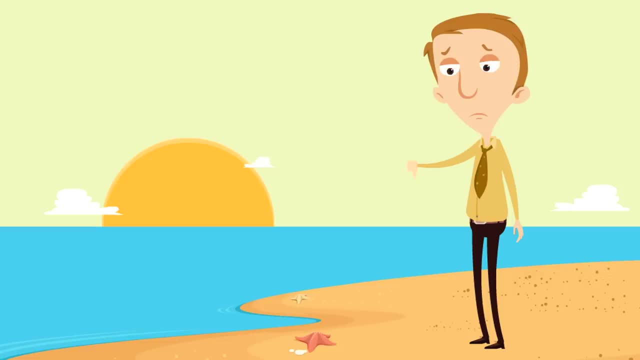 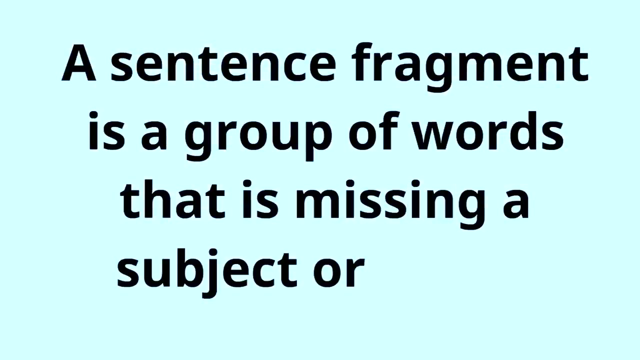 know it's missing something. a sentence fragment is a group of words that is missing a subject or a verb. that's what it's called. is a sentence fragment? when it's missing a sentence that is missing a subject or a verb. that's what it's something. when it's just part of a sentence, it's missing something, it's not. 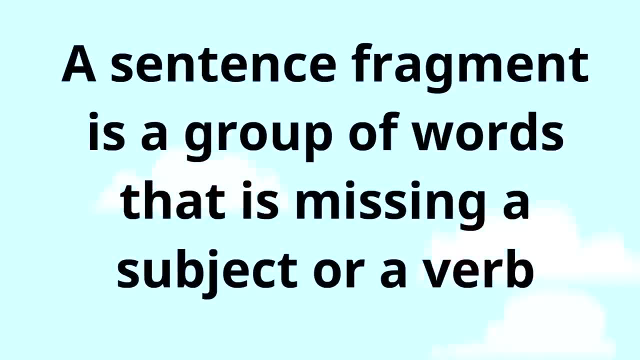 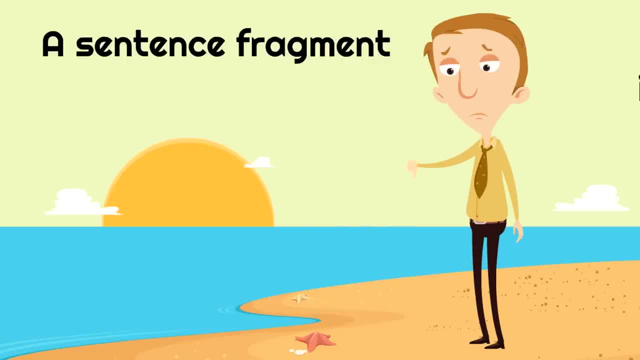 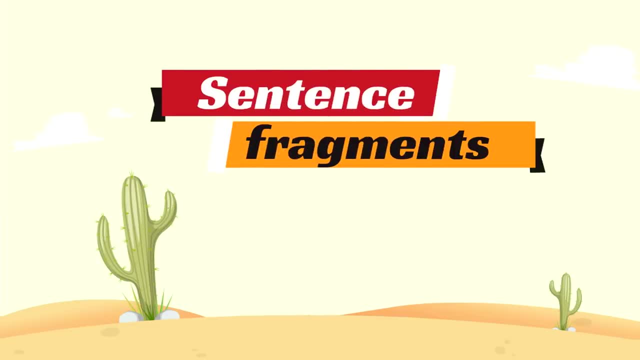 a complete sentence. it's a sentence fragment, kind of like being on the beach without my cards. a sentence fragment is incomplete, it's missing something. we're going to show you some sentence fragments so you can see that they're incomplete. they're missing something. they're missing either a subject or a. 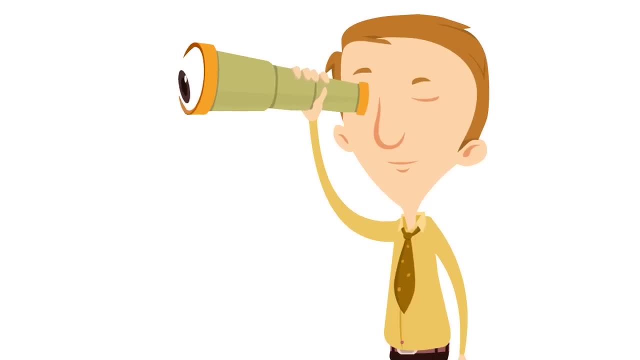 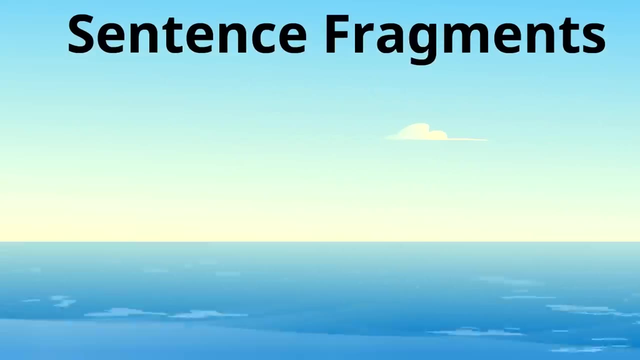 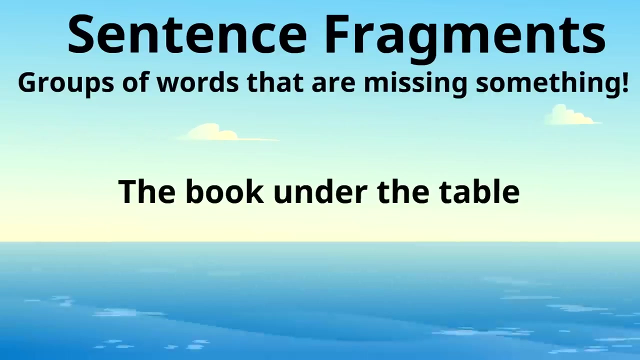 verb. all right, I'm ready to look at them. sentence fragments are groups of words that are missing something like this: the book under the table. what? the book under the table? where's the verb? there's no verb. it has a subject- the book- but there's no verb. it doesn't tell us. 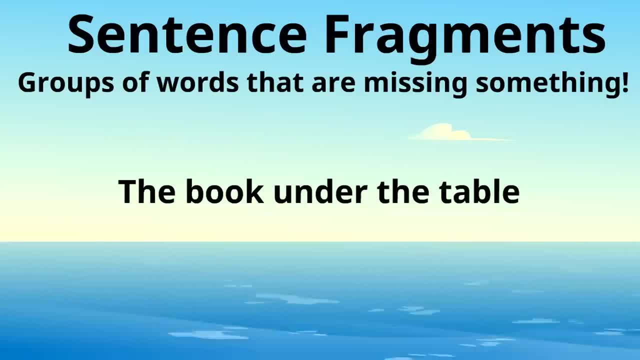 what's going on with the book? what about the book under the table? there's so many unanswered questions. this is not a complete thought. the book under the table is a sentence fragment, or how about this? one ran to school, ran to school. it doesn't have a subject. who? 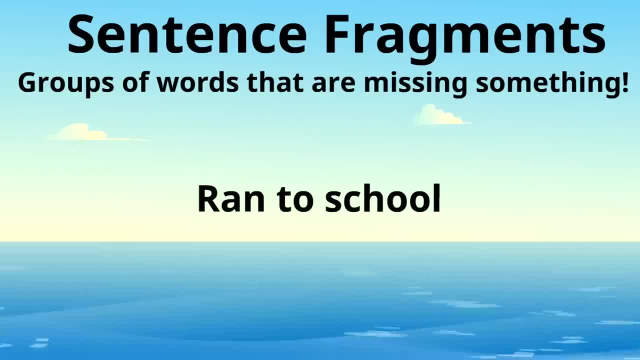 ran to school. we have so many questions about this. this is not a complete thought. it doesn't tell us who it's talking about. every sentence has to have a subject and a verb. this has the verb ran, but it doesn't have a subject. ran to school is not a complete sentence. it's a 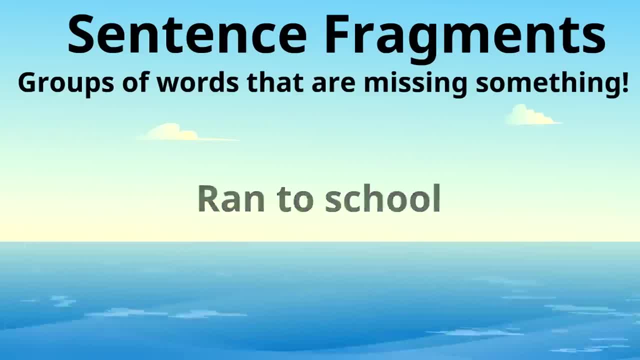 sentence fragment. look at this one: the old car on the road. wait a second. this doesn't have a verb: the old car on the road. it's missing something, isn't? it's a sentence fragment. it's not telling us what the old car on the road is doing. 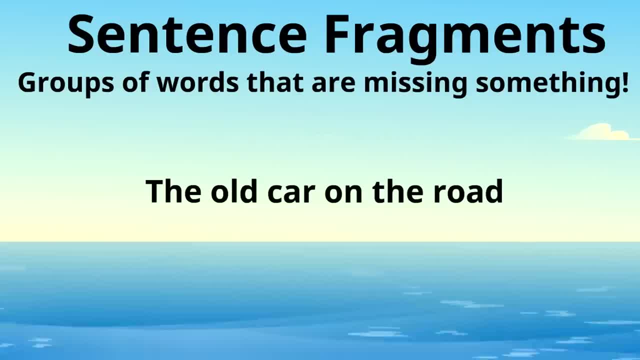 it's just saying the old car on the road. well, what about it? what about it? what's the old car on the road doing? this is a sentence fragment. it's a group of words that's missing something, and our final sentence fragment is: mr whiskers on. 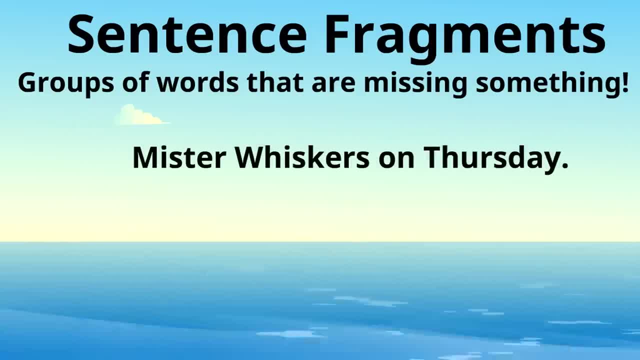 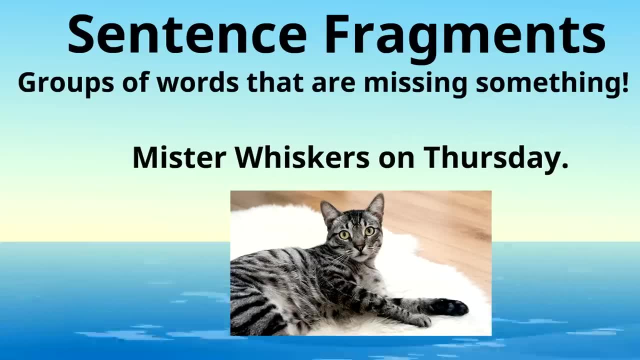 thirst. a wait, a second. what, mr whiskers? what did you do on Thursday? it's a sentence fragment. I don't know, I don't. what did you do, mr whiskers? you don't speak English to you. I have no idea what you did on. 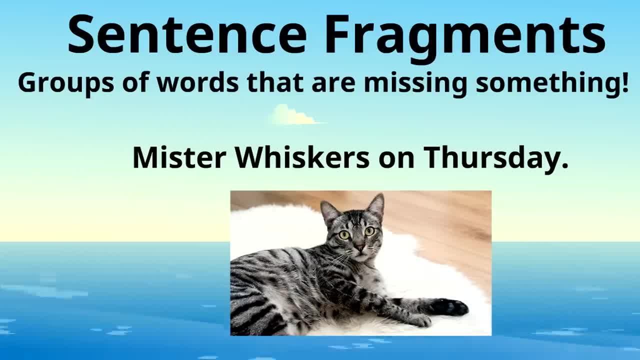 Thursday. I hate sentence fragments because they don't give you all the information. there's no verb. I don't know what mr whiskers did on Thursday. it's not a complete sentence. you gotta have a subject and a verb. mr whiskers, please. I hope you're safe. you know I I go to the beach with my shopping cart on. 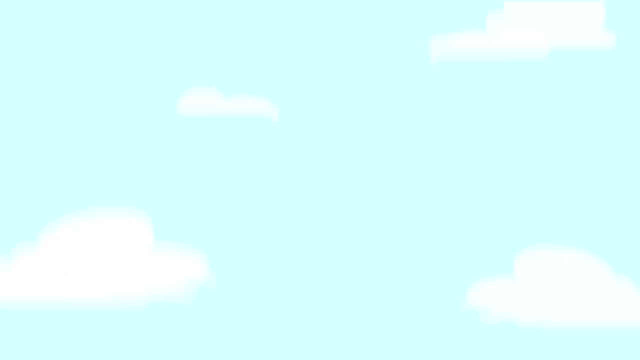 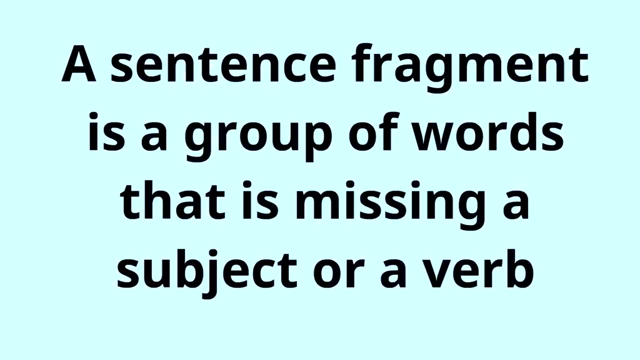 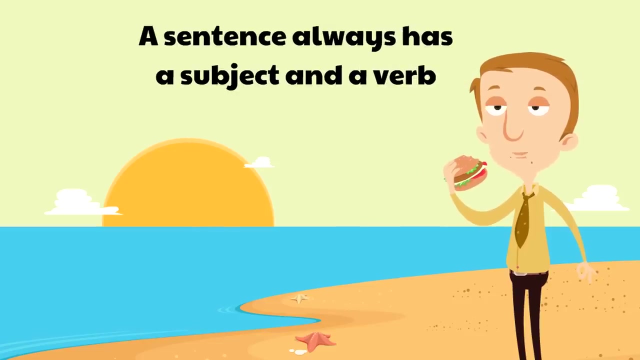 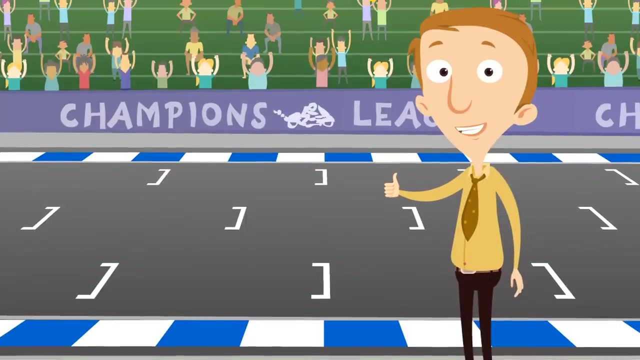 Thursdays and everything to review. a sentence fragment is a group of words that is missing a subject or a verb. now, a sentence always has a subject and a verb. a sentence fragment, though, is missing either a subject or a verb. a sentence fragment is missing something. wow, we are super proud of you. now you know what a sentence fragment is, you. 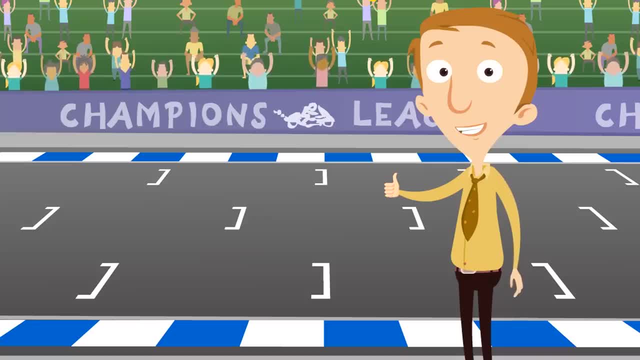 know that a sentence fragment is a group of words that is missing a subject or a verb, and you know that a sentence has both a subject and a verb. a sentence shares a complete thought, but a sentence fragment is missing something. pretty cool, huh. so the next time somebody says something to you that isn't a complete 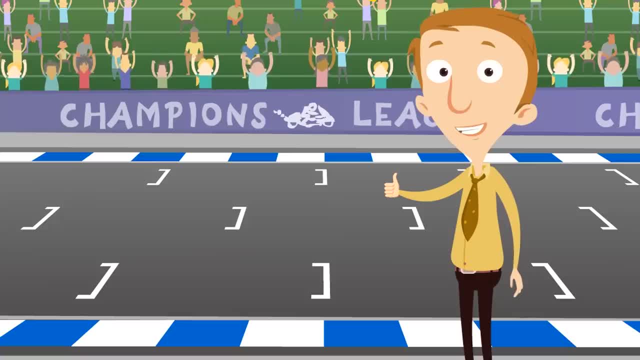 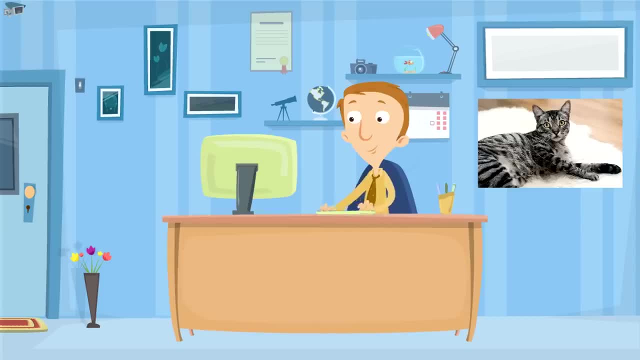 thought you could say: hey, that was a sentence fragment because, uh, that was missing something. we are so happy to have you with us. I mean, you are so awesome, you really are. oh, you like my poster, Mr Whiskers poster. you know, it's pretty cool, pretty cool, you know. oh, it's a pretty cool poster, pretty cool cat too. I. 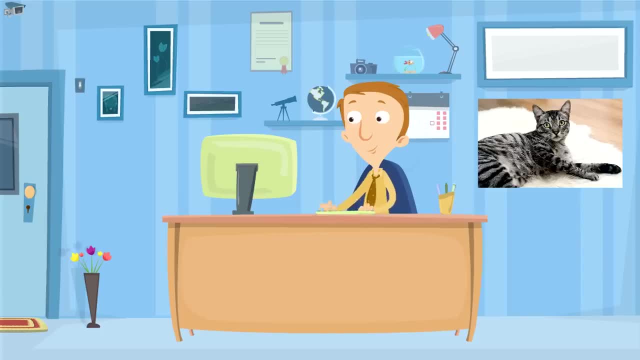 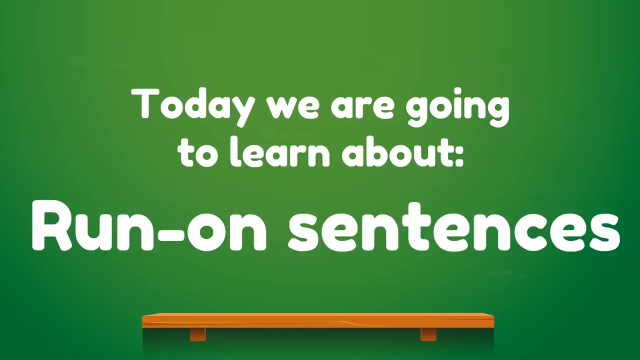 wonder what he would like to learn about next if he would learn from one of our videos. what would he like to learn next? hmm, how about? hmm, let's learn about run on, run on sentences. run on sentences are very interesting. there's something special we have to do to fix them. 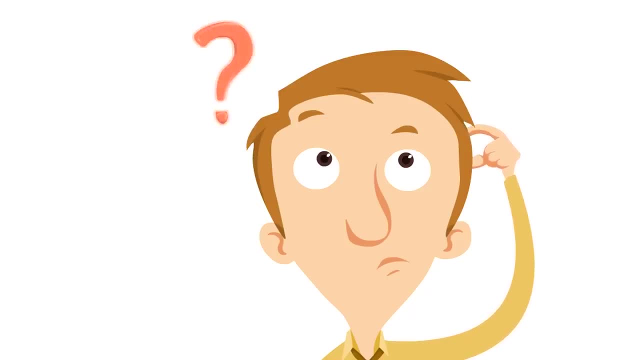 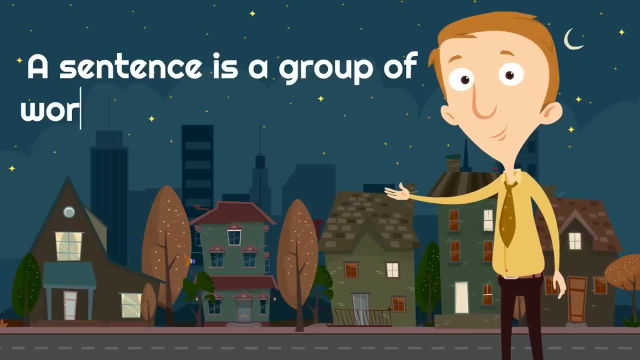 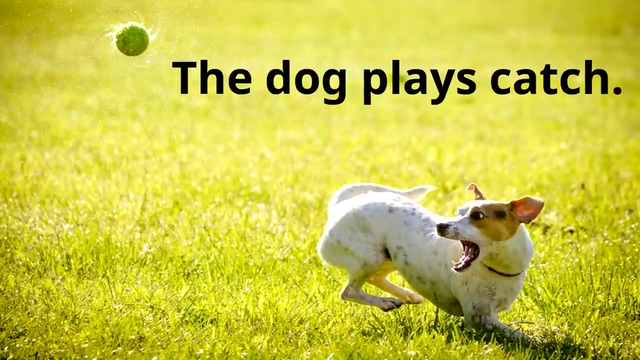 but first, what is a sentence? do you know what a sentence is? well, a sentence is a group of words that has a subject and a verb. so if you see a group of words that has a subject and a verb, you could say, hey, that is a sentence like: look at this, the dog plays catch. this is 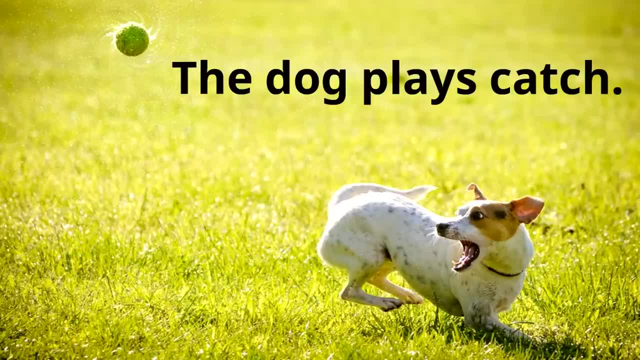 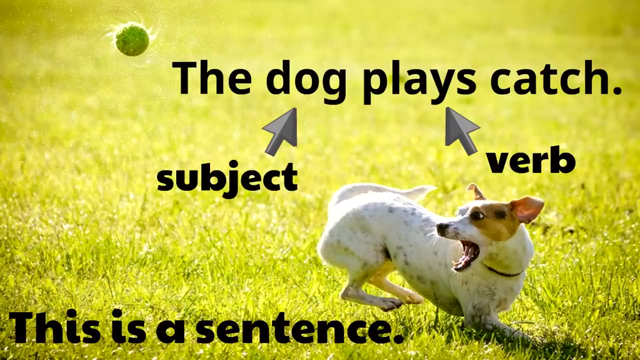 a group of words, isn't it? now, this group of words? does it have a subject and a verb? yeah, it does. the dog- dog is the subject, and what word is the verb? plays. yeah, this is a sentence, isn't it? it's got a subject, it's got a verb. it's a.